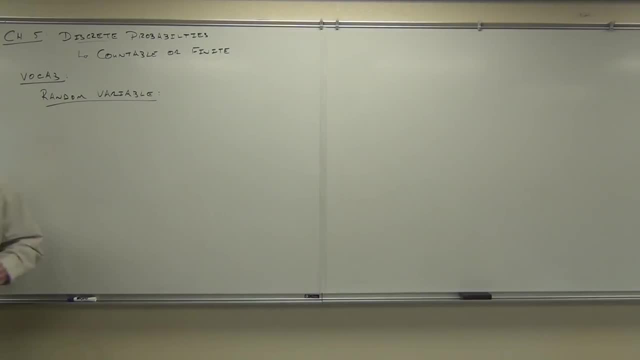 All of our outcomes based on chance, Or in other words, a variable that has a value for each outcome, and those outcomes are determined by chance. And we also use the letter X for our variable- Sorry, that has a value: Variable X. it has a value for each outcome of a procedure. 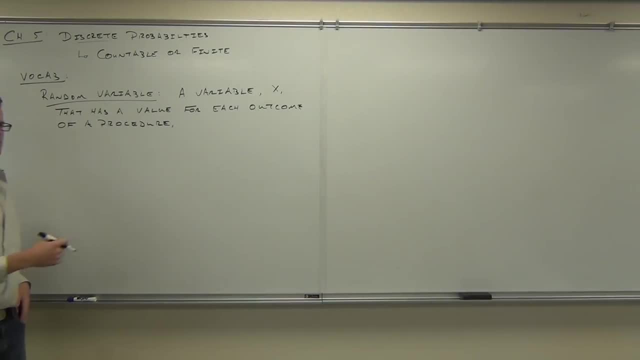 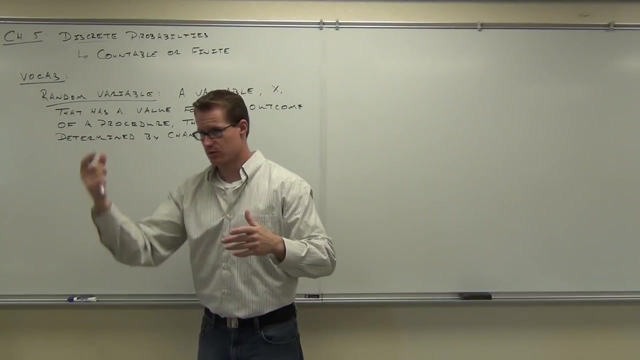 That is a variable that can change at any time. aguary variable that is determined by chance. So random variable. random means by chance, Variable means the outcomes that are changeable, such as rolling a die. we would have a certain number of outcomes. 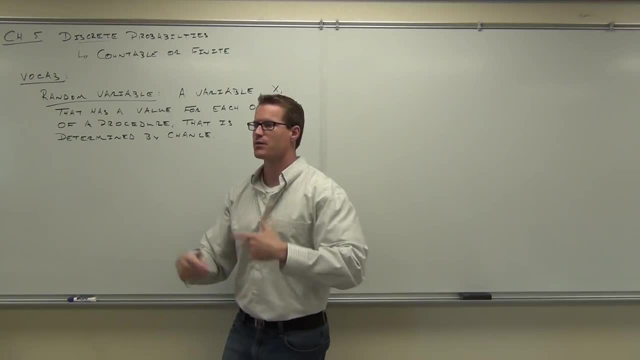 The variable would take the place of those outcomes and the outcome that you get is dependent on the chance of you rolling that die. So the probability of rolling a three or a four or five or six or one or two. So that's a random variable. 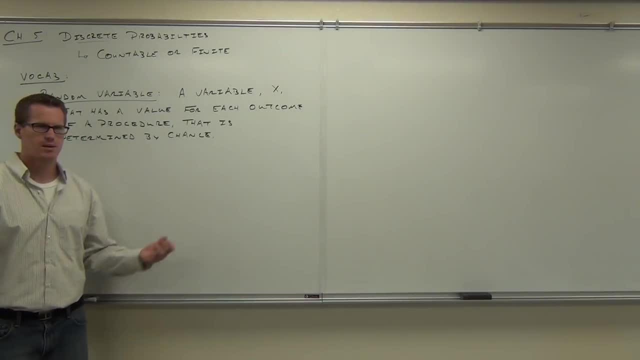 I want you guys to understand the idea of a random variable, And we'll talk more about some examples of random variables in just a little while The other thing we gotta talk about is what's called a probability distribution, Not distribution distribution. Well, we've seen frequency distributions, haven't we? 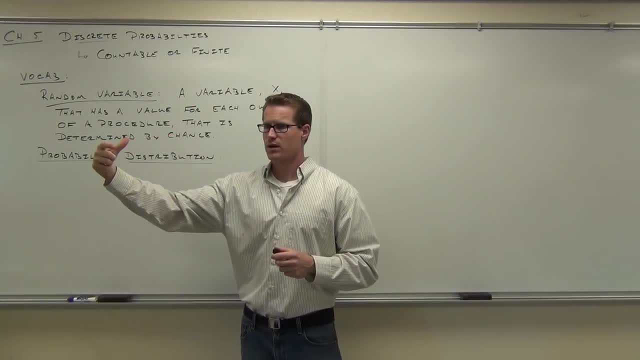 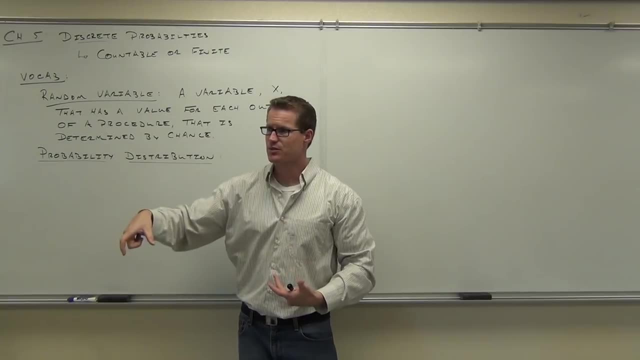 Frequency just took a certain number of classes right, Said what amount we had for each class and put it in a table. That's exactly what a probability distribution does, except instead of classes we have the possible outcomes, or in other words, the values of my random variable. 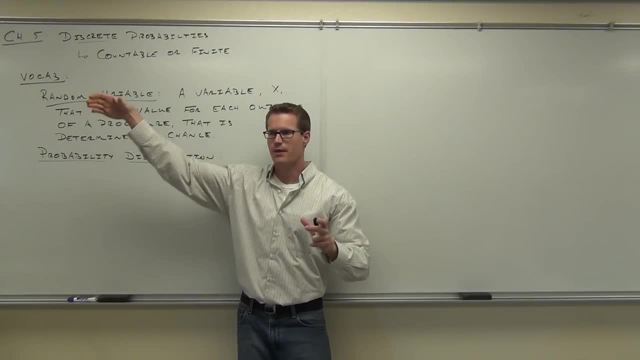 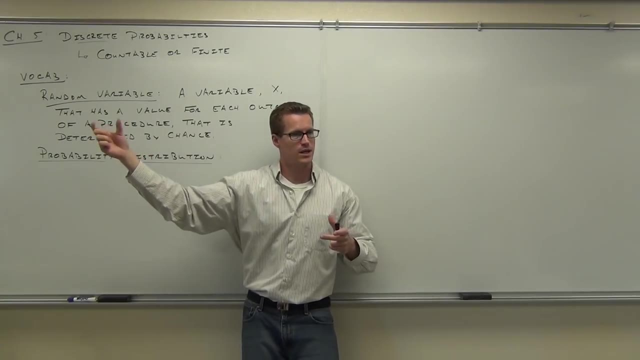 So a probability distribution is based on the outcomes or the values that my random variable can take and the probabilities for each of those outcomes or each of those values that my random variable can take. So it looks just like a frequency distribution, Just like it. 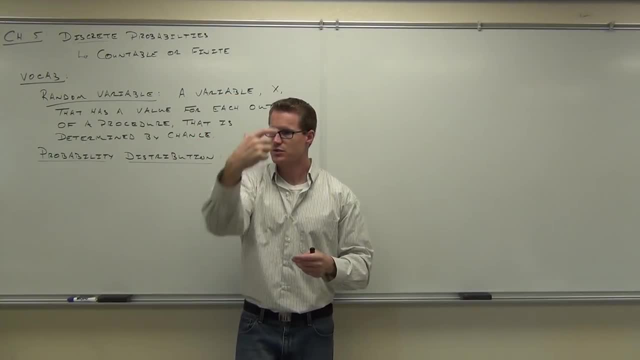 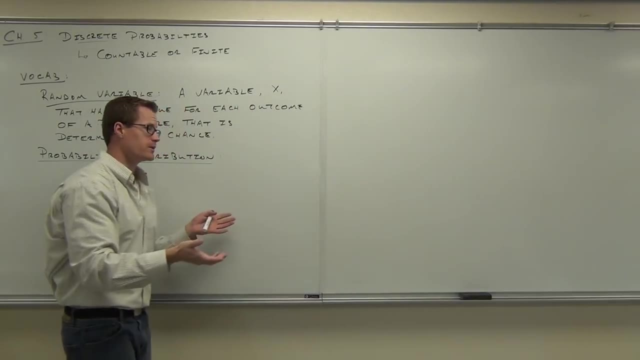 We're gonna have a table like a T chart. We're gonna have some, some columns. on the left-hand side we'll have values, our random variable values. on the right-hand side, we'll have the probabilities and that's a probability distribution. 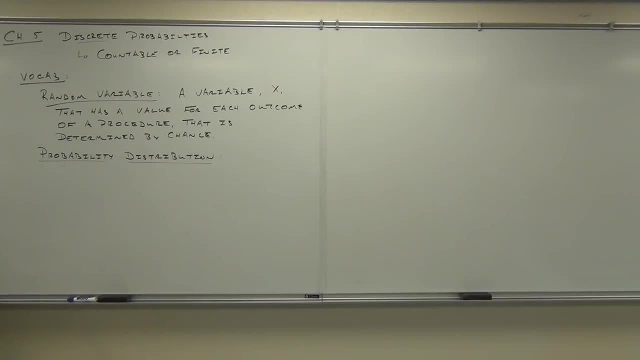 just puts it in a table for us. So probability distribution. what this does, it's a table that gives us the probability for each value of a random variable, A table that gives the probability for each value of a random variable. Let's look at one and kind of flesh all these ideas out. 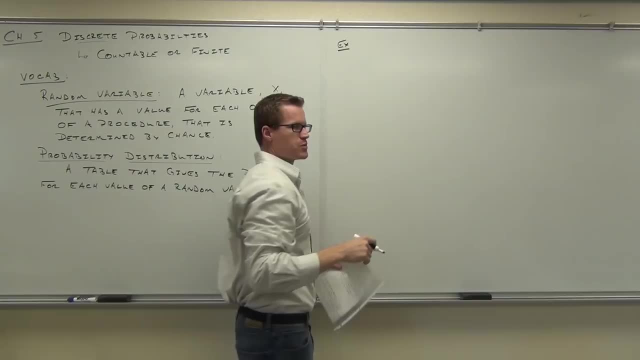 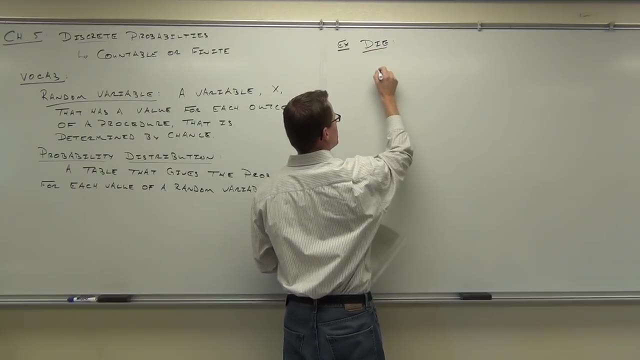 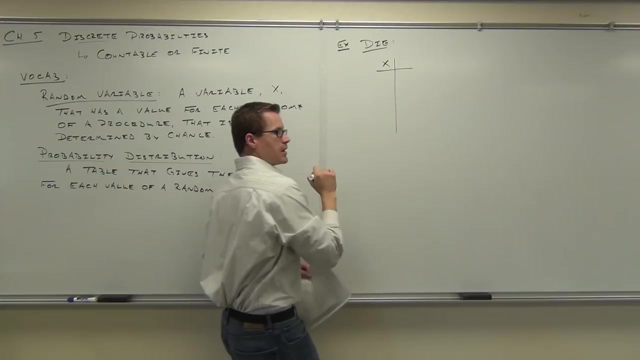 Let's go ahead and do our probability distribution for rolling a die. We've been talking about that already today. Let's actually do it. So here's a probability distribution for rolling a die. Probability distribution is set up like this: You have your x's. 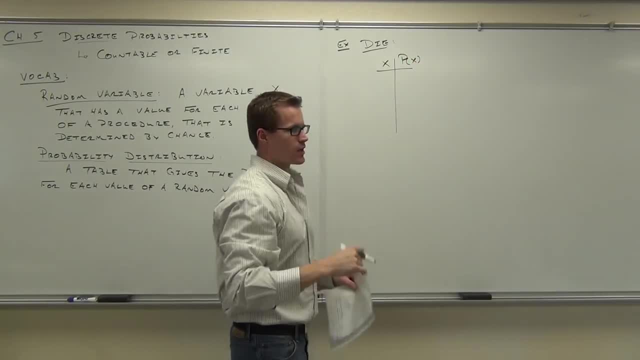 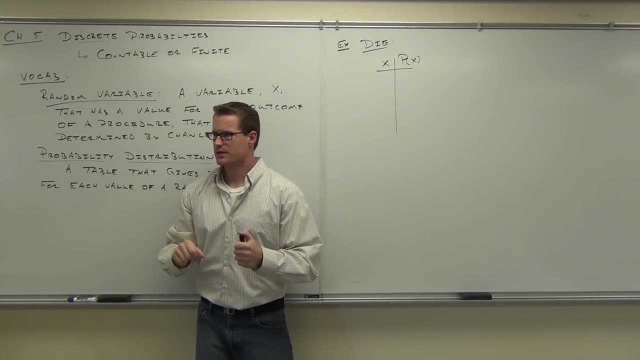 and you have your, your probability of achieving that outcome or probability of getting that value of x In our case. can you tell me what are my x's if I'm rolling a single die? What are my x's? One through six and one through six? 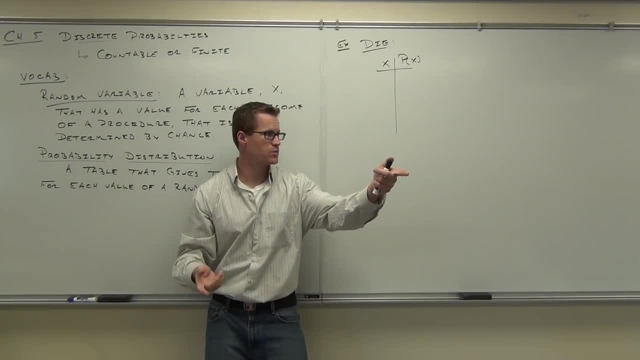 What was that? One through six? One through six, sure, And I heard one through six over here as well. Well, that makes sense, doesn't it? The random variable there is x, and x just has to take on every value. 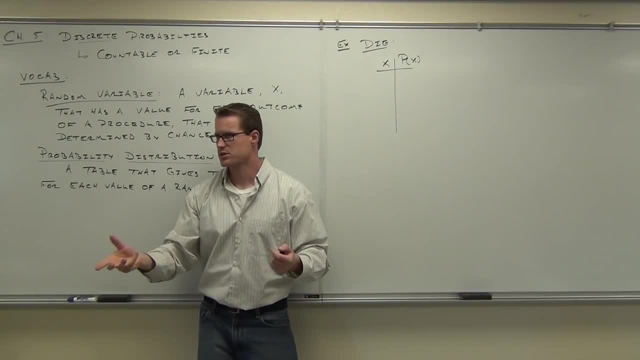 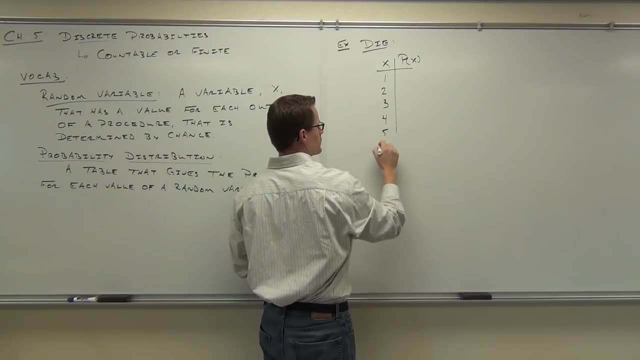 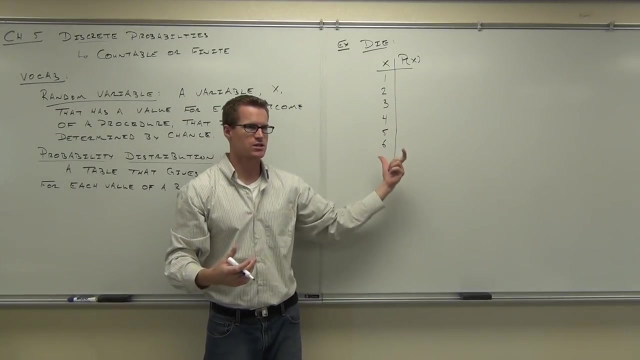 that we can get out of rolling a die. If our die is our standard one through six die, then those values- well, we have one through six. Those are my values of x. My random variable can take on just this many, just six, if I have a standard die. 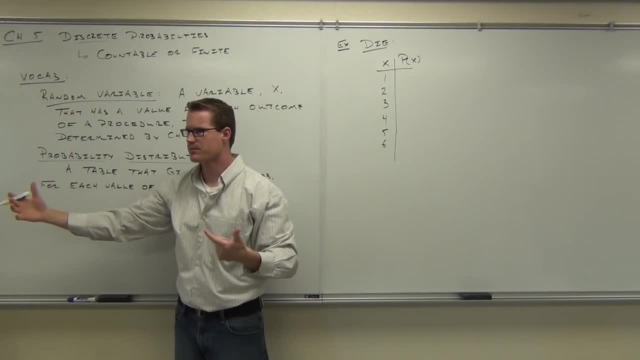 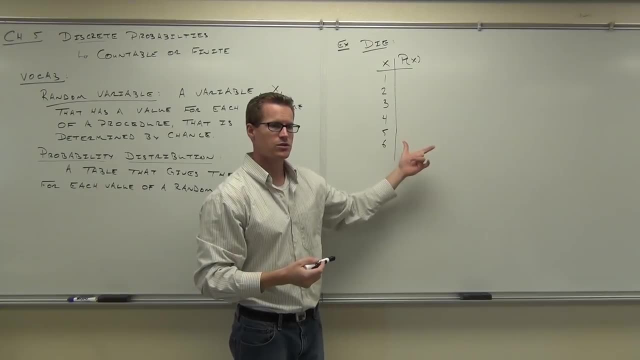 Rachel, are you okay with this? so far? Good, So you kind of understand the idea of a random variable then, right, It's just our outcomes that we can get from the procedure. Now the probability says what's the probability of getting each of these values. 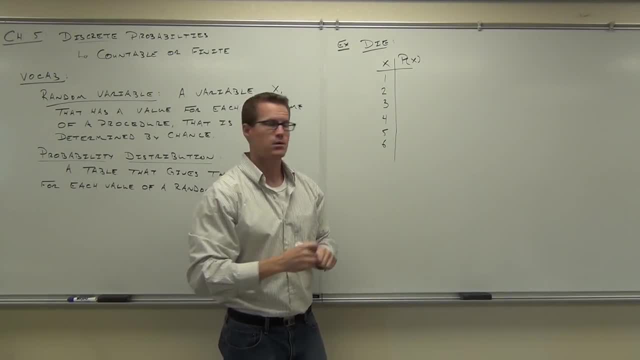 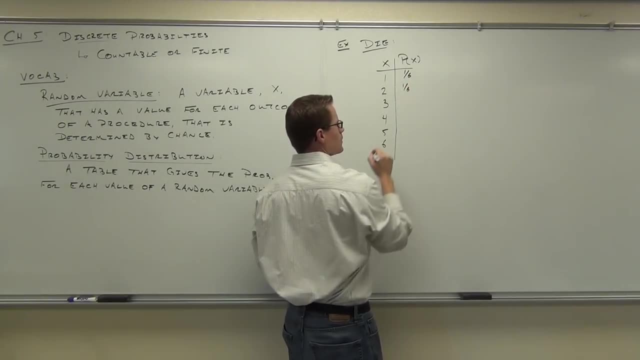 So what's the probability that you're going to roll a one, One, One, One? What's the probability that you're going to roll a two, One third? How about a three, One third? Is it going to change? 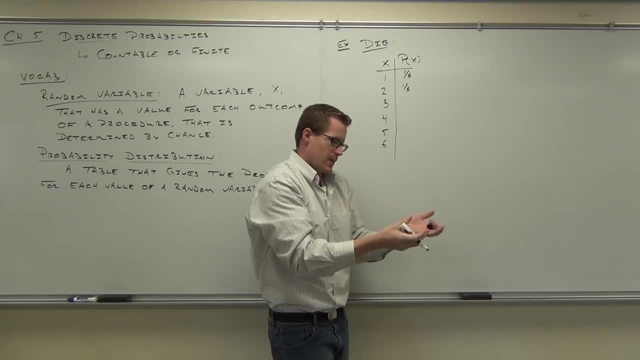 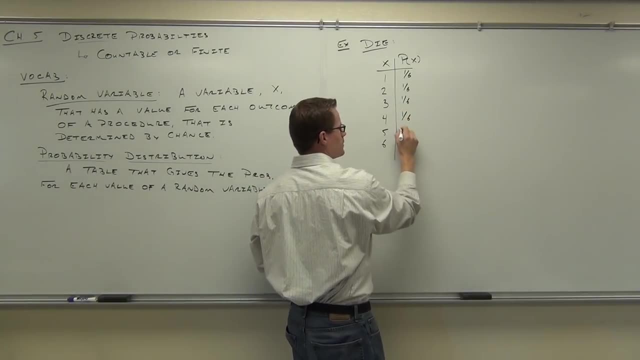 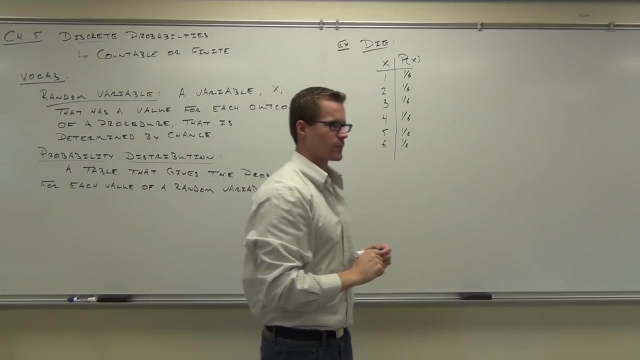 No, Not if you have a standard die right, Because that's the reason that we have a die, is that the chances are equal to get all six sides. We'd have one sixth for every value of our random variable, So we've got a couple things going on. 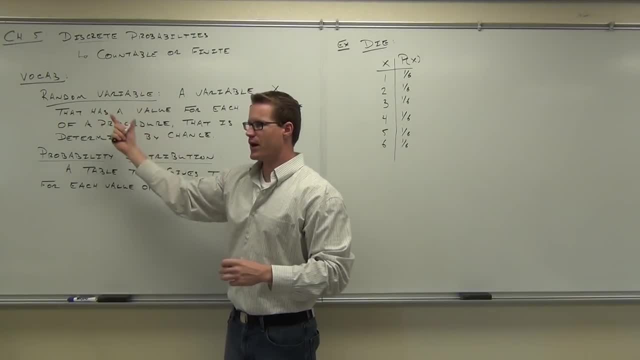 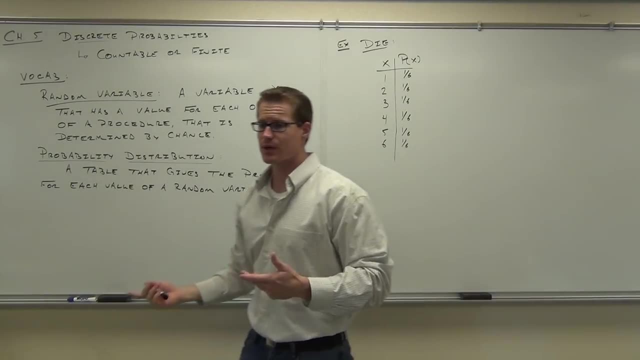 We have this thing called the random variable. That's just telling us that the value of our outcome can change. but the random variable has to take the place of every possible value. So one through six in our case, for the die, The probability, that's just what's the chance. 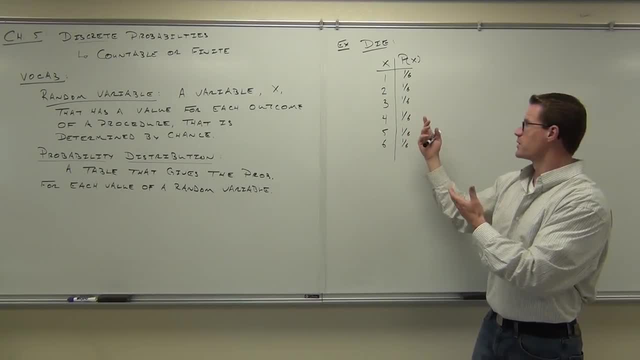 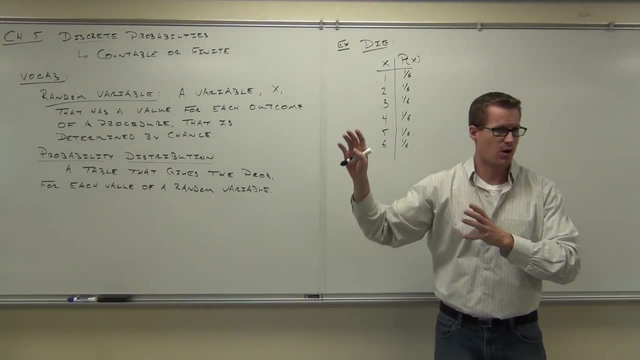 Again, it's classical probability here, isn't it Classical probability? What's the probability that you're going to get each of these? Now? we can use either classical probability or observed probability, depending on the context of our problem here. I just want to reinforce those concepts as we keep moving through this stuff. 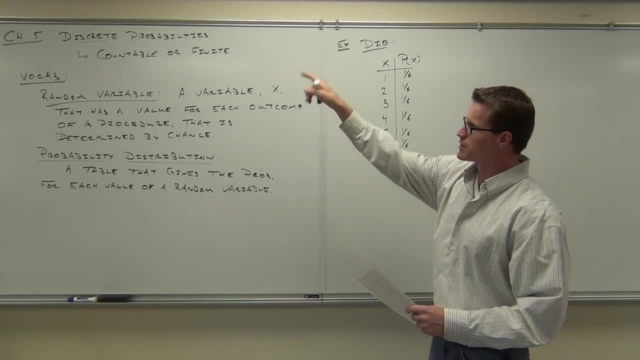 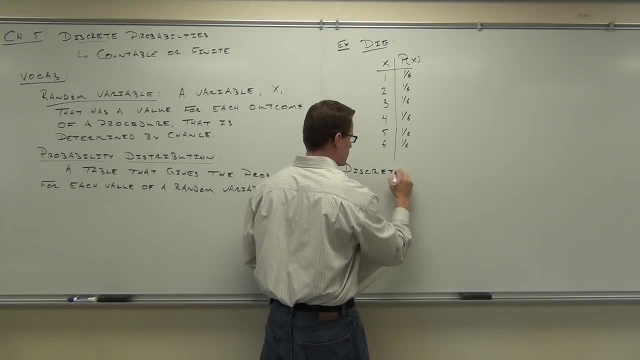 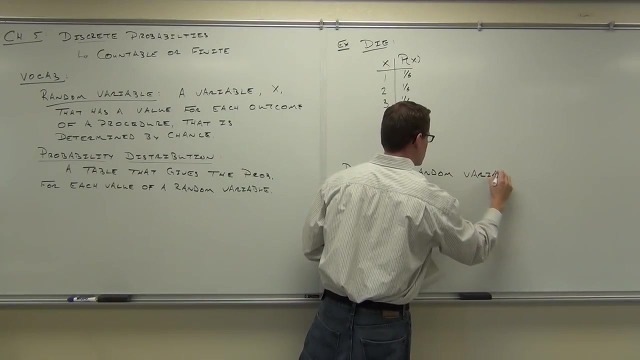 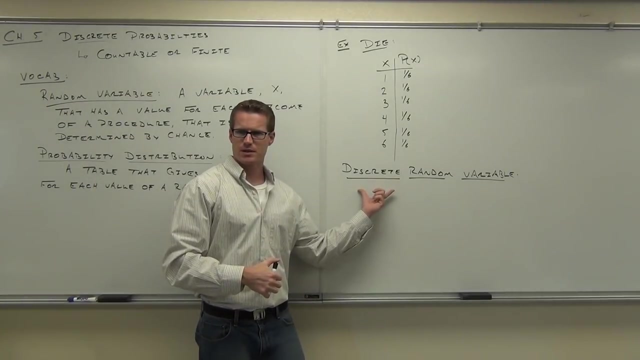 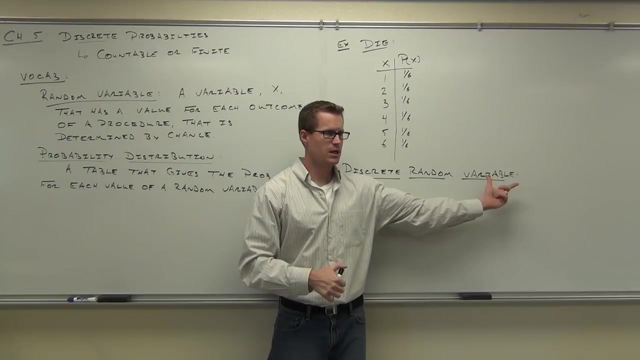 So we have a random variable, We have a probability distribution. We haven't really talked about discrete yet. A discrete random variable- Discrete means What was discrete, mean again Countable, Sure Countable, or finite. And random variable, those are just the values of a procedure that we can get. 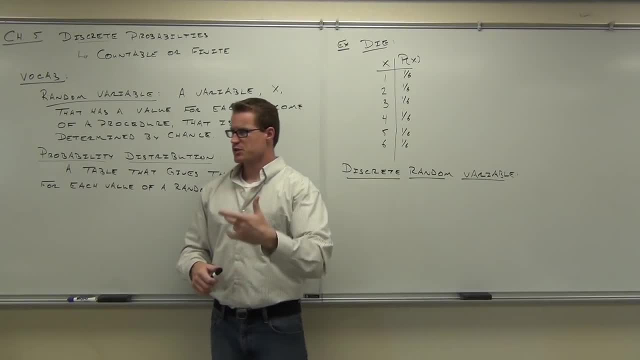 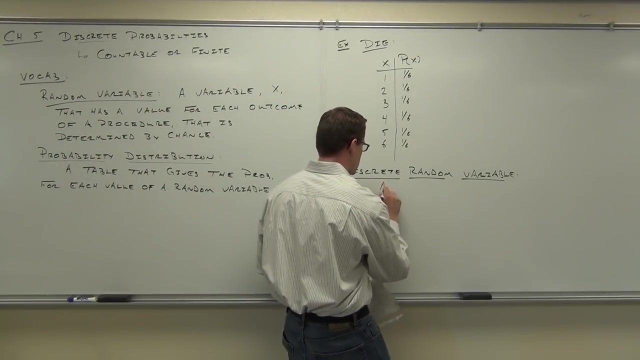 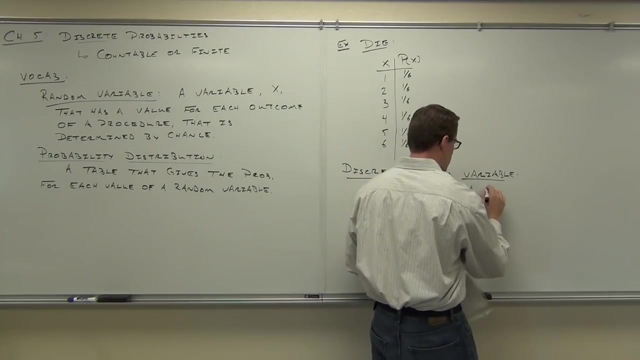 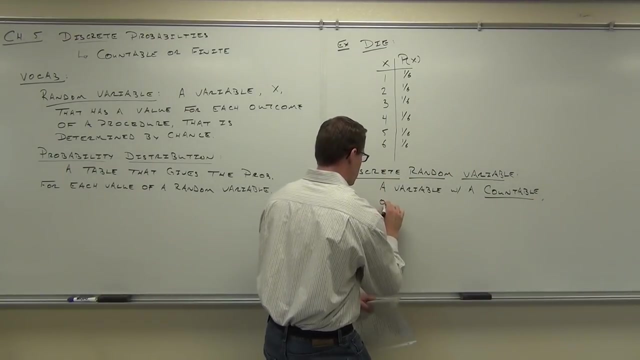 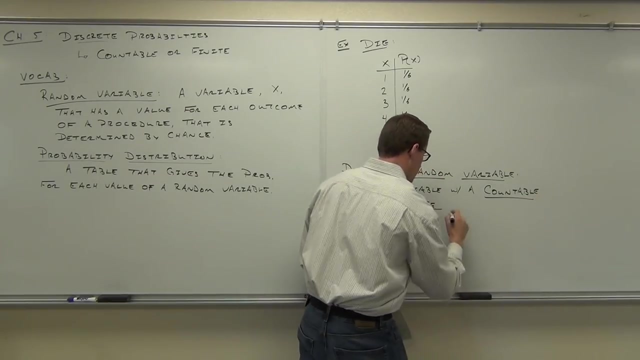 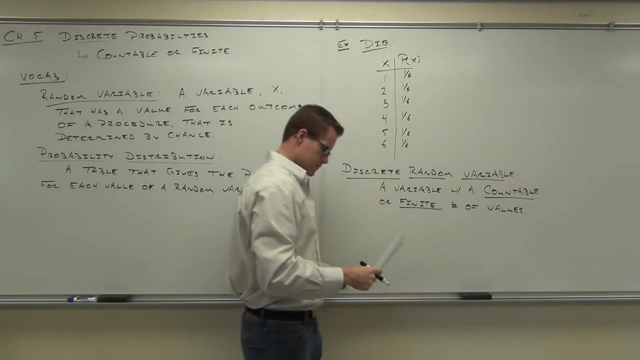 So a discrete random variable signifies a procedure where all you can get out of it are countable or finite number of items. That's what a discrete random variable signifies. So it's a variable with a finite or countable number of values. Okay, examples of discrete random variables: 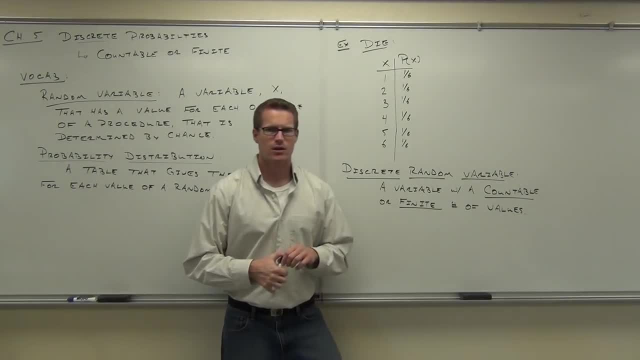 Okay, Examples of discrete random variables: Discrete, If I counted the people in this classroom, that would be discrete, because I couldn't get something like 42.3785 people, could I? Geez, I sure hope not, That'd be gross. 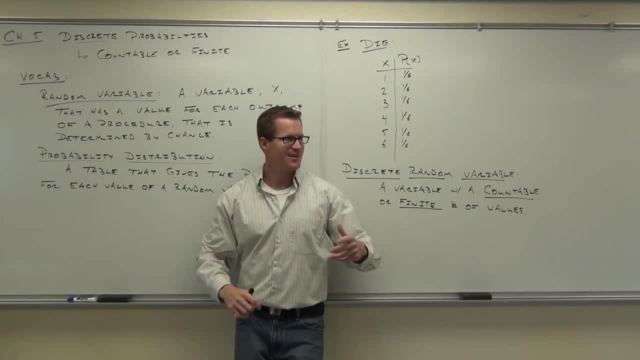 It's not even Halloween yet. I'm talking about dismembering people and stuff. No, no, You're going to get a whole number of people right. We can count every person that walks in this room. That would be something that's discrete. 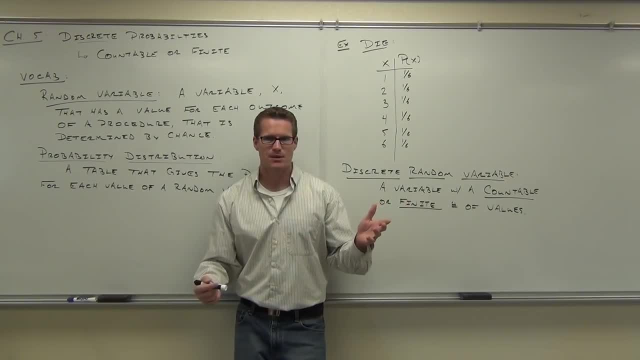 Or I use this example all the time- but if you count up the number of eggs a chicken can lay in a week, that would be something that's discrete or continuous. What do you think Is it going to lay? potentially 3.2 eggs. 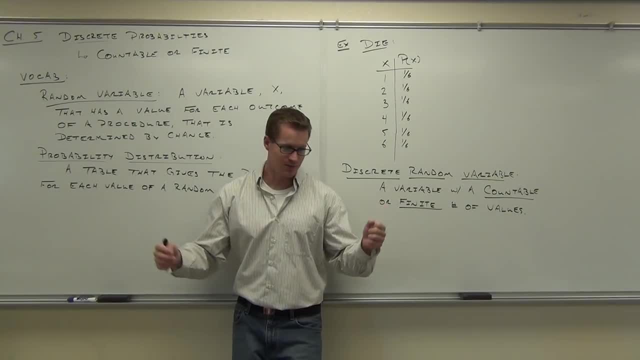 That'd be weird too. right, It's like I'm done. Didn't have to push that all the way out. 0.2.. Got it? Yeah, it's not going to happen. So this countable, this discrete idea is, you have a whole number of something. 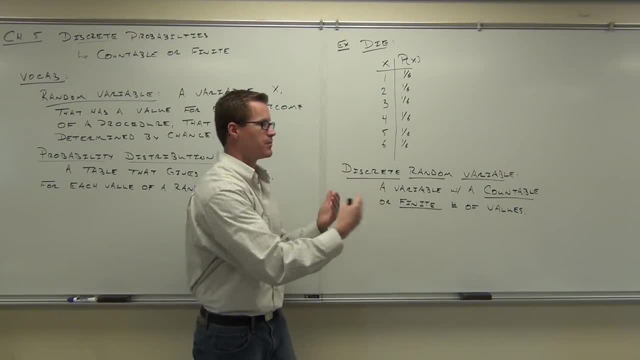 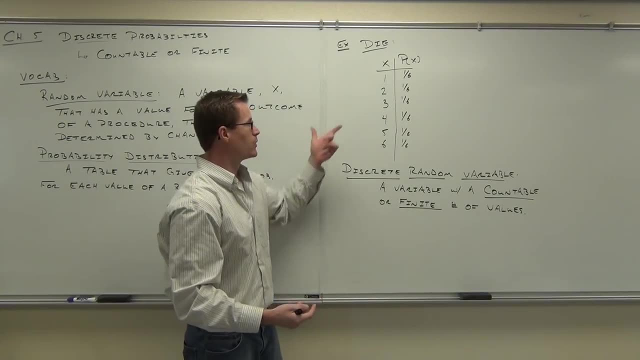 or it's countable or there's finite, So there's only a certain possible number of values you can actually choose from. So, for instance, if I labeled my die right, it would have to be 1,, 2,, 3,, 4,, 5.. 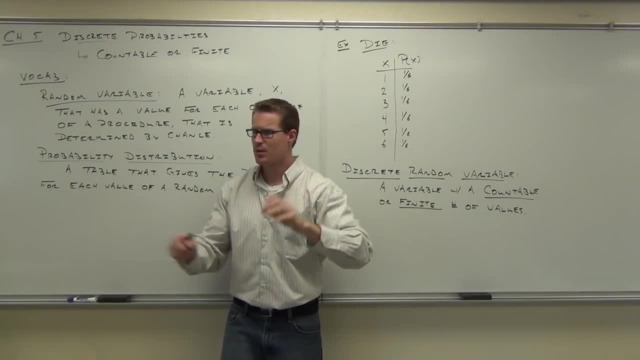 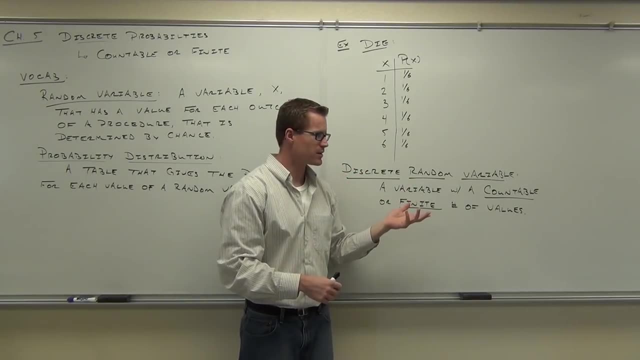 What if my die, my die, were labeled? There's only six sides still, but I label it 1.135.. That's one side. The other one's 2.002.. That's the other side. You with me on this. 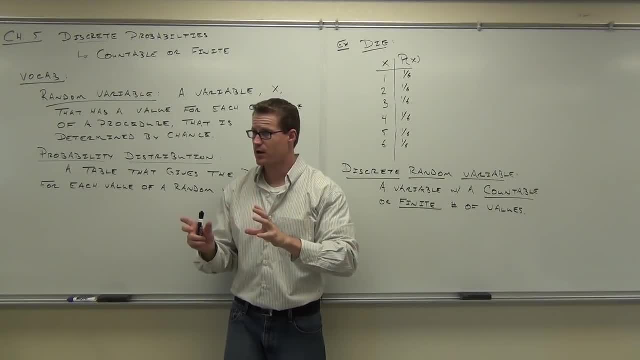 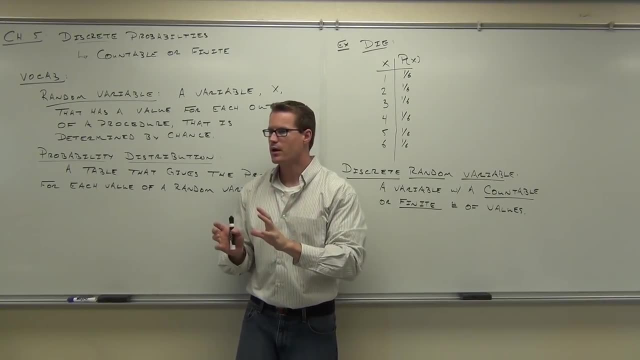 There's still only six choices. Even though I would have a decimal there, I can only get six things out of it. That's finite. You with me on the difference. So it not necessarily means a whole number, It means it's countable, sure. 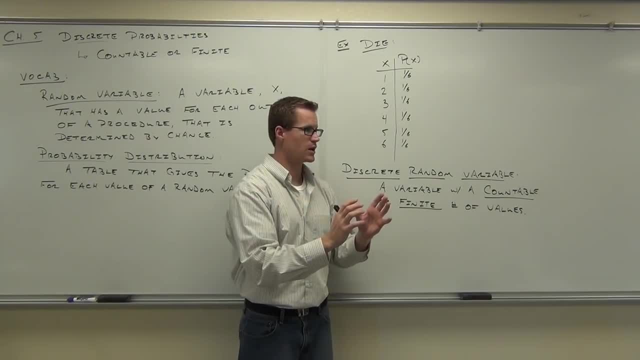 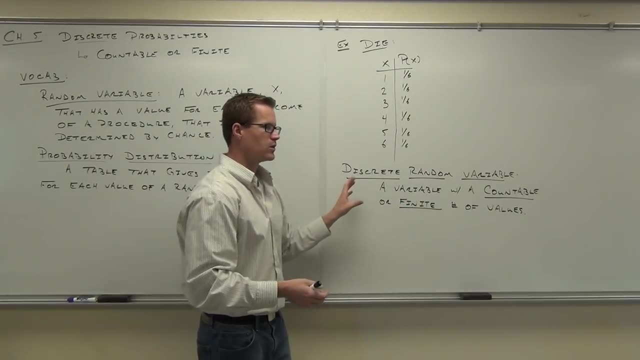 Or there's only a certain amount. There's only a certain amount that you can get out of your procedure. It doesn't have an endless number of possibilities. I'm not sure if you're with me on that. That's discrete, Countable, finite. 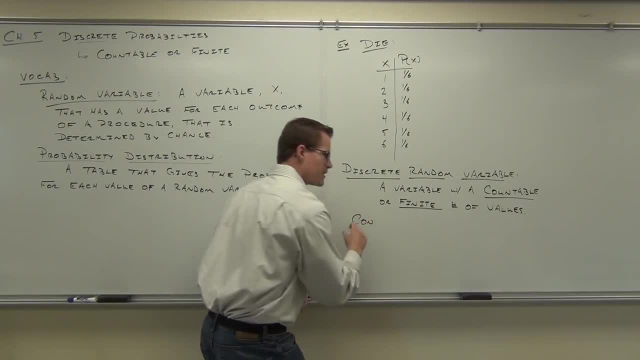 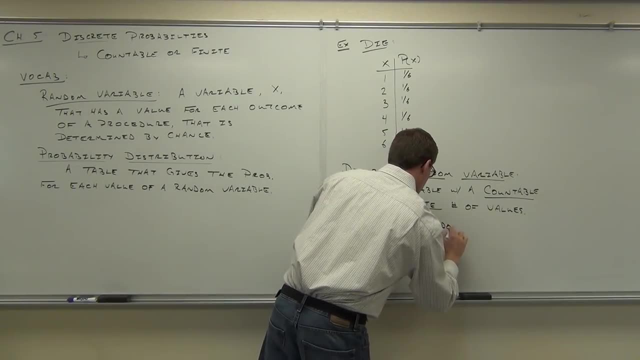 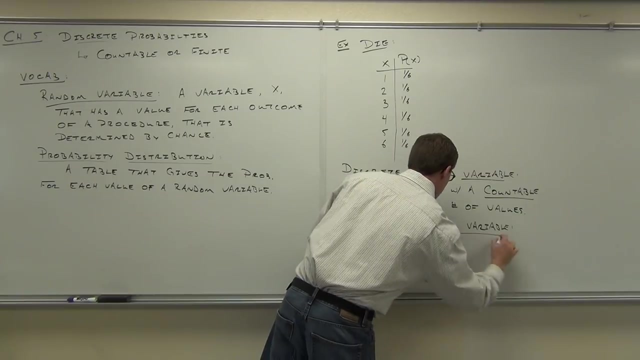 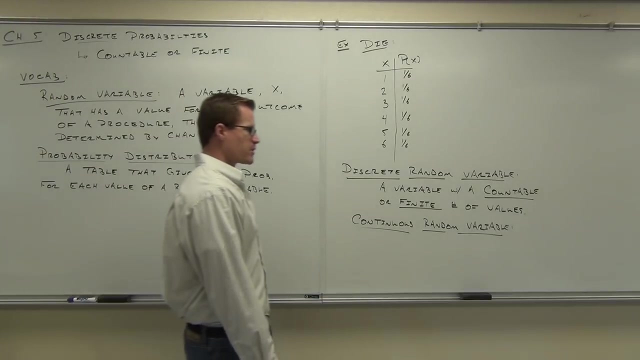 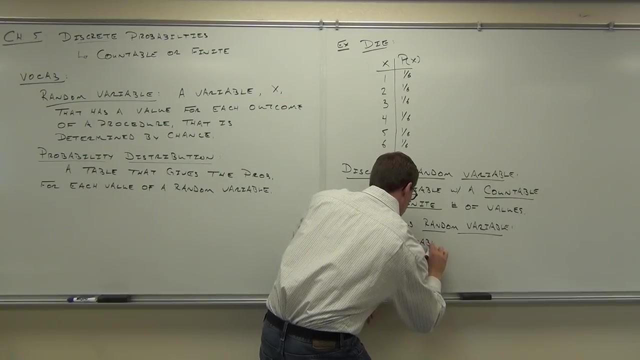 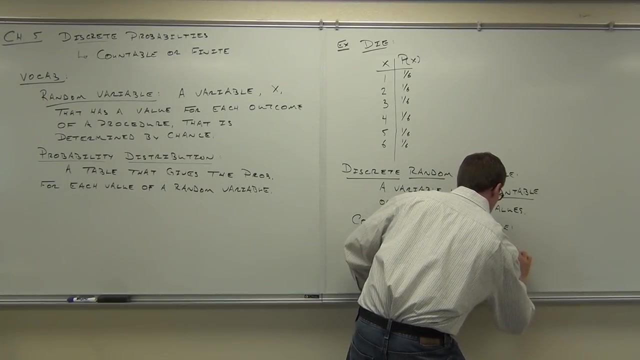 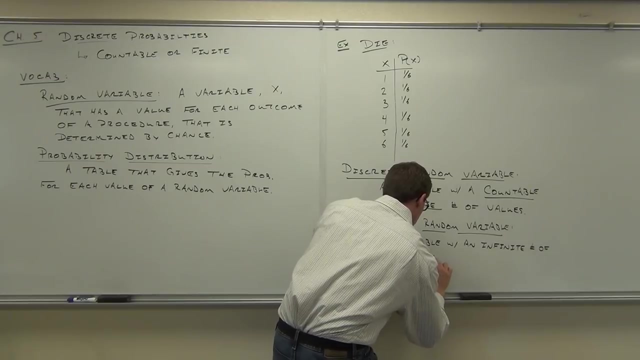 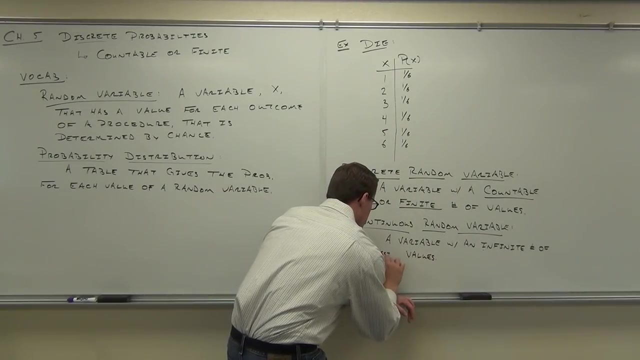 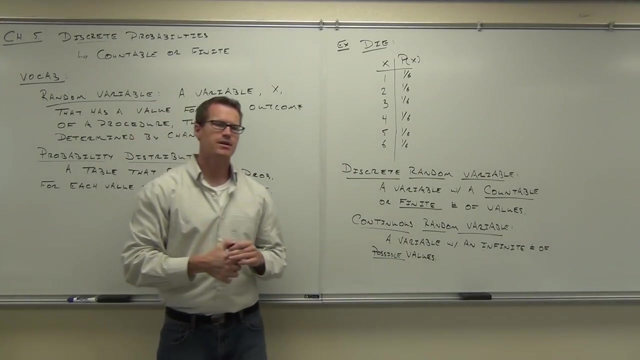 A continuous random variable would be everything else Uncountable or infinite. We'll just say infinite, A variable with an infinite number of values. Let me add one more word on there: An infinite number of possible values. Let me give you a for instance on this, because a lot of people get confused between discrete and continuous. 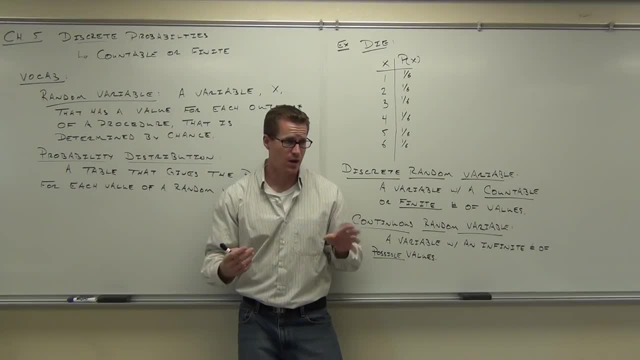 They're like. well, I know that discrete means countable- Keep counting them- Or typically, finite. There's only a certain number possible. How can we possibly get something that's continuous? Well, here's what continuous means. Continuous means an infinite number of possible values. 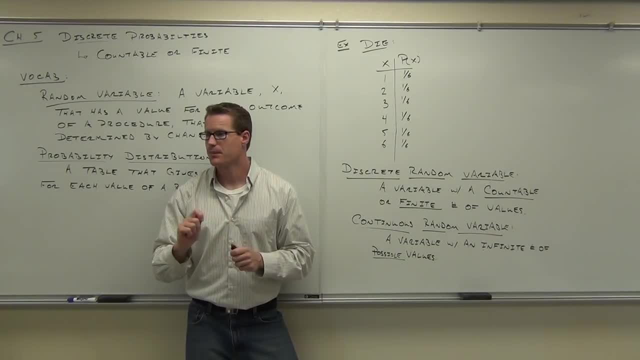 Here's the way this would work If you're picking people at random. if you're picking at people at random, do they have to be exactly 5'7 or exactly 5'8 or exactly 5'9?? Can you find someone in between there? 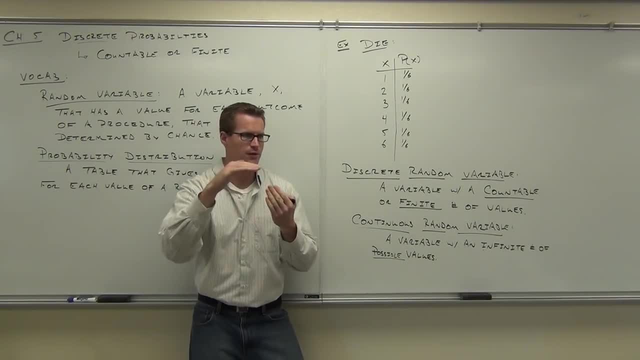 Typically, almost nobody is exactly 5'7, right? So let's say we found we have this range of 5'7 to 5'8.. That's our range right now. Can you find someone between 5'7 and 5'8?? 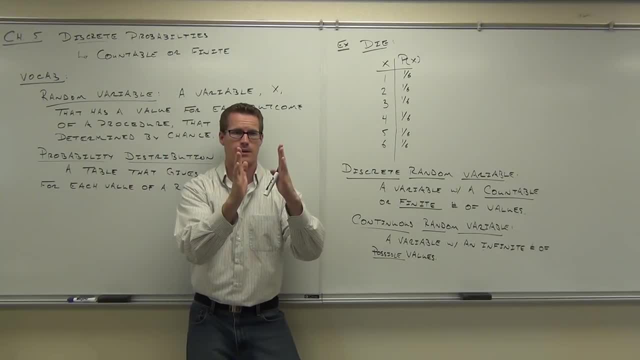 Sure, Let's say they were 5'7 1⁄2.. Is that the only two outcomes that you possibly get? Could you get more than 5'7,, 5'7 1⁄2, and 5'8?? 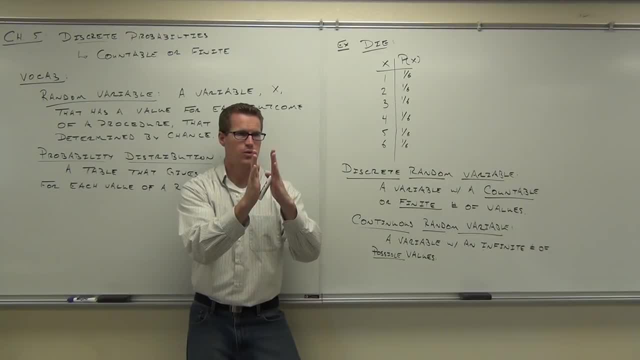 Sure, What if you pick someone between them? 5'7 3⁄4?. Do you see the point? You can always find someone between those two numbers. Are you with me on that? No matter how small you go, can you find someone who fits between there. 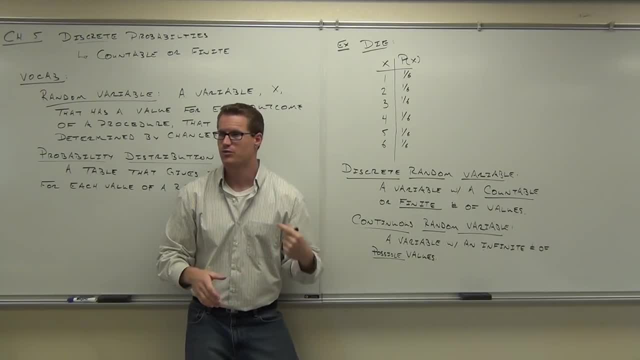 That means that if you keep doing it forever and ever, you have an infinite number of possible values And you can't count them. You can't say, oh, what's after 5'7?? 5'7.. What's the measurement after 5'7?? 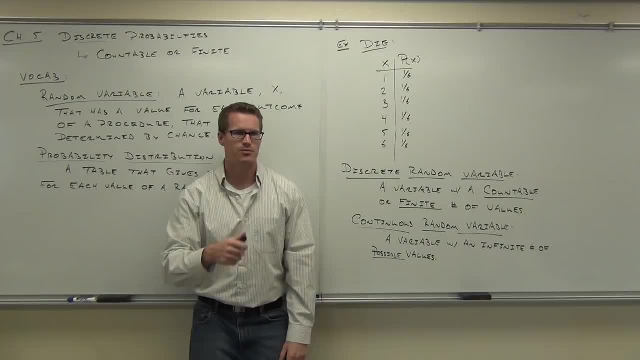 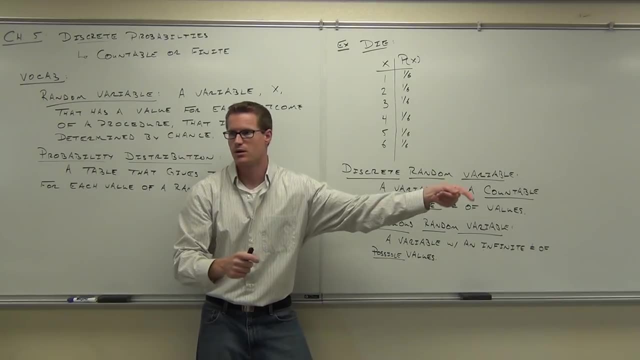 You can't just say it's 5'8, because you don't know how I'm measuring it. It could be 5'7.0000001,, right, But you can go 5'00000000001, and that would be uncountable. 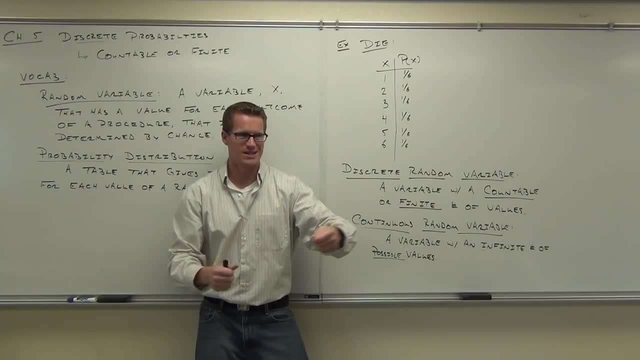 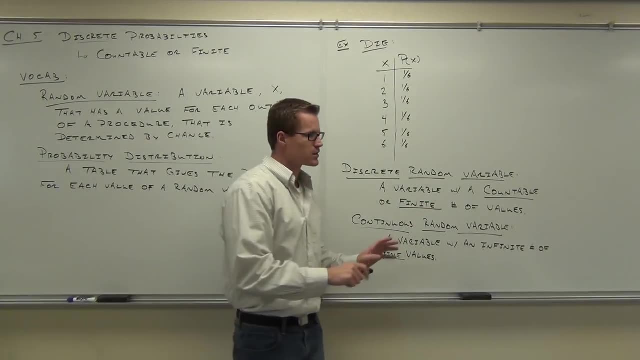 You can't say the next one in line, Do you get that? So it's infinite number of values and it's uncountable. Typically, continuous random variables are something to do with a measurement, Typically Not all the time, but typically. 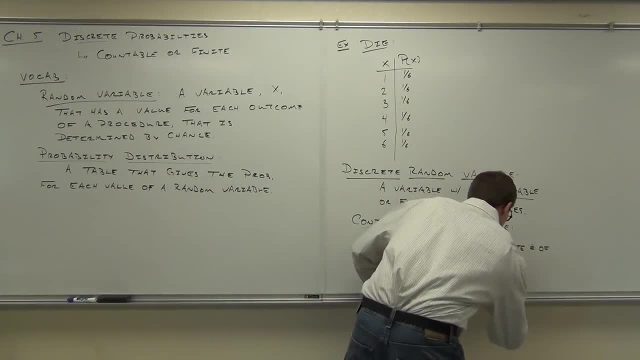 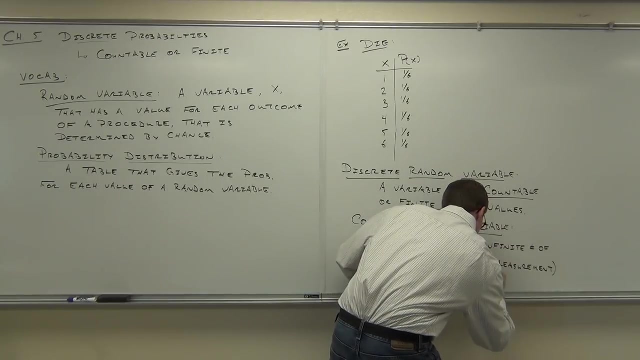 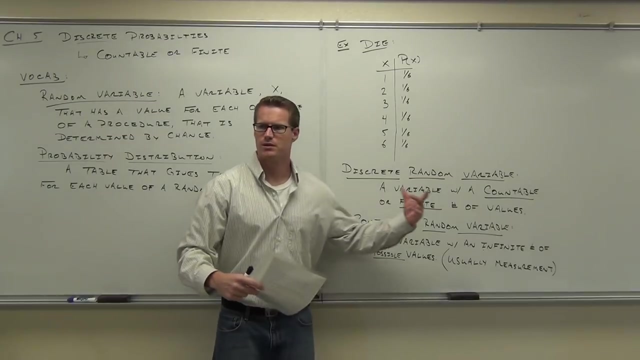 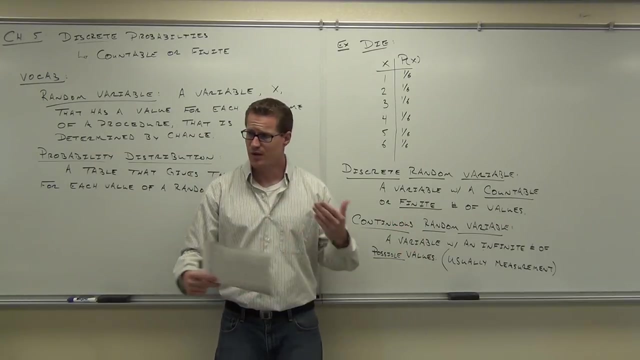 Volume, Weight, Height, Length, Temperature, Usual, Usual, Usual, A Usually Usually measurement. Do you understand the difference between discrete and continuous, Discrete, countable, finite, Continuous, infinite number of possible values, such as measurement, such as volume or height? 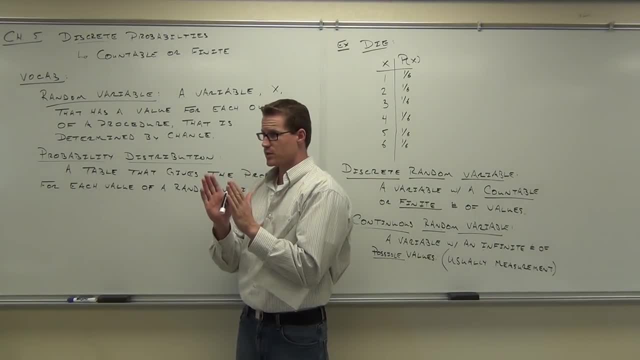 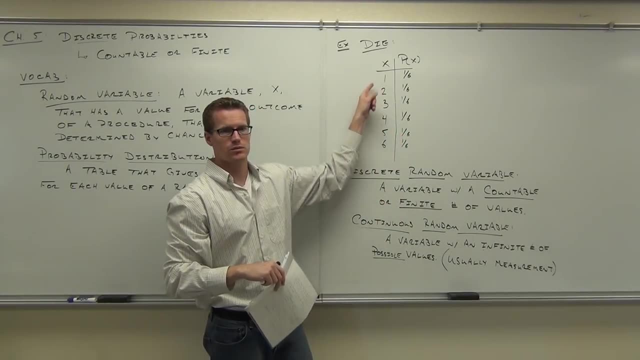 You can always find the way you think about that. you can always find a number between those two. Compare that to rolling a die. If you roll a die, can you ever get a number between 1 and 2? Can you do that? 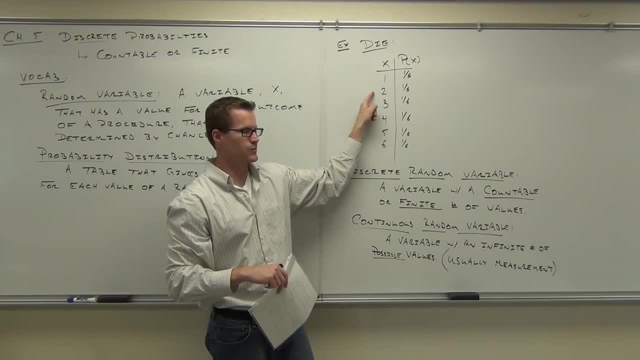 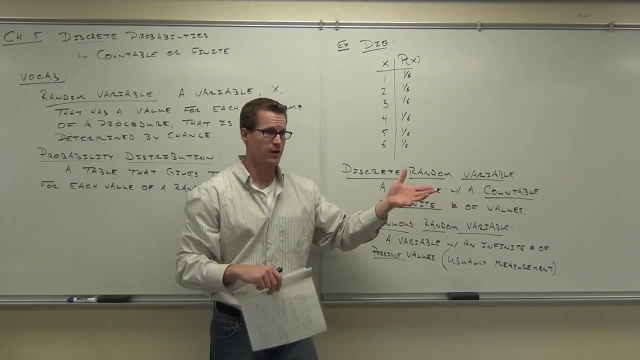 Can you roll a die and get 1.7?? No, That doesn't work. Not unless 1.7 is listed on the die, but it's not in this case. You can't get that. So that means that there's not an infinite number of values, there's only 6.. 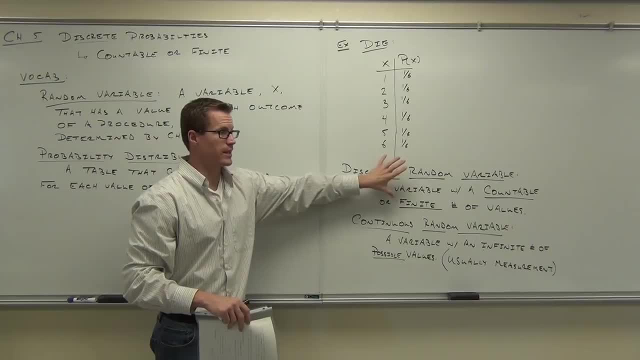 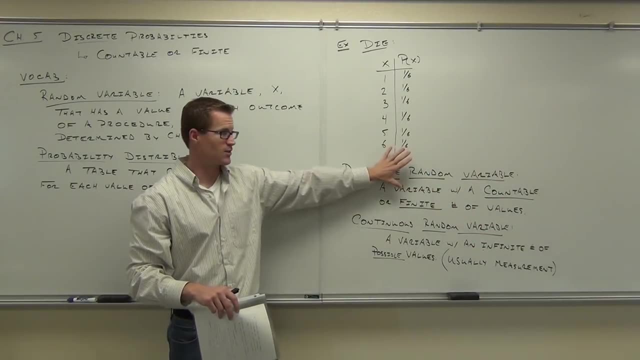 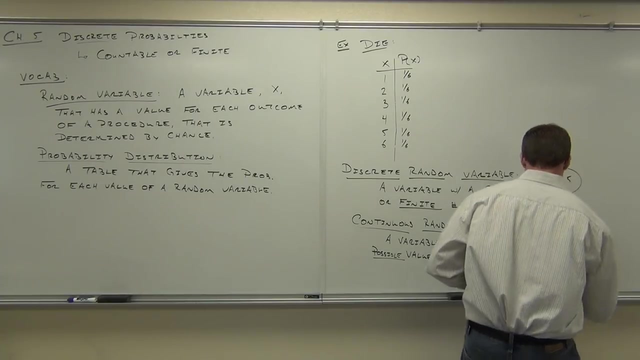 In chapter 5,. we're in this land, We're in discrete random variable land. The magical land of continuous random variables comes in chapter 6.. So chapter 5 here, chapter 6 here. 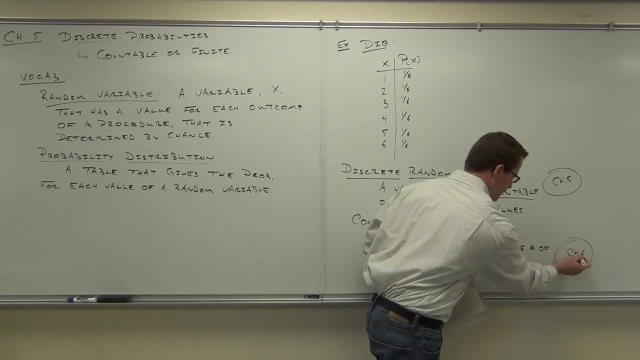 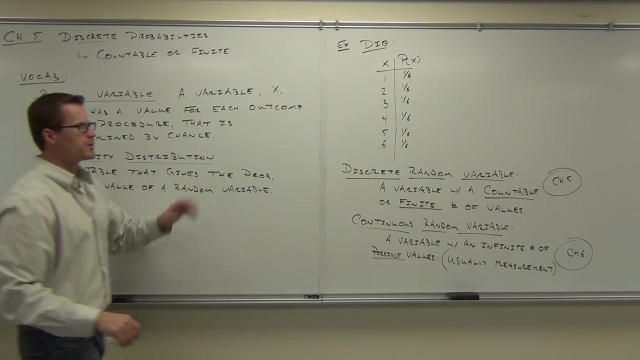 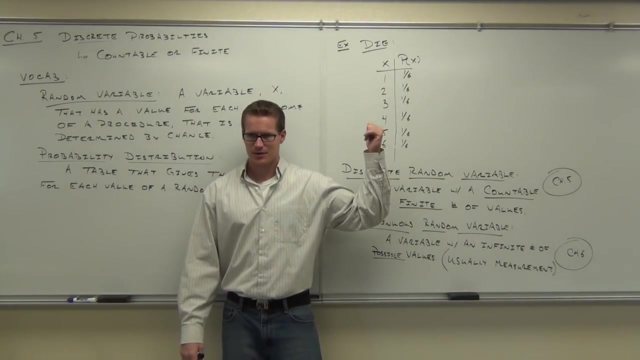 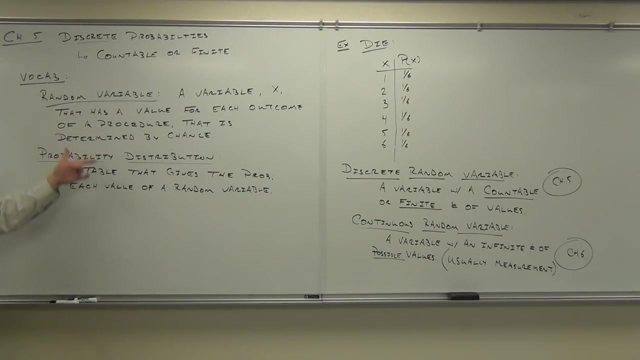 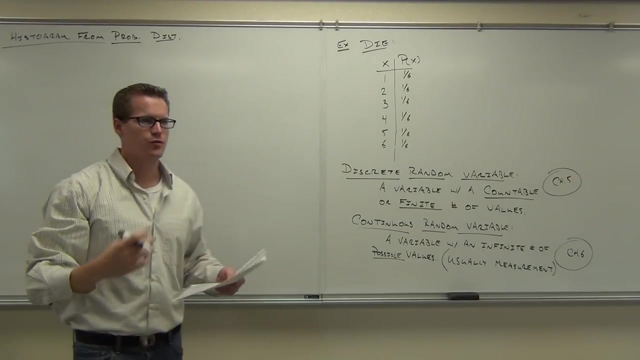 From a probability distribution. you know it's going to be really similar to a frequency distribution. 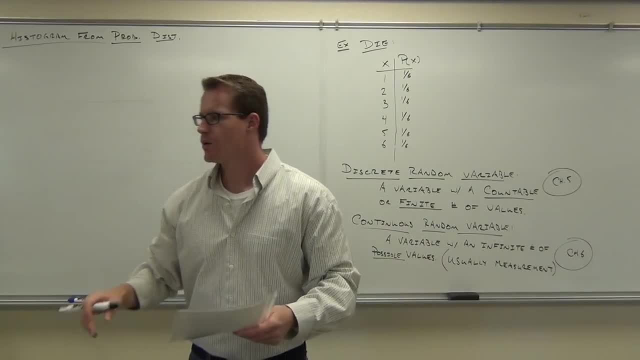 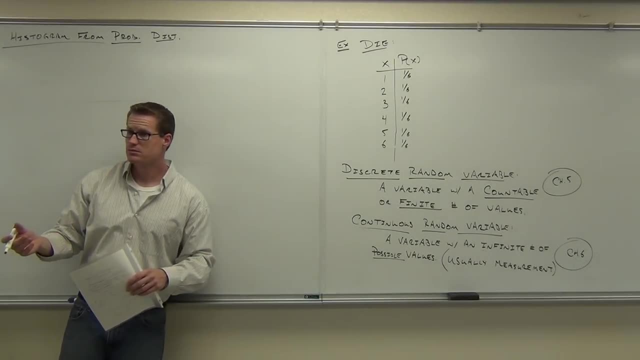 We're just going to have two axes. We'll have the x and the y. We're just dealing with the positives here. Can you ever have a negative probability, by the way, Ever? The probability of that happening is negative 2.. Does that make sense? 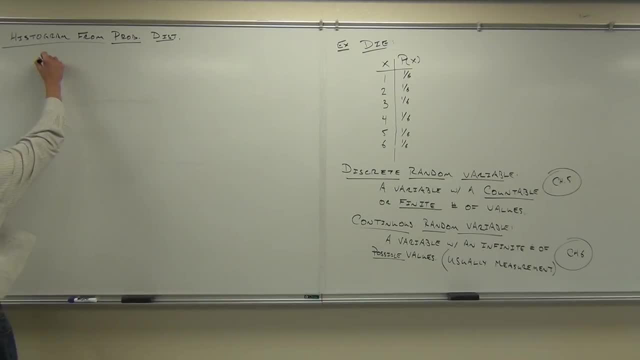 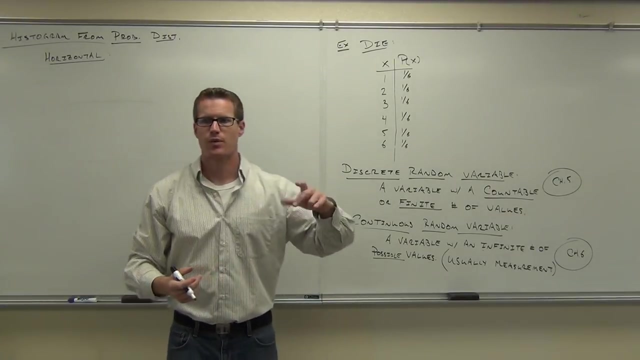 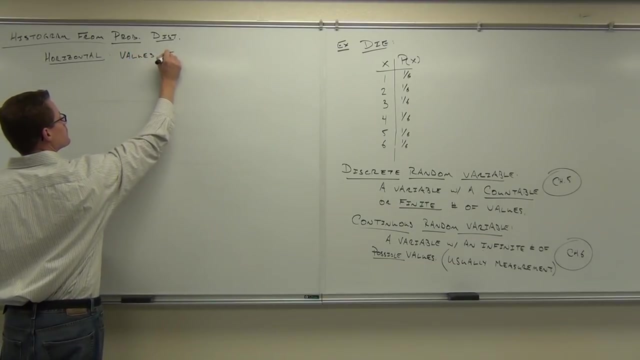 Probably not, not so much. So we're just dealing with positives. On the horizontal axis, we're going to have the values that x can take, the values of our random variable, whatever that has. Well, there's only two things. 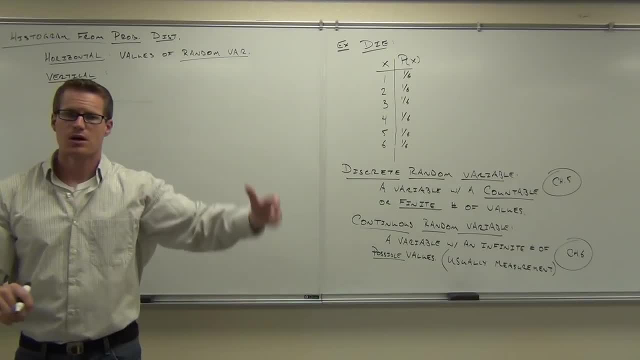 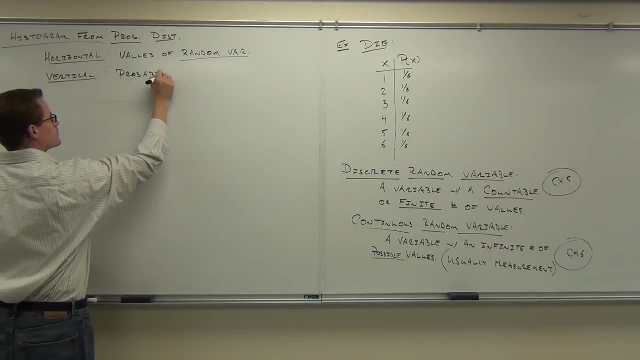 I mean, there's the values and there's the probability. So horizontal we'll have the values, Vertical we'll have the probabilities. But let's do something more interesting, because right now, if we were to graph that thing, can you see that we would just get a flat line? 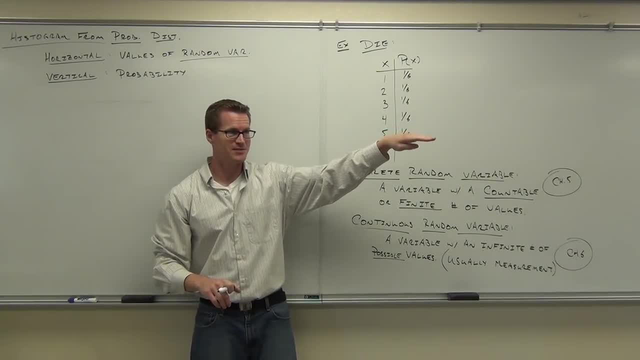 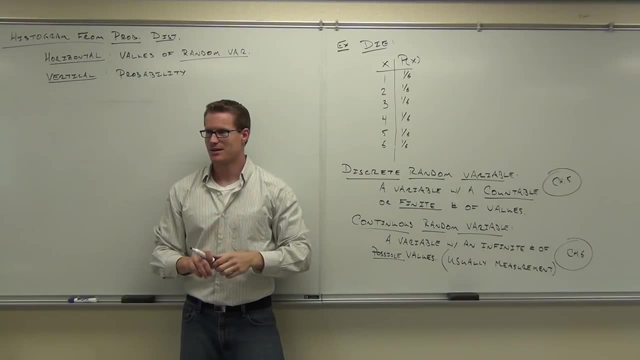 They'd all be 1 sixth. That'd be pretty boring. So here's what I've done. You see, I like playing craps and I like to win, So I made up my own little way to die. I cheat, whatever. 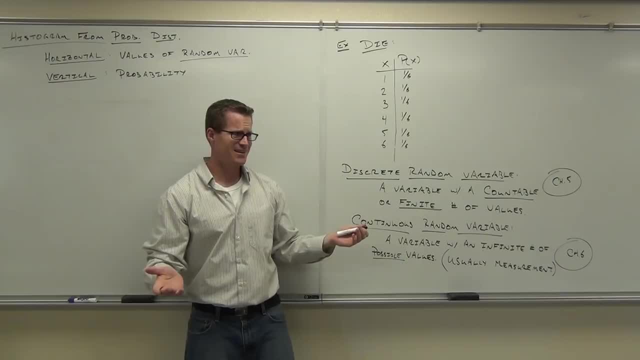 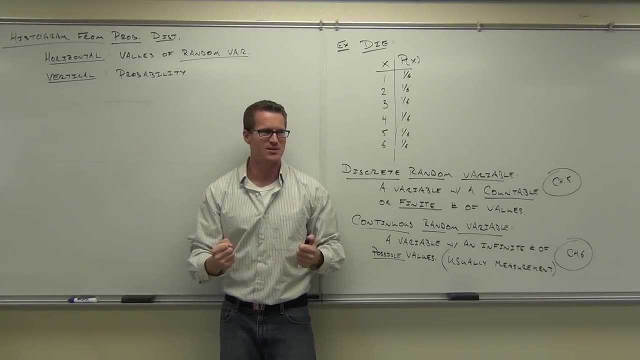 Cheater, Yeah, cheater, I die. It's money, man, Come on. No, I'm just kidding. You'd get seriously probably. well, I don't know if you'd get arrested, but they'd certainly beat you up in Vegas if you tried to die. 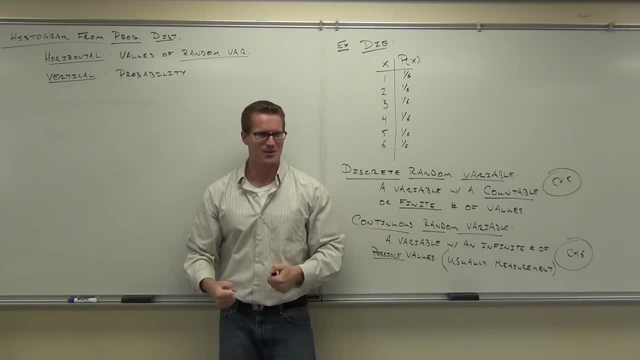 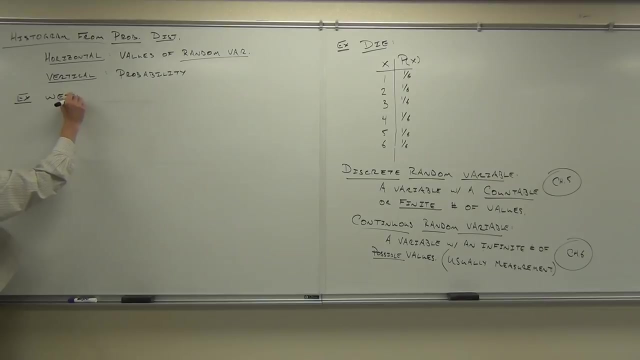 Have you seen the movie 21?? I don't want to do that, But I have a way to die. So let's say you have a way to die and I know even the probabilities for my way to die. And here they are. 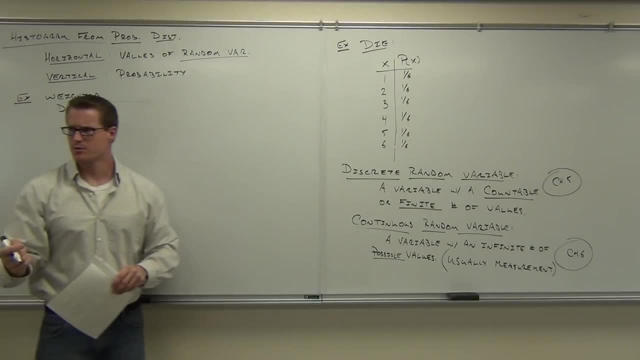 By the way, did I explain to you why someone might want to have a way to die when you're playing the game of craps? Because you want two numbers. You want 7 and 11. 7 is much more likely to get. get picked than 11, so you try to make 7s all the time And that's why you'd want a way to die Or whatever number you decided you wanted to have. If you wanted 8s, you just put all your money on 8,. 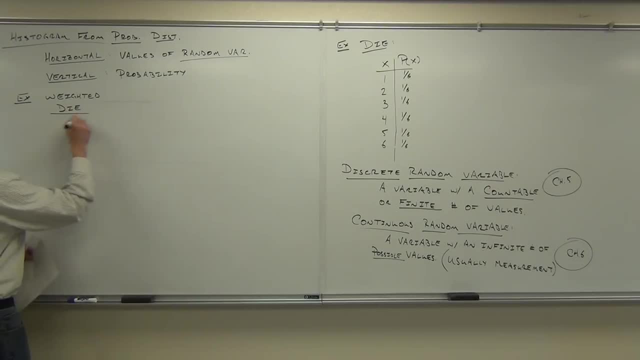 and you just roll on 8s. So we have a way to die here, and here's how my die works. By the way, what are my x's for my way to die? It's still a die right. You still get the same values. 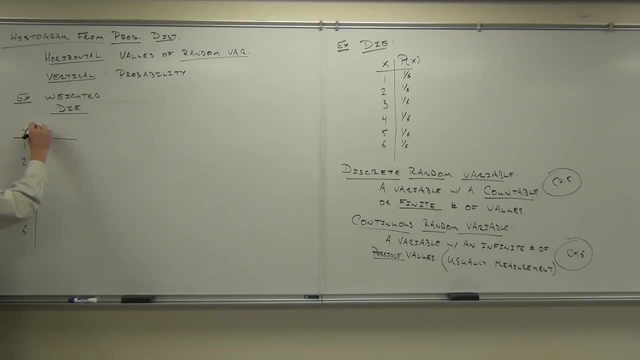 But what you don't know is the probability for each value. So here is the probabilities: if you roll my die- 0.5, or 5% of the time- you're going to get a 1.. A 2 occurs 15% of the time. 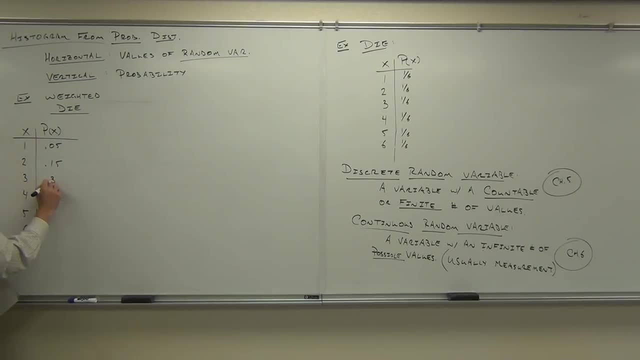 A 3 occurs 35% of the time or 0.35.. A 4 occurs 30% of the time, A 5 occurs 10% of the time And a 6 occurs only 5% of the time. 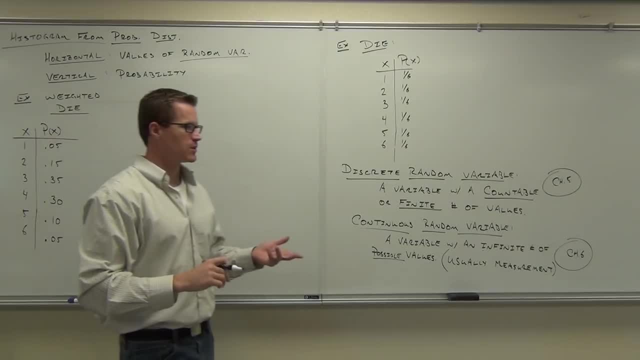 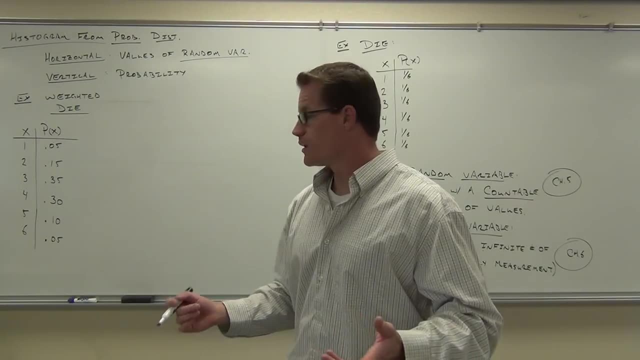 Hey, before we go any further, I need you to be able to identify whether this is a valid probability distribution or not, Because people look at that thing and go, yeah, that makes sense Or that doesn't make sense. How would a probability distribution? 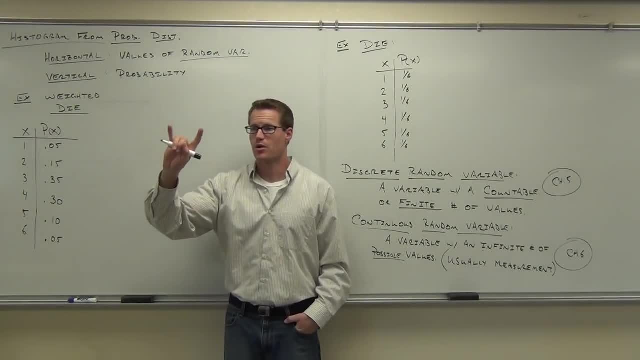 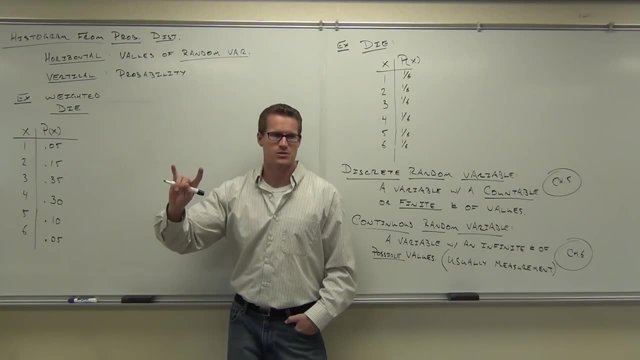 not make sense. Well, let's talk. There's only two ways. a probability distribution would not make sense. Let me ask both questions. Firstly, are all these probabilities positive? Can you ever have a negative probability? Then one way: a probability distribution. 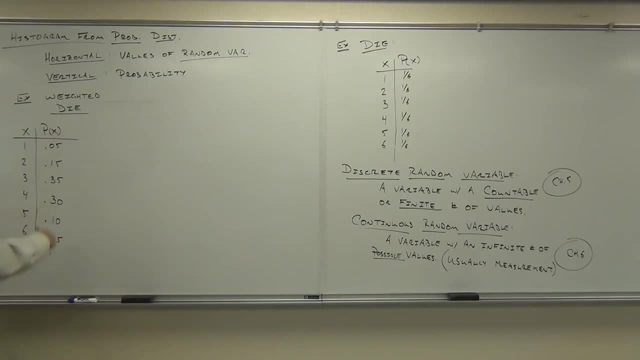 would not make sense would be if one of these were negative. They go: oh yeah, you roll a 1, it's this, roll a 3, it's a negative 35% probability of getting a 3.. Yeah, that wouldn't make sense. 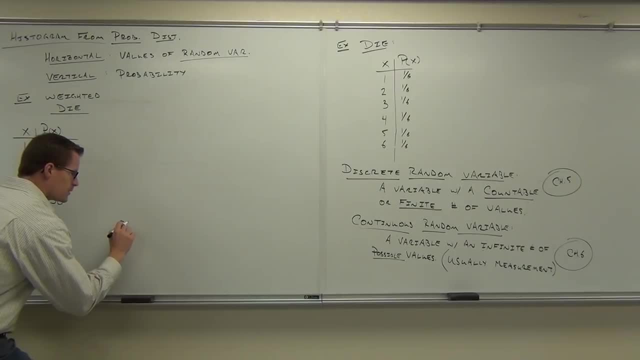 So first thing we know about probabilities is that every probability must be between 0 and 1.. So this is first note That's got to happen. So you look down at your probabilities. Are they all between 0 and 1?? Yes, no. 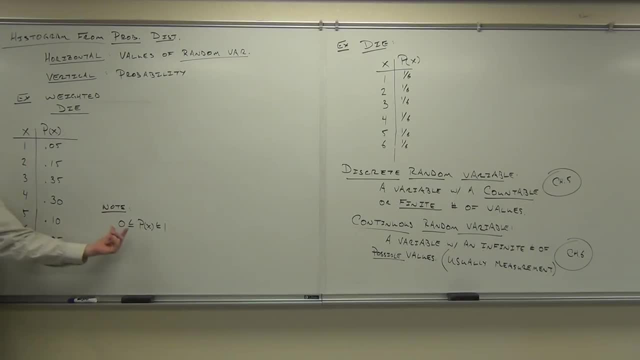 Yes, that makes sense. That's good Between 0 and 1.. Could you have the 0 and could you have the 1?? Can you have a probability of 0?? Yes, Sure, yeah, yeah, Can you have a probability of 1?? 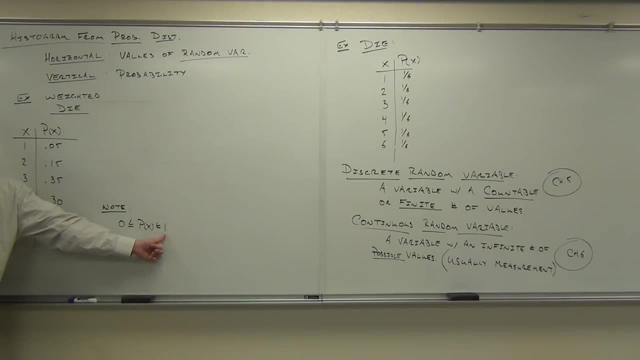 Absolutely. That's OK. That means a certain outcome is going to happen for sure. This means it's not going to happen for sure. Another thing: If this is a die, I'm rolling the die and there's a 5%, 50%, so on, so on, so on. 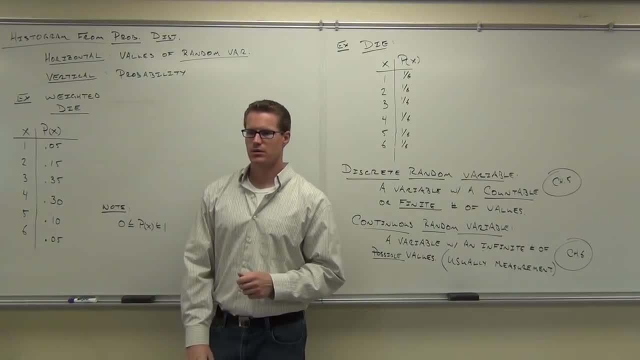 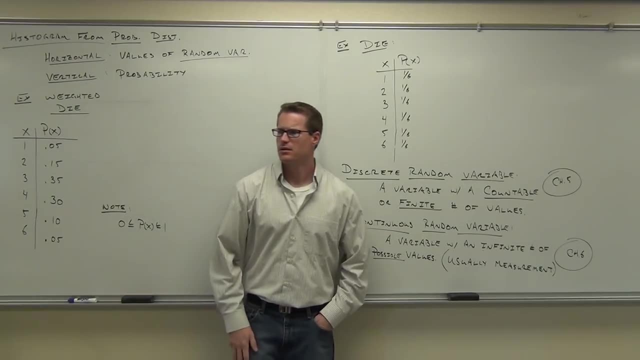 If I add all these up, what does it have to equal 1.. Why? Why does it have to equal 1?? You're right, it does, but why? I mean you know this intuitively right, I mean it's. 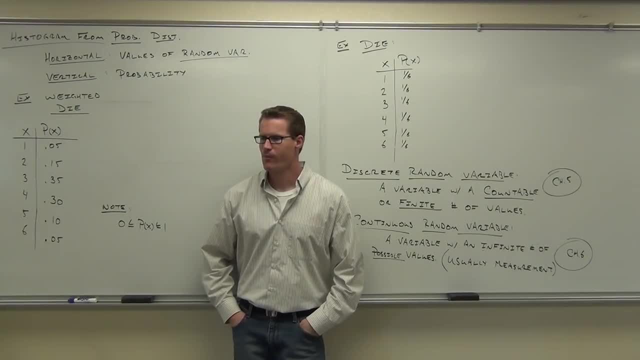 Explain it though, Because it's a percentage. OK, They are all percentages: 5%, 15%, 35%, 30%, 10%, 5%. The probability has to be less than or equal to 1.. For each one: 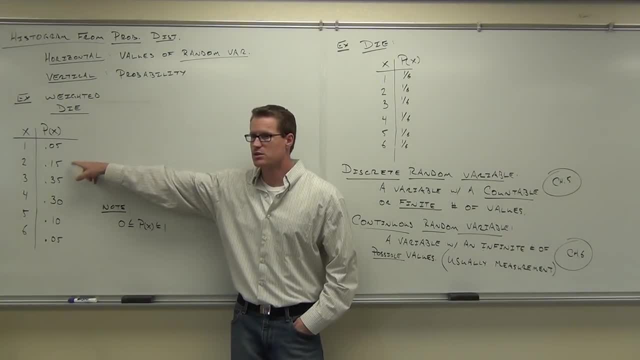 For each one it does. Yeah, so this has to be between 0 and 1.. That one does 2, and that one does 2.. But why is it that when I add them up I don't get something like 0.95?? 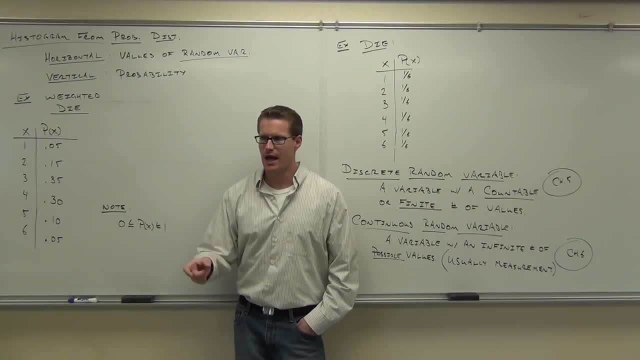 Or 1.3? Why does it have to equal exactly 1? You have to have all the information for it. What do you mean By? You might be on the same track, You might be on the right track, but what do you mean by that? 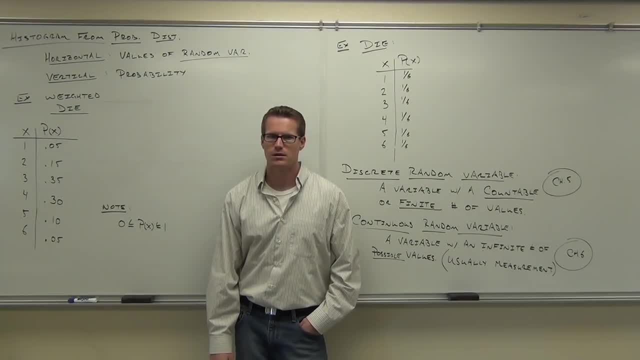 you have to have all the information. You're always going to get a number. Explain that. I mean you can't roll it, it's going to land on the side or anything. OK, so is it that when I roll a die? 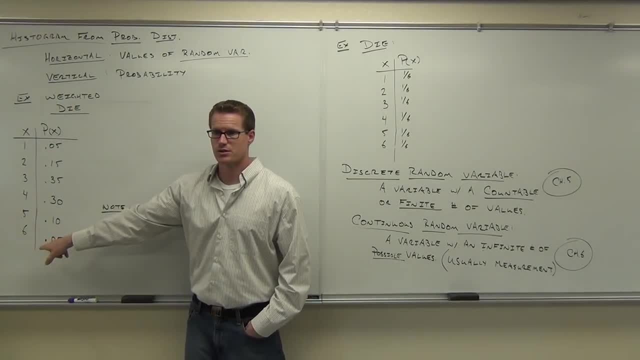 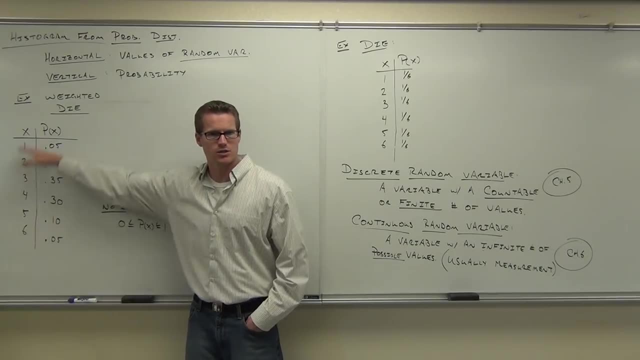 I am always going to get one of these numbers. Yes, So then, if I'm always going to get one of these numbers, is there any possibility that I'm not going to get one of these numbers if I actually roll the die? So, when I combine all of the probabilities, 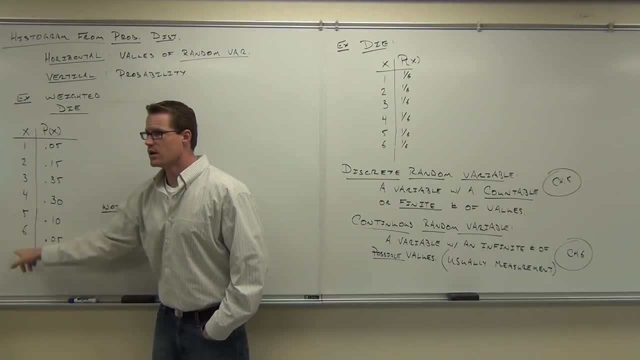 of rolling the die. it's here. true, There's a 100% chance I'm going to get one of these numbers. Do you agree with that? That's why, when you add up this probability, it has to equal 1.. 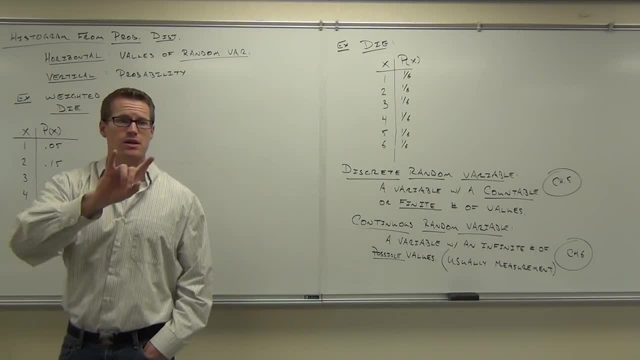 It can't be less than that. it can't be more than that. it has to be exactly that. So there's two things you're going to check for in your homework and on your test. when I ask you, is this a valid probability distribution? 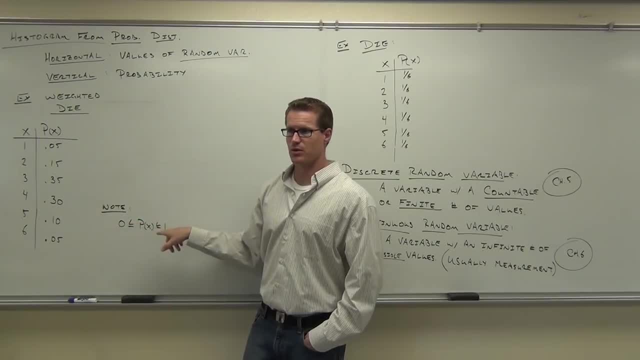 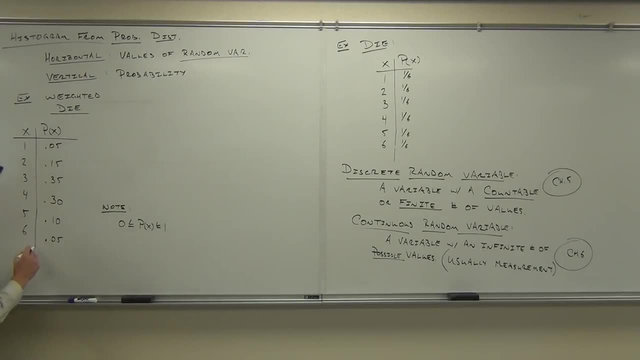 You're going to check, number one: are all the probabilities between 0 and 1?? Are they all there? Next thing you're going to check: when you add up all the probabilities, does it equal 1?? So number one. 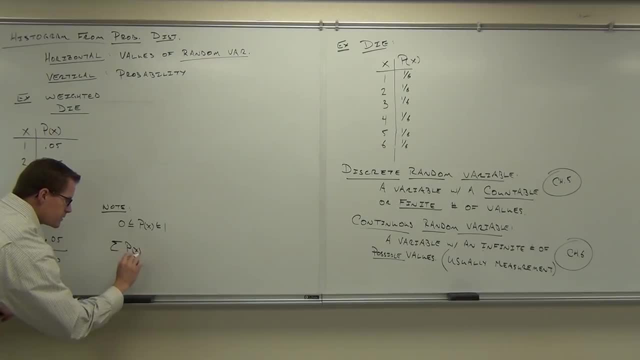 the sum of the probabilities has to equal 1.. On the exam, are you going to be able to put: has to equal exactly 1, or, Oh, it'll equal 1.. Yeah, yeah, Exactly 1.. Now there are some cases. 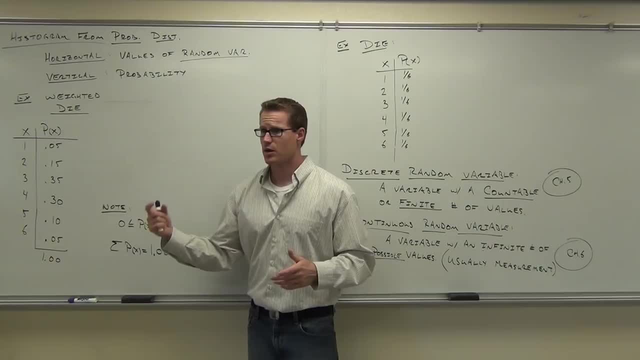 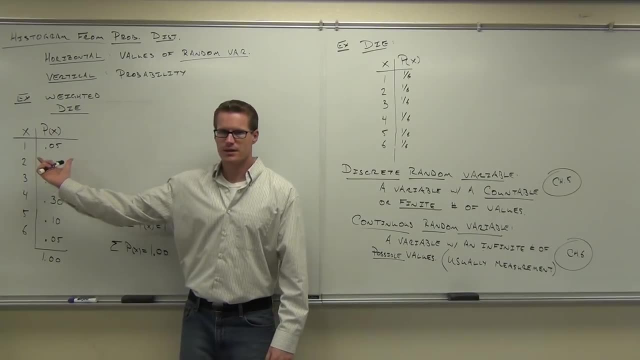 where, if you've rounded, like, if you're calculating probabilities on your own or the book is calculating probabilities on their own, they're going to give you exact stuff. But if they, if you have rounded some of this stuff, then there might be a chance. 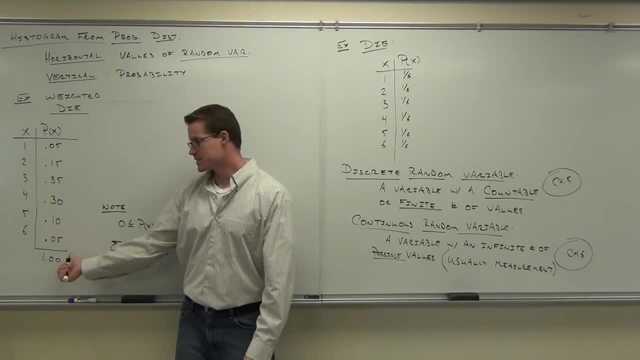 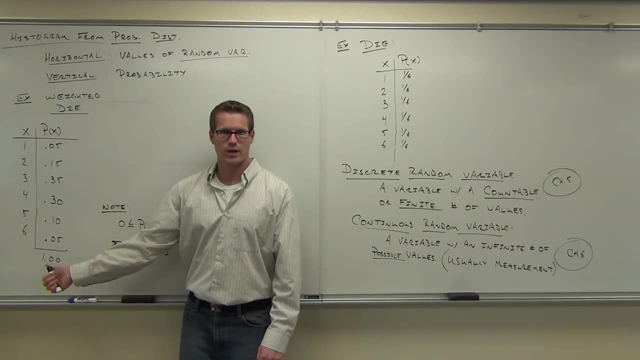 that you're off by just a little bit, but it's not going to be significant. It'd be like .0001, okay, or .9999.. It's not going to be like .8 or 1.7.. Okay, that would be way off. 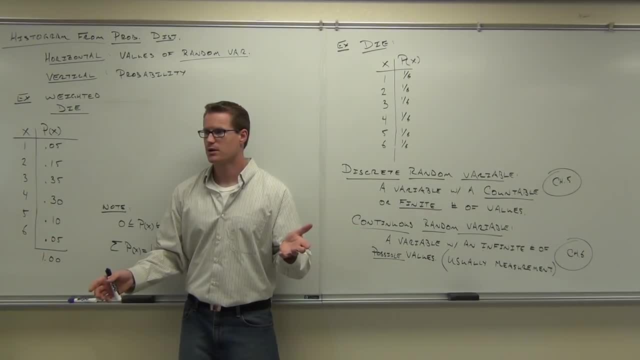 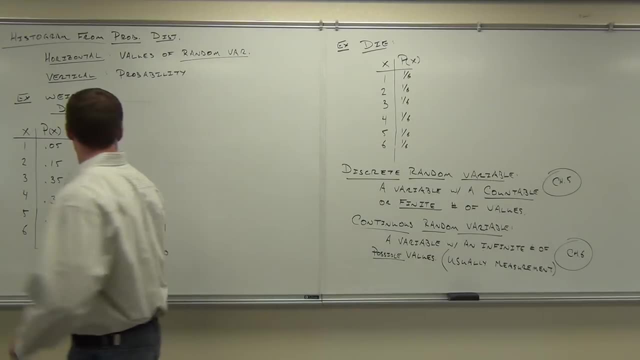 It's not going to even be like 1.2.. That'd be too far off. Or .97.. That's too far off. We're talking the thousandths and the hundredths. Okay, Let's go ahead and make up our probability distribution histogram at this point. 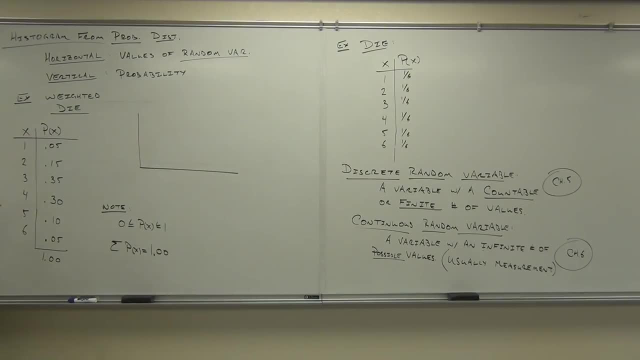 So we have this histogram now On the bottom, on this horizontal axis. what we're going to be doing is putting the values of our variable, Since there's six possible values plus six columns going upwards, six bars: One, two, three, four, five. 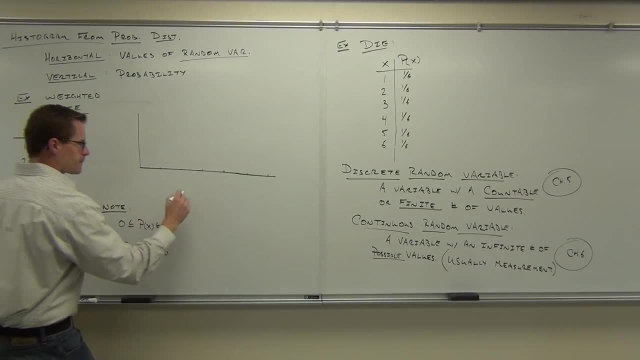 There we go. So x values go here and the probability of those x values goes here. So maybe we'll do something like five, ten, fifteen, twenty, twenty-five, thirty and thirty-five percent, Or .05, and so on. 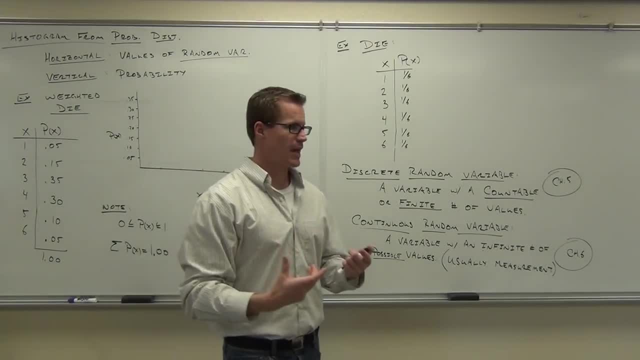 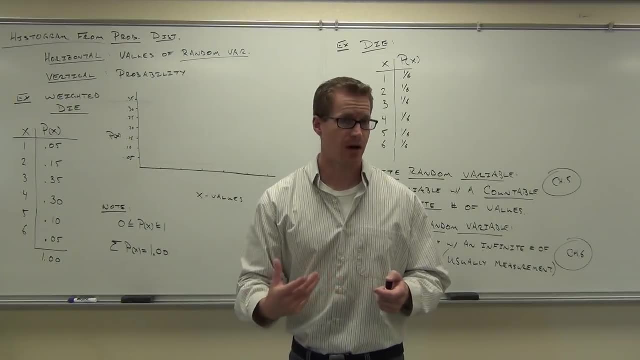 By the way, this could be one of those cases where this probability actually comes from observed data. So maybe I actually went and rolled my die a thousand times or a hundred thousand times and maybe I got the information from that. It could come from that. 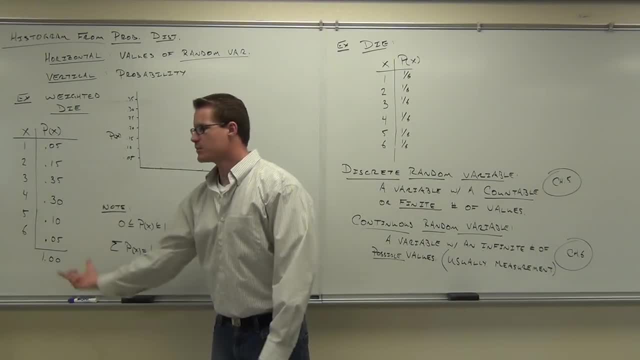 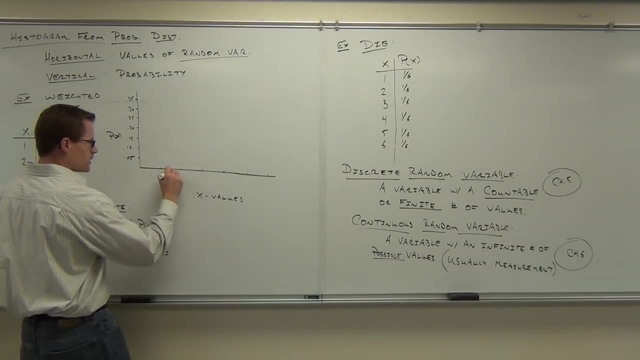 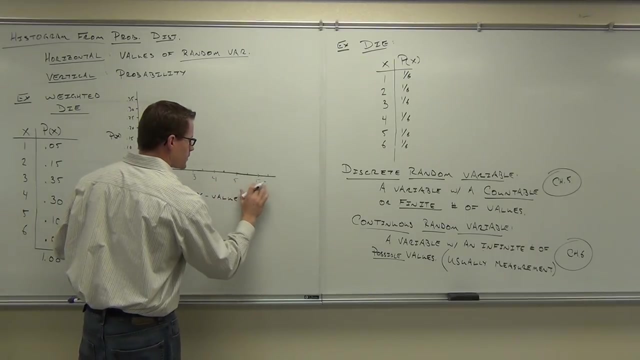 It doesn't matter whether it's classically based or whether it's observed based. You can still do the same things with it. So here we'll use our values. This is a one and a two, and so on And from: Can't have that twice. 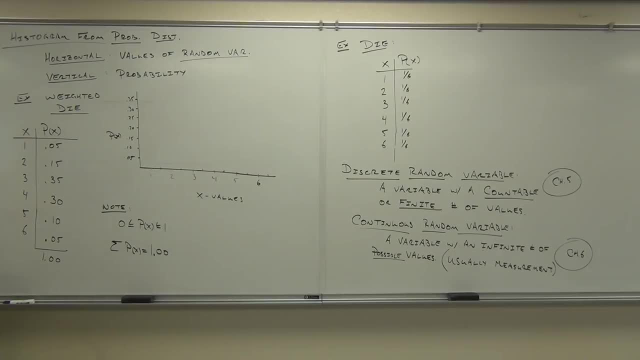 From here, we'll just make up our bars. What probability? What's the probability of getting a one here? What did we find? Okay, so very much like our last histogram we made up in this class, which was quite a while ago. 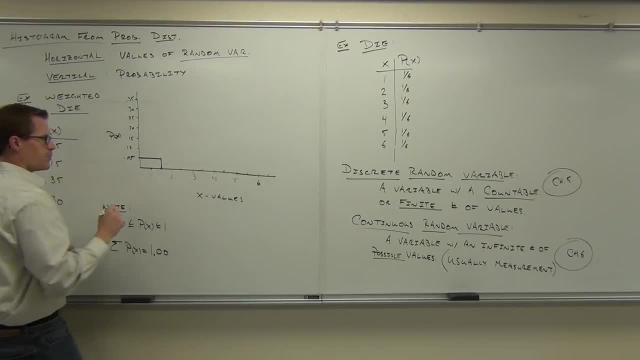 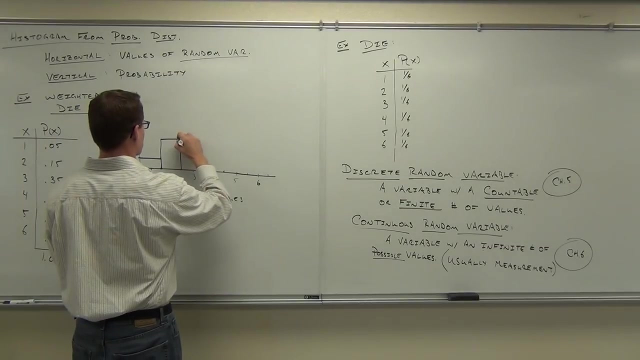 we're going to go from one, go .5, make a bar. Next one was at .15.. So for our two we'll go to .15, make our bar. Three, wow, thirty-five percent, .35, that's way up here. 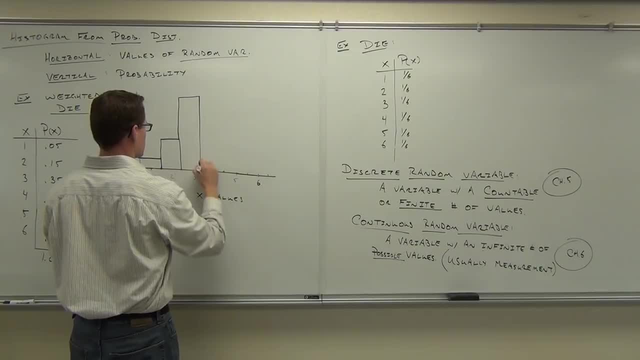 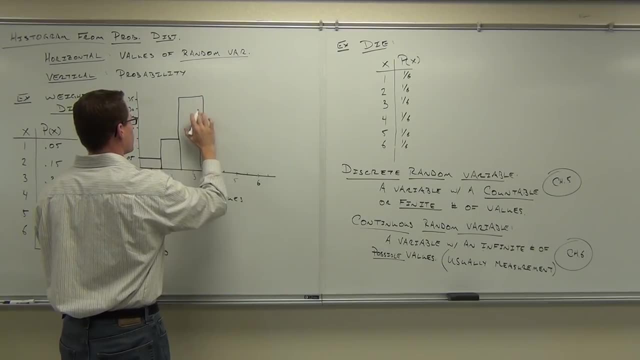 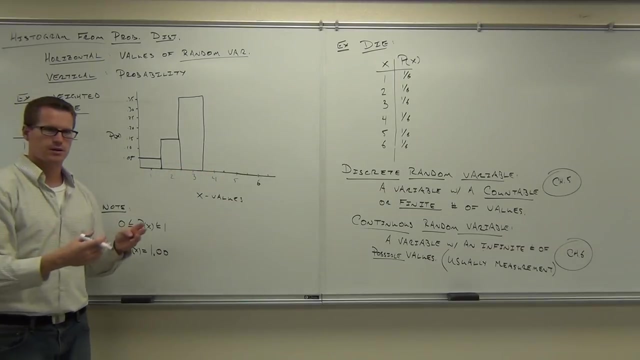 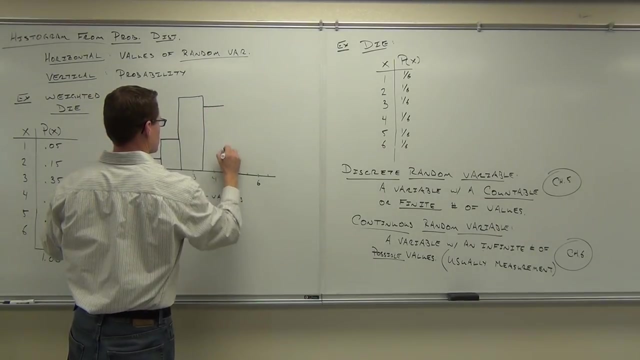 I wish I could draw straight. That's horrible. By the way, these all do need to be the same width just to make sure that we have a valid, unbiased histogram. Four is at .3,, so that's down a little bit. 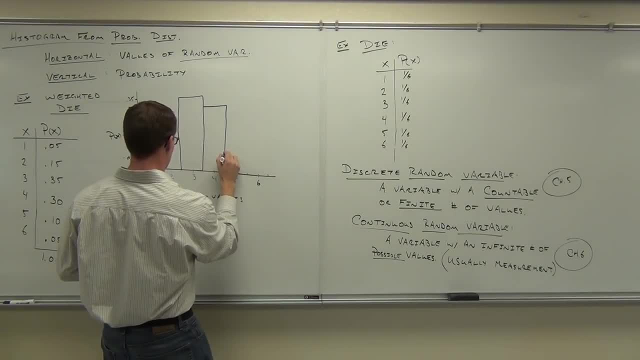 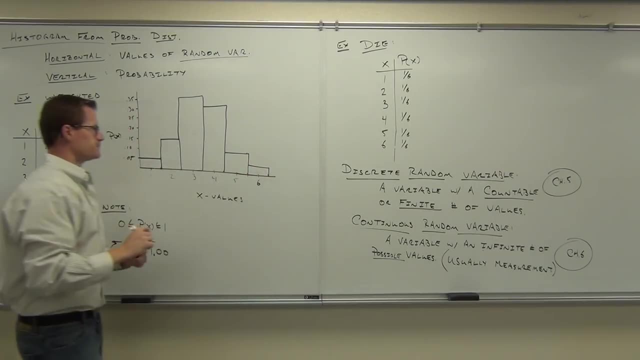 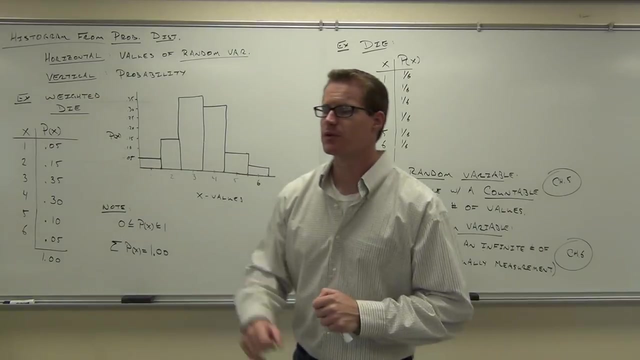 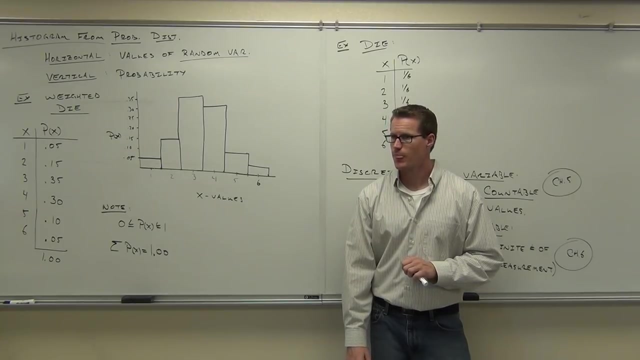 Five. we drop any further, Even further here to .1.. Does this give you a good picture of what should happen? What value should I be rolling? most often? Page four, Page four. typically that's what should happen. Am I ever going to roll ones and sixes? 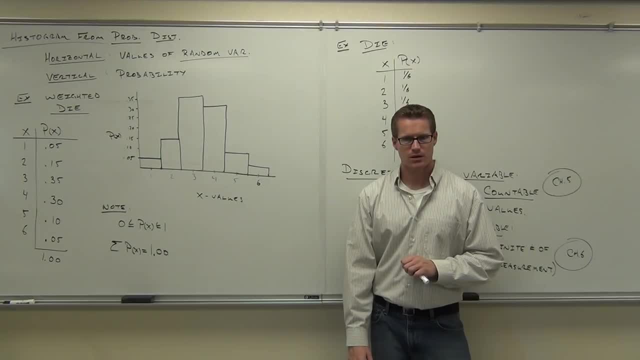 Am I ever going to roll those? Is there a probability? Then you can't say no, Because if there was no probability, then you'd have what You'd have: zero. So am I ever going to roll ones and sixes? Absolutely. 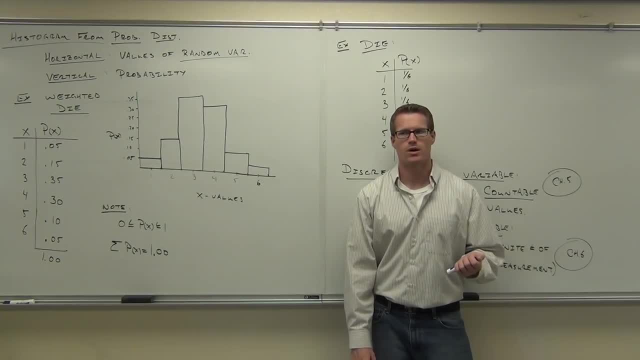 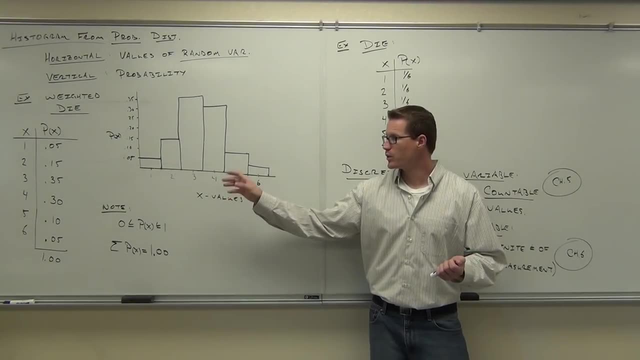 Is it rare? We haven't really talked about rareness as far as probability goes. We will at the end of class, So we can't say whether it's rare or not right now. We will in a little bit, But will you roll all these numbers? Yes, Is there a different chance of rolling certain numbers than others? Absolutely Most often you should be rolling threes and fours And then after that twos, Then fives And then ones and sixes are equally spread, But you'll get all of them at some points. 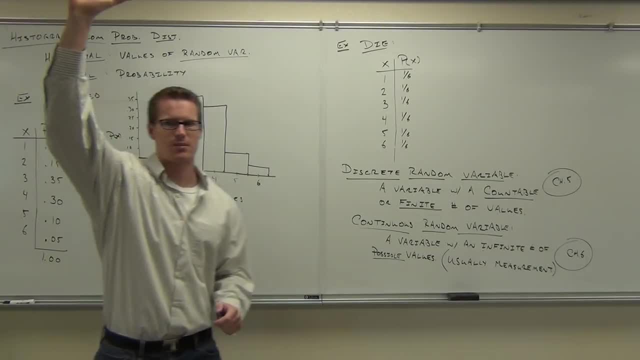 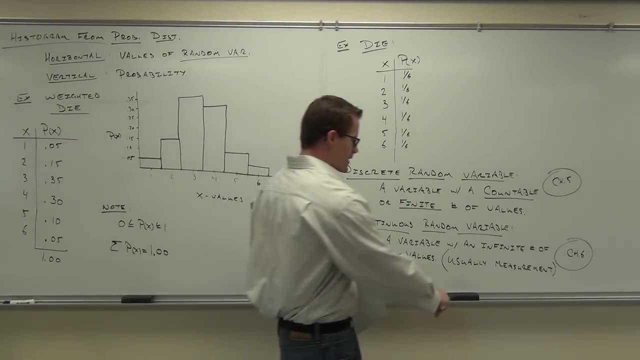 Just, most of them should be threes and fours. How many of you feel okay with making up this histogram? All right, Good, good, You know. what's interesting is that not only can we make a histogram out of our probability distribution, we can also find the mean and the standard deviation for this data. 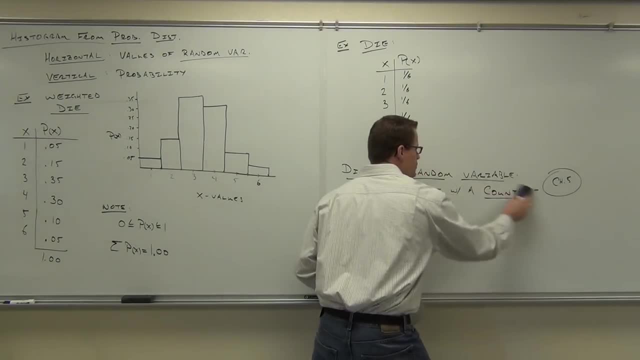 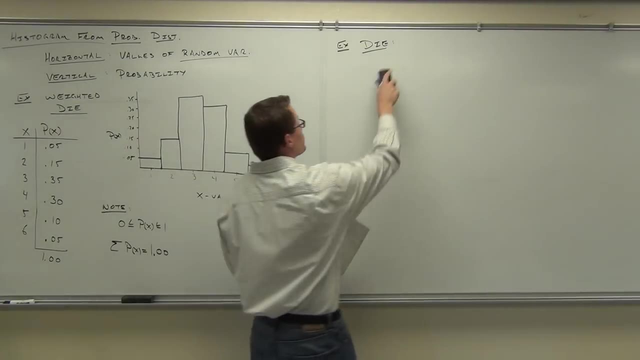 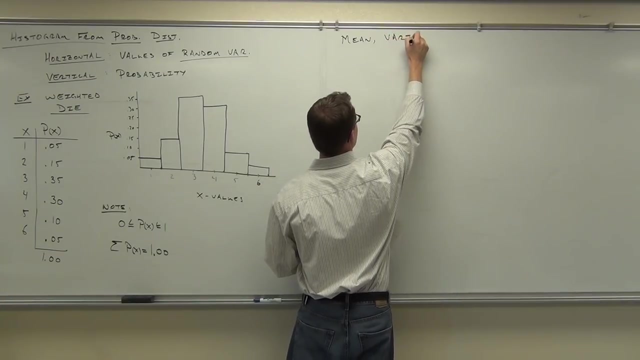 So we'll talk right now about how to find the mean from a probability distribution. I'm going to draw some parallels from a frequency distribution, So this should be kind of nice for us. So let's discuss mean variance and finally, standard deviation. 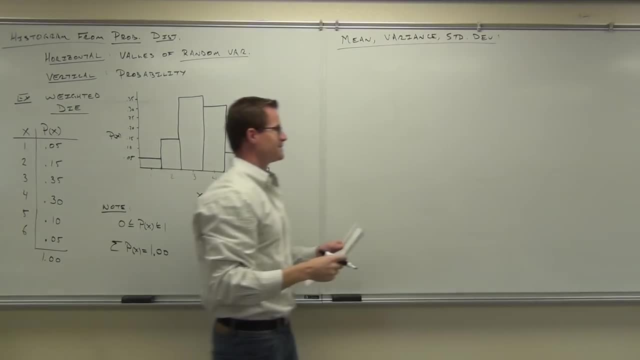 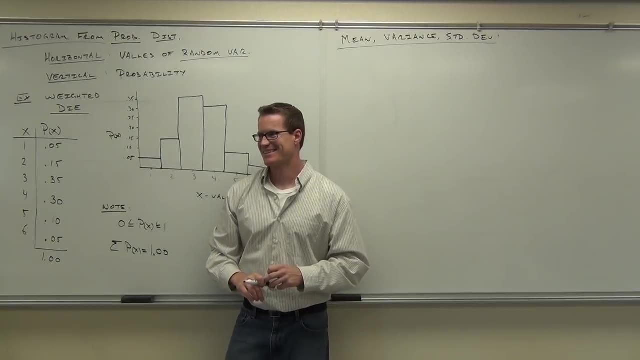 Oh yeah, You didn't know we were getting back into standard deviation, did you? You didn't know you were going to have an exciting day when you came into stats class? Uh-uh, You're like: ah, more probability maybe. 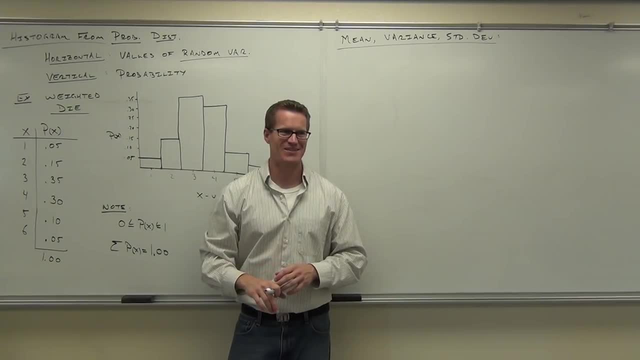 Probably some distributions, But you didn't know about variance and standard deviation. Aren't you glad you came here today? Is this a good day for you? I think it's a good day for you. Let's start with the mean, because we know. 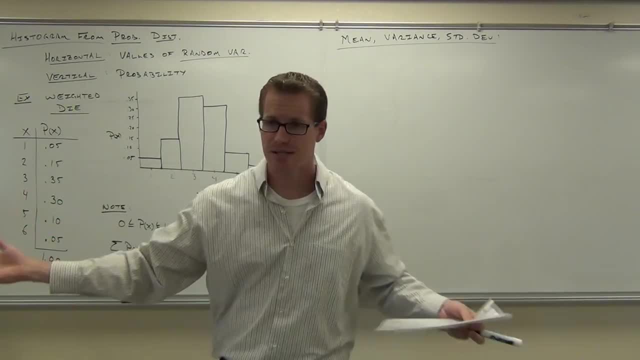 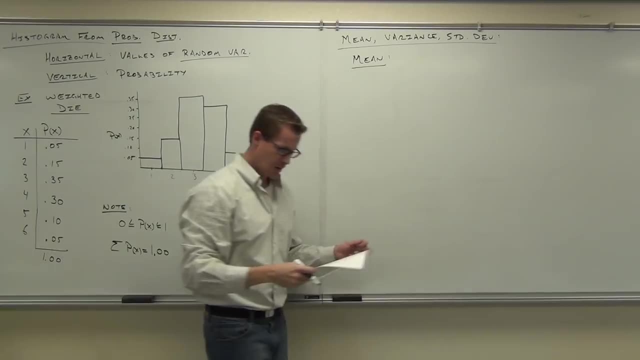 that we're probably going to have to take the mean to find our standard deviation. It's what we did last time when we first introduced this stuff. So how about the mean? The way I'm going to do this is I'm going to draw this from the mean of a frequency distribution. 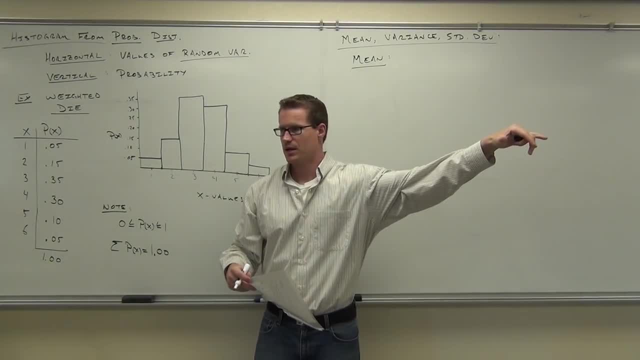 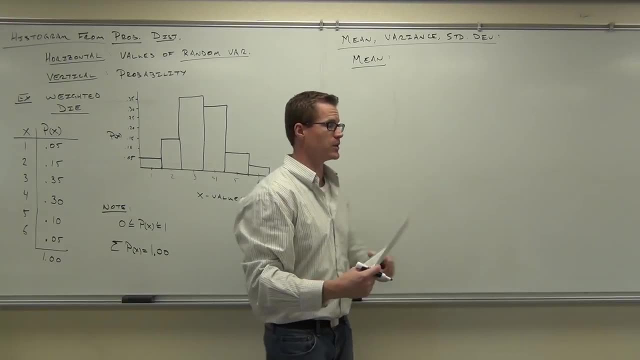 I'll play around with that thing and make it into a mean for a probability distribution. So we're going to change a frequency distribution's mean into a probability distribution mean. Here's how we're going to do it. If you remember, this is from a long time ago. 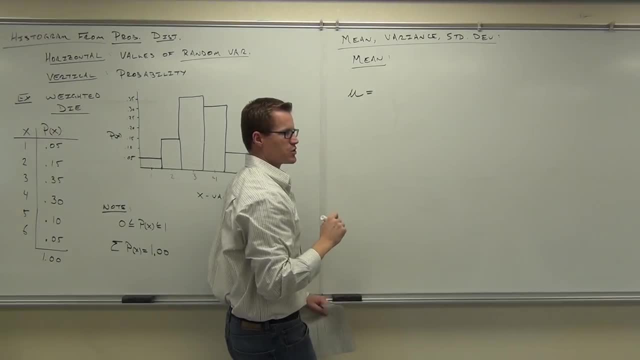 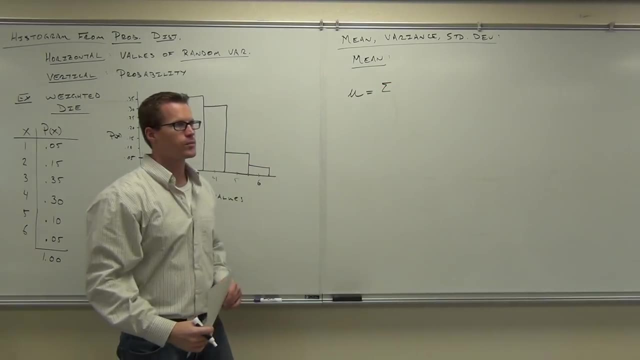 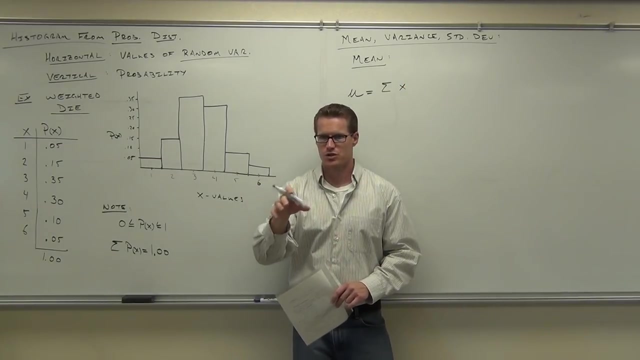 but the mean of a frequency distribution was this: You added up every value but for- if you don't remember this, go back and watch the video- but for a frequency distribution, the x value was actually the midpoint of your class. Do you remember that? 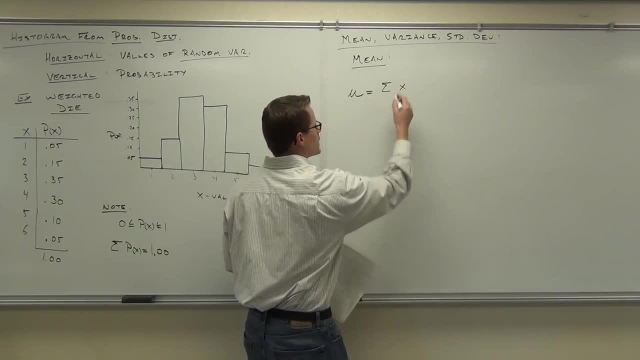 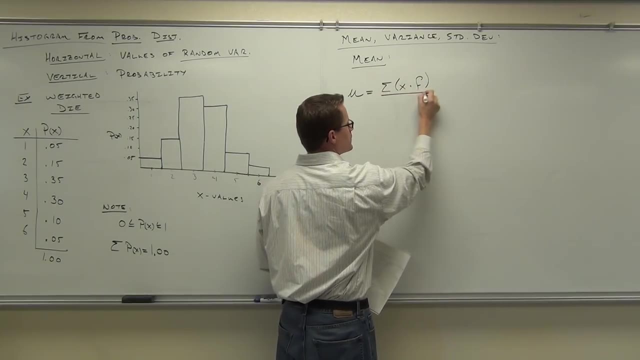 That was the midpoint. We had x. This was the midpoint times, the frequency for each class. This was the midpoint times, the frequency for each class, and then we divide by the total number of items in our sample or in our population, in this case. 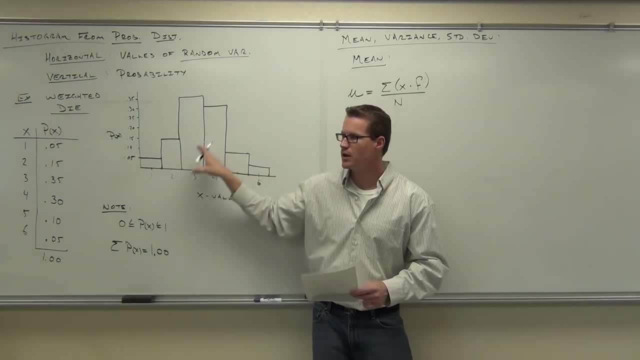 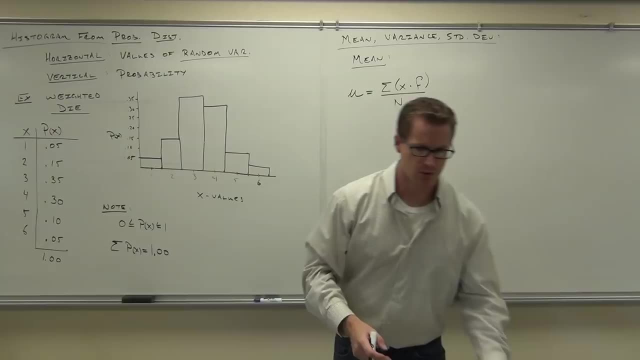 It would be a population. I'm using population because we're dealing with a finite or countable number of items, so we're dealing with the whole thing, So we're only going to die. That would be a population-based probability. there, The only thing you can get out of it is 1 through 6, right? 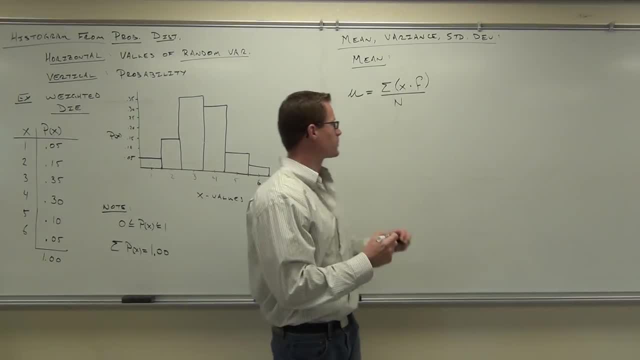 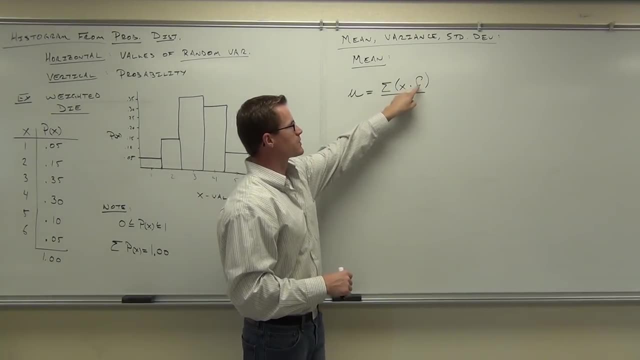 You can't get anything else. We want to make sure this to be a population here. So for a population's frequency distribution we're going to find the mean of that. We take the midpoint times, the frequency, We divide everything by n. 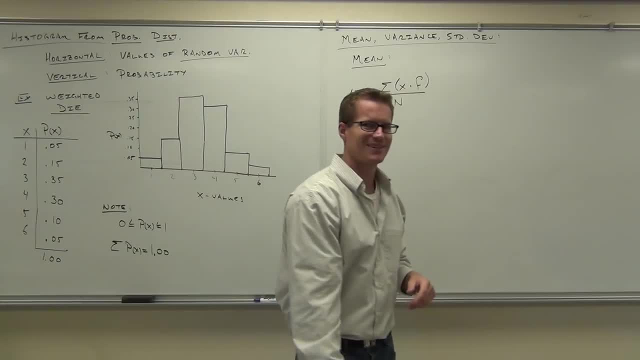 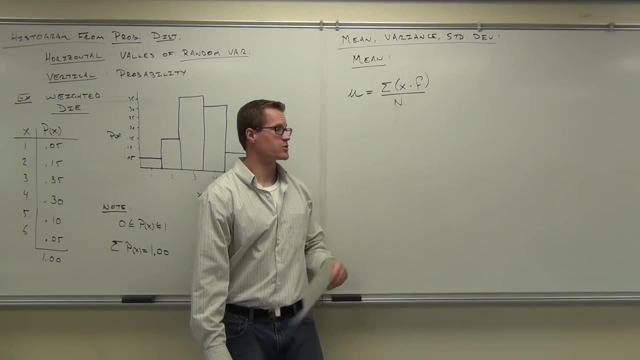 You with me on this. You guys awake today. There's only one: You better wake it up. This is important stuff we're dealing with right here. There's only one thing you're going to have to trust me on, and you have to trust me that. 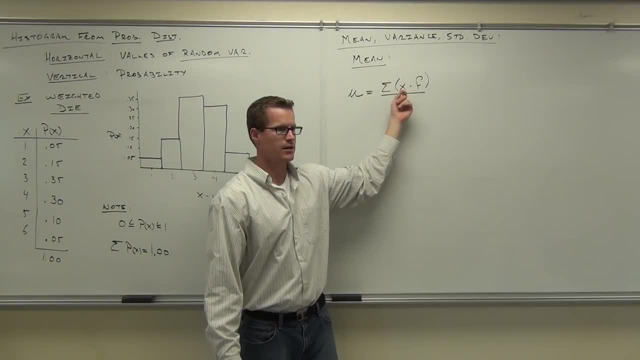 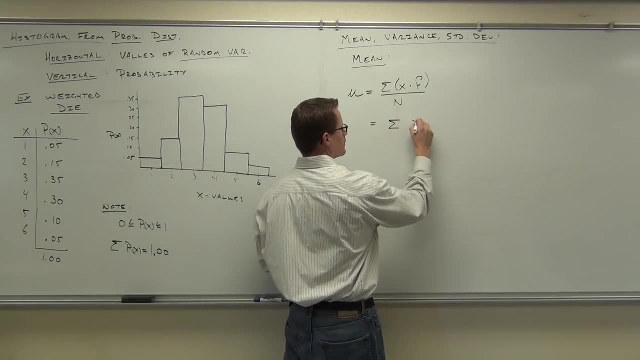 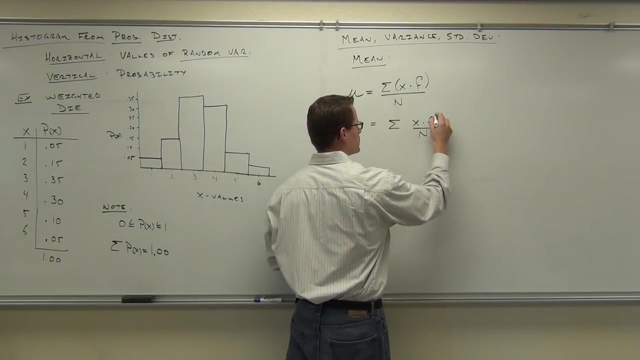 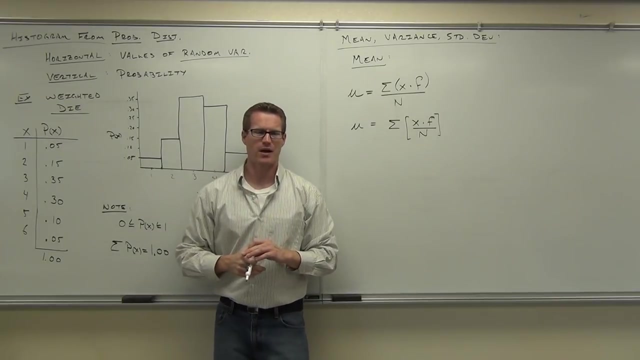 dividing a sum like this, after you've already added, is the same thing as adding up the division as you go. You're going to have to believe me on that part, Do you believe me on that part? I hope so. I'm a math teacher. 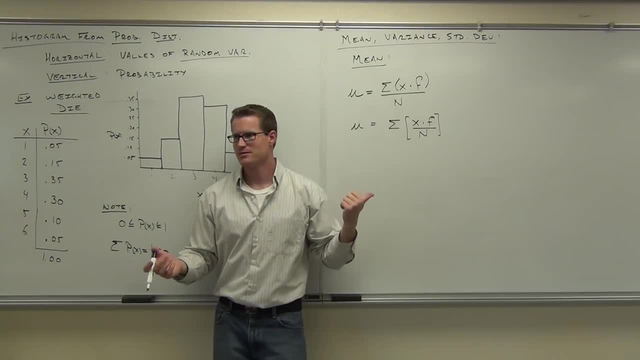 I mean, what's wrong with you? if you don't believe me, Think I'd lie to you? Yeah, I probably would lie to you, but not about that. Not about that. I can prove it to you. though, If you want to do this thing, right here. 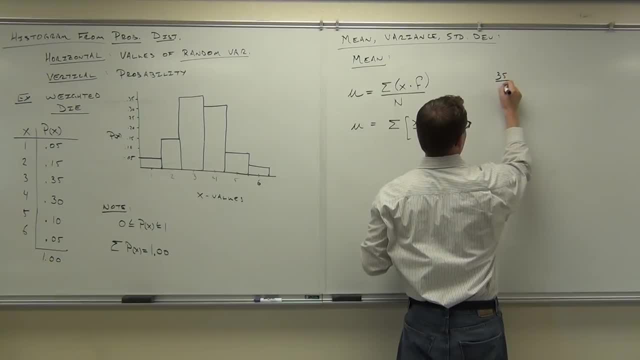 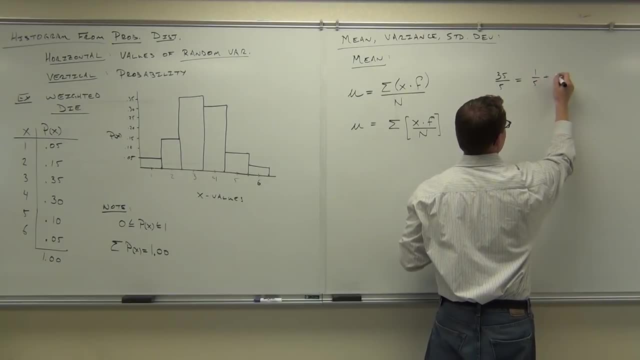 and say 35 over 5, you know it's 7, right? You could also do it this way. You could say: this is equal to 1 fifth plus 1 fifth plus, and do that 35 times. Do you believe me? 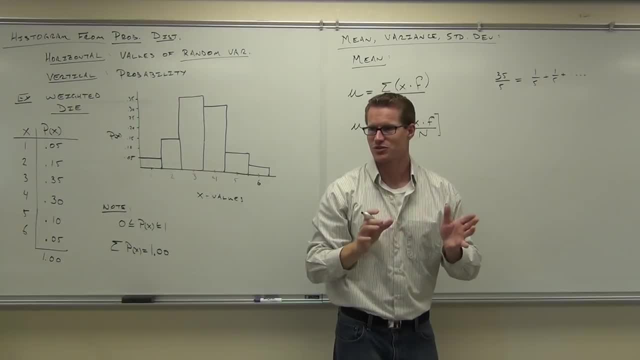 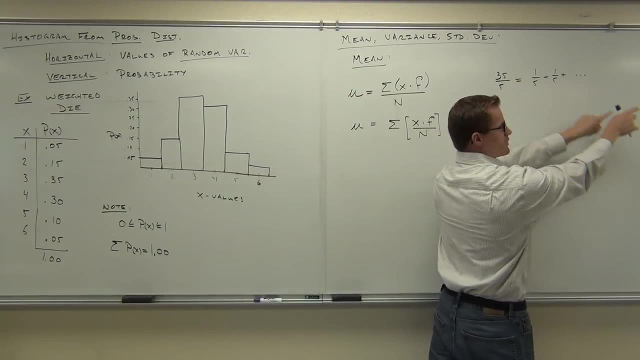 If you do that 35 times, it would add up to 35 over 5.. You know that's true, right? So I can separate something that's already added and being divided by adding each little division piece in a row. So that's a true statement. 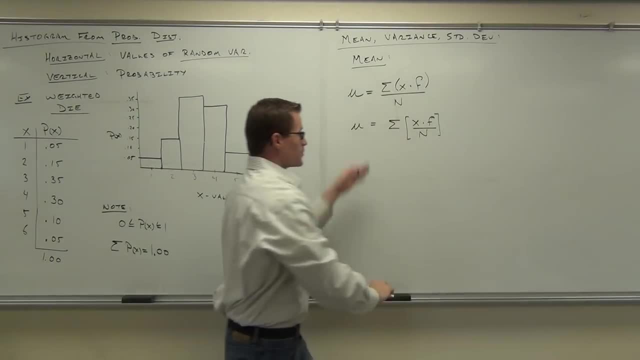 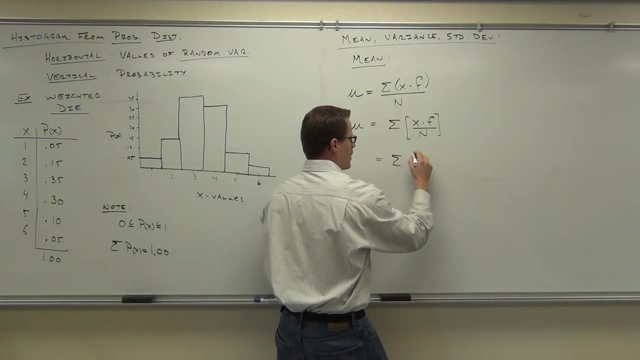 You can do it, But once we do this, this is pretty kind of obvious. what we have here- I hope you're seeing this, Check it out- This is the same thing as a sum of- I'm going to use a little fraction work here. 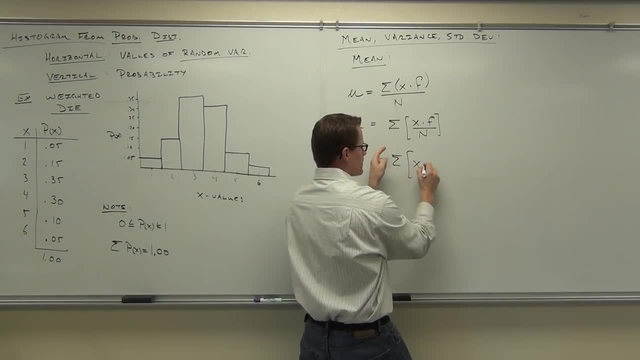 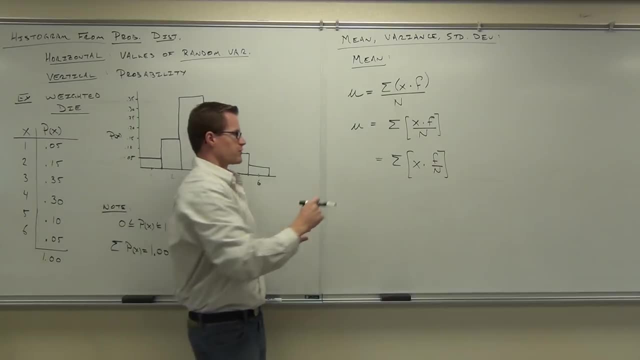 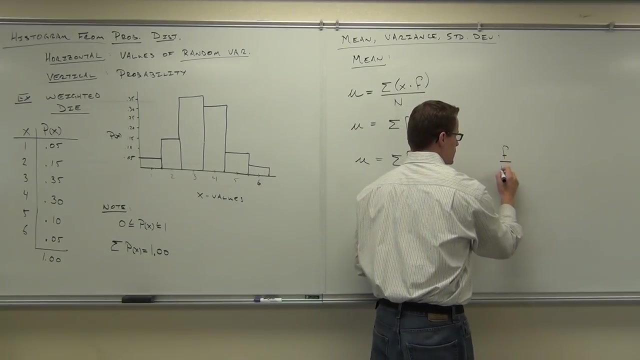 You should be able to do this on your own, though. This is the same thing as x times f over n. Do you believe that That's for sure? true, For sure, true. Well, here's the cool part. What is a frequency? 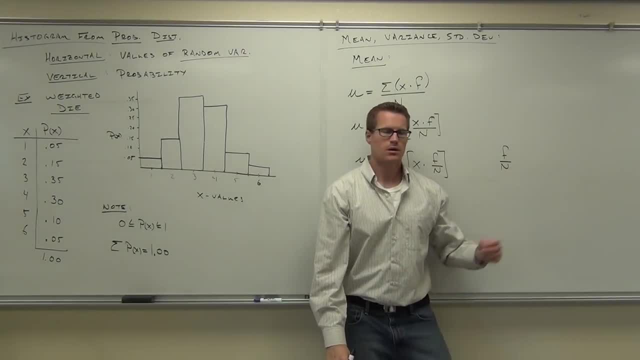 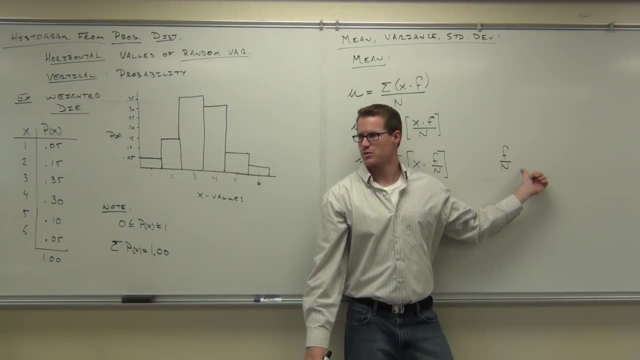 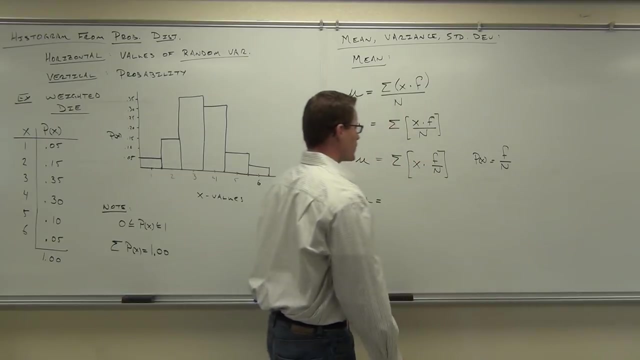 divided by the total number of items. What's a frequency divided by the total number of items? A, That's outcomes divided by total number of possible outcomes. right, That's a probability. So what we have here is the sum of x times p of x. 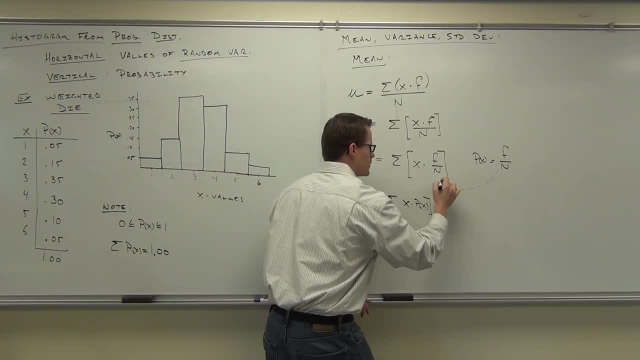 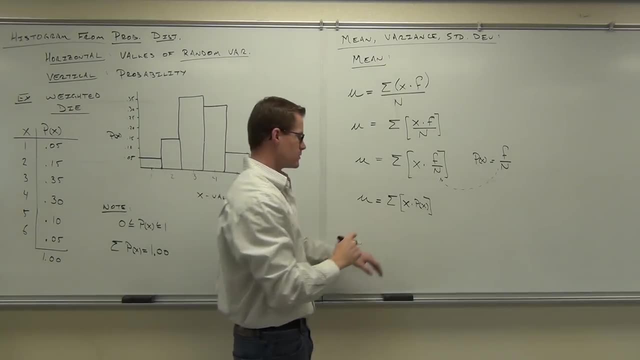 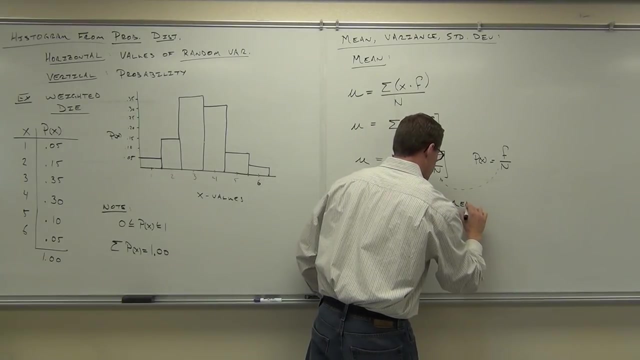 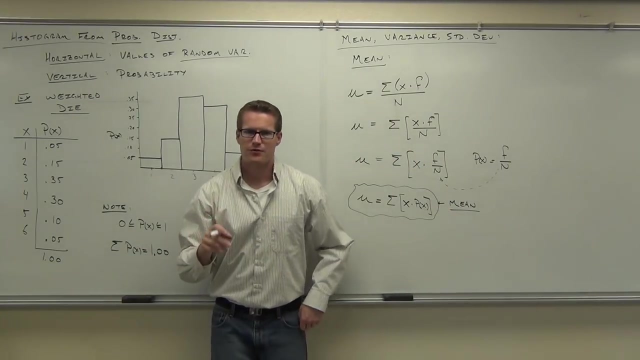 by a little substitution. This expression right here, this equation: that's your mean. Also, there's another expression for mean that you need to know If you're ever asked for expected value. expected value is the mean. It means this: 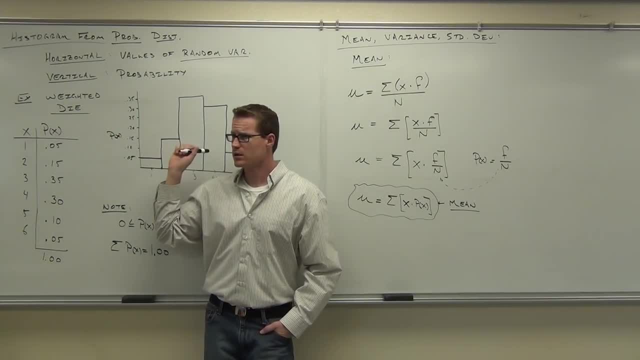 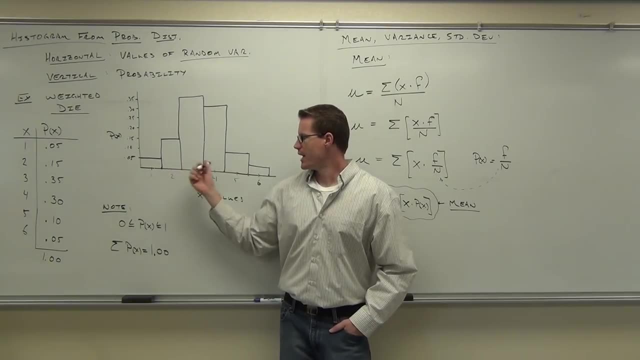 What's the average you should get? You should get somewhere between three and four. right, Are you with me guys? What should you get out of this thing? The average you should get is around a three or a four. That's somewhere in there. 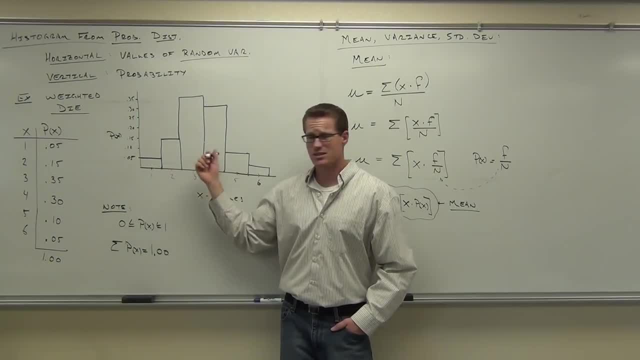 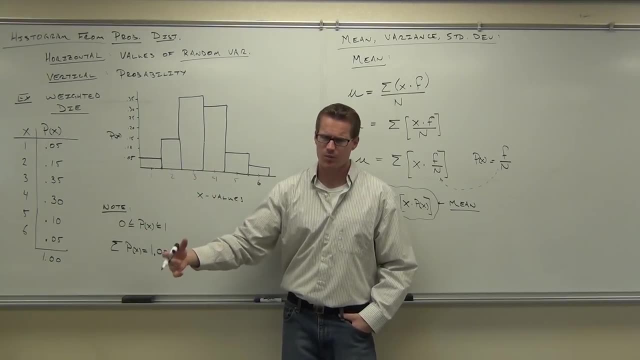 That's average. What are you expected to get? You're expected to get somewhere around a three or a four. This is telling you what should probably happen here. You should probably be getting probably probability right. should probably be getting somewhere around a three or a four. 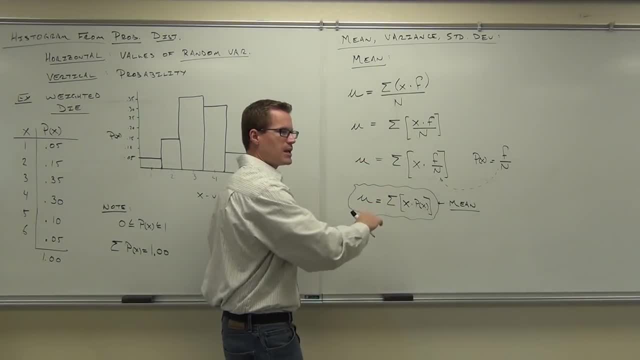 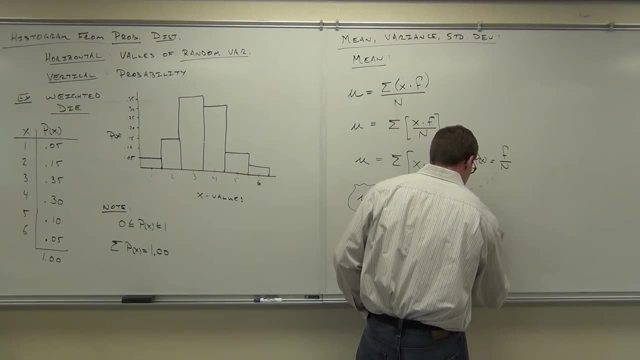 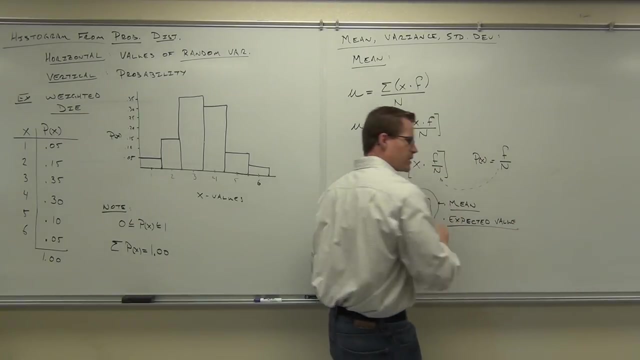 That's also known as the expected value. So mean and expected value are synonymous. So when you get down to your homework, and it's well, we never talked about expected value, Yeah we have. It's the mean. It's the same exact thing. 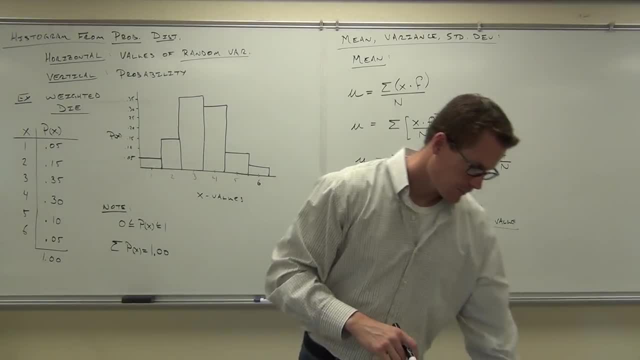 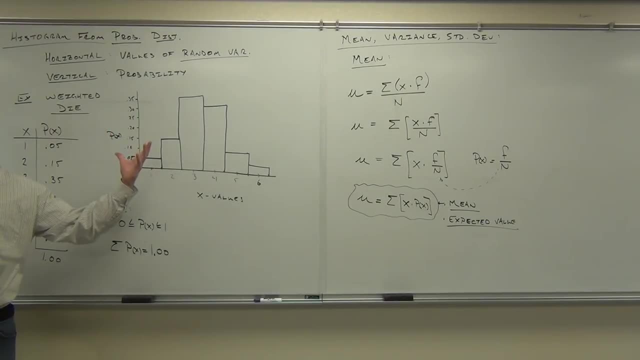 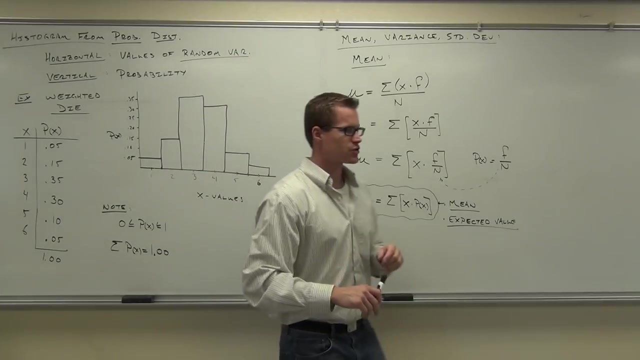 So mean or expected value. Okay, what do you say? we do this with our diet. You ready to do that? See what this, if this comes out the way we hoped it does. Do you guys have any questions on the histogram part? 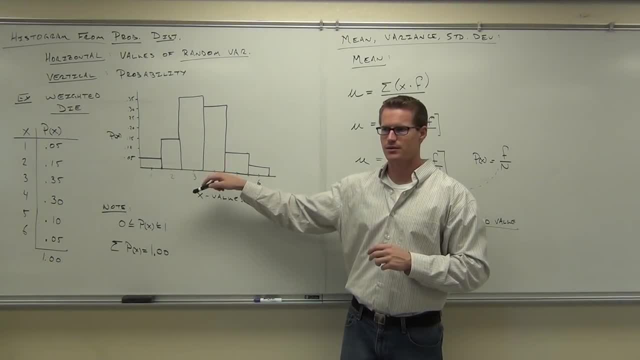 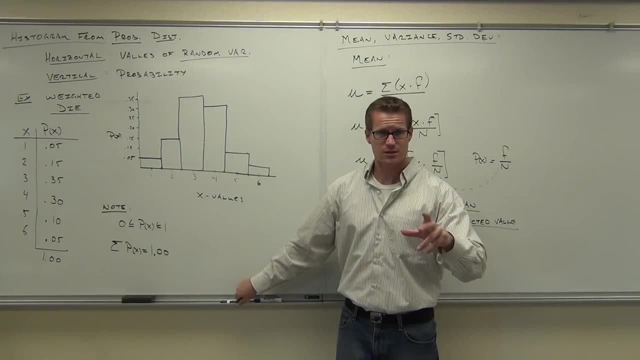 Because I need to erase that to do our probability math. Okay, so so far we've learned about random variables. We know the difference between continuous and discrete. yes, What are we dealing with in this chapter? So, countable or finite? 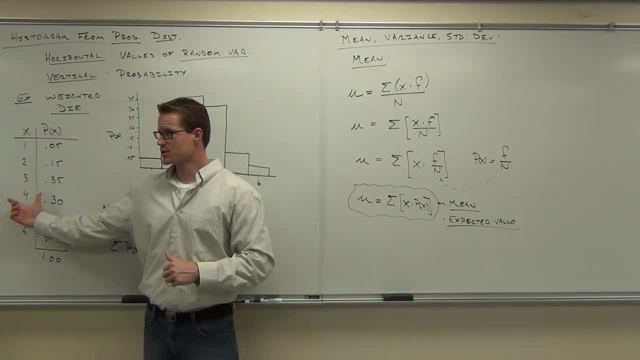 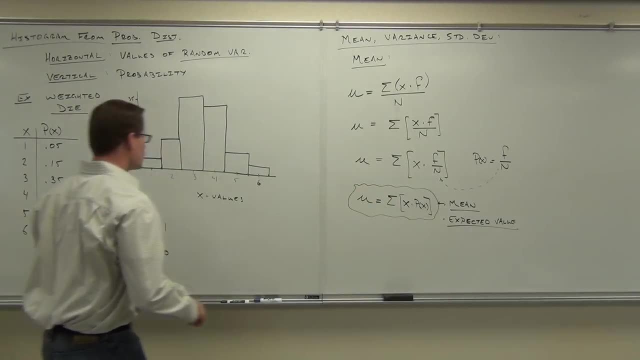 We know what our probability distribution is. It's really similar to frequency, right? We just have our values and the probability for each one. We know we can make histograms out of that And I've just developed the mean for us. Let's see if we can find the mean. 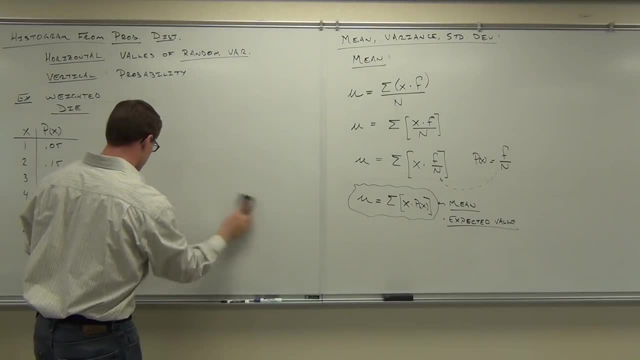 of my weighted diet example. Also, we know every probability of course has got to be between zero and one, And if we add all of them up for our distribution it has to equal exactly one. Okay, So our sum of p of x times x. 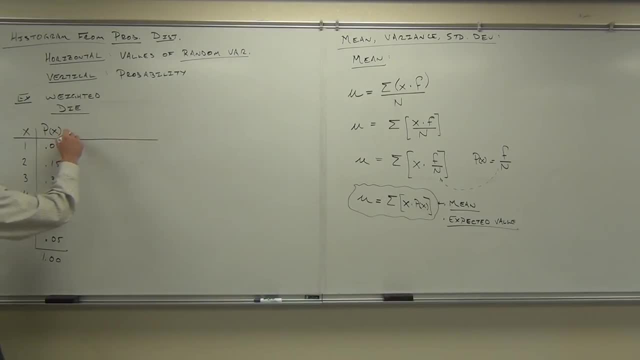 We add all that up. That is our mean, So let's do this together. The first thing we need to make up is a column for x times p of x, Because that's what this says. It says you're going to multiply them. 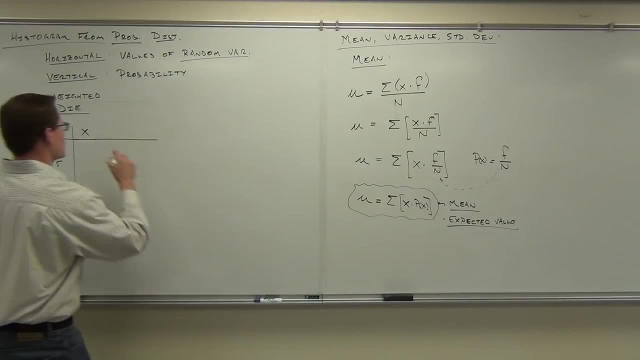 and then you're going to add them all And that, right, there is your mean, No extra work. So find x times p of x. Let's do that together. I'll take care of the first one, okay? First one is .05.. 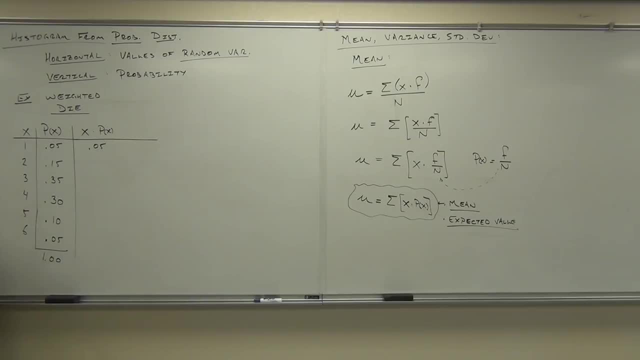 Now I did all the hard work. Go ahead and do the rest of them. That was funny. Use your calculator if you have two. 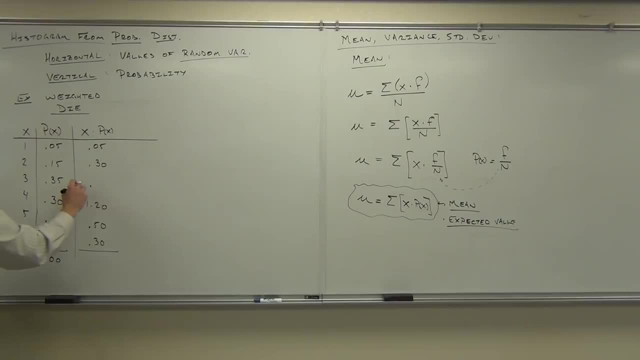 It can't be between zero and one, Or it can't. I'm sorry. it has to be between zero and one. 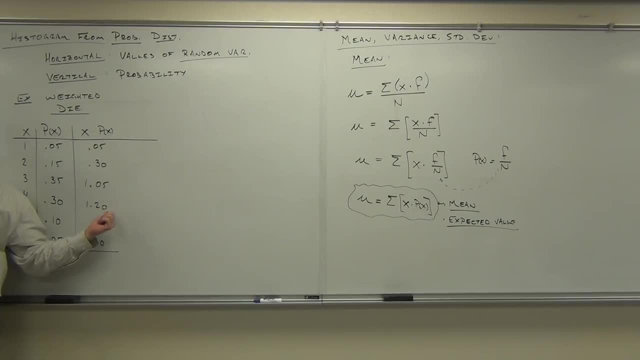 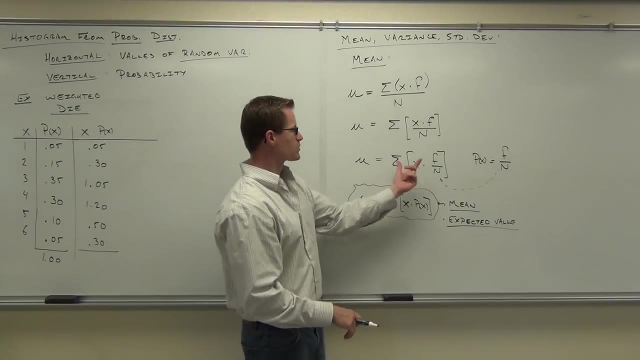 What about that one? and what about that one? Are we dealing with the same situation here? These aren't probabilities anymore. We're multiplying a value times a probability. What this is giving us is what we had here when we did our frequency distribution mean. 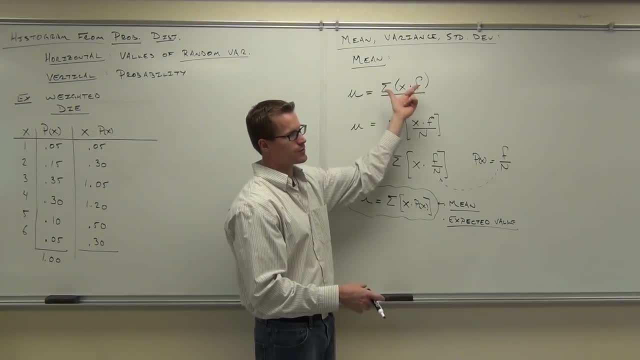 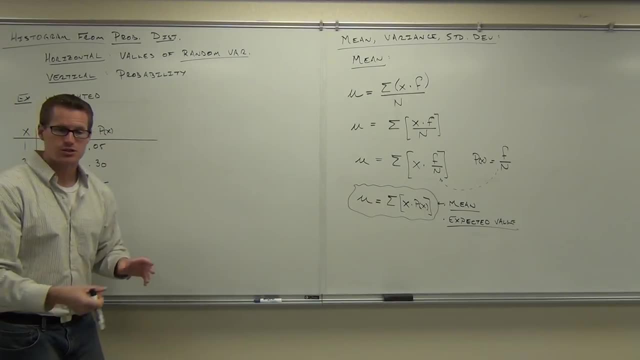 before we add them all up. Actually we did that. we multiplied first and then divided. Look here we're multiplying. we're just getting our value times our probability. If we add all these things up, that's gonna give us our mean. 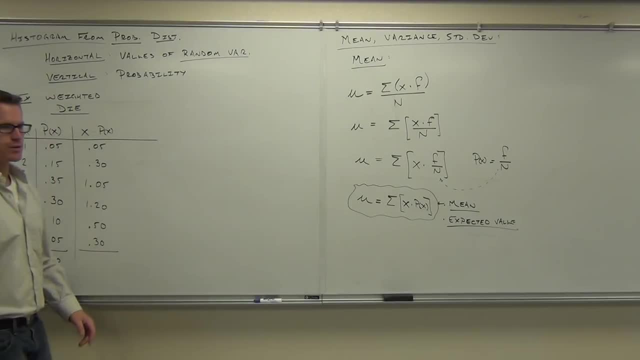 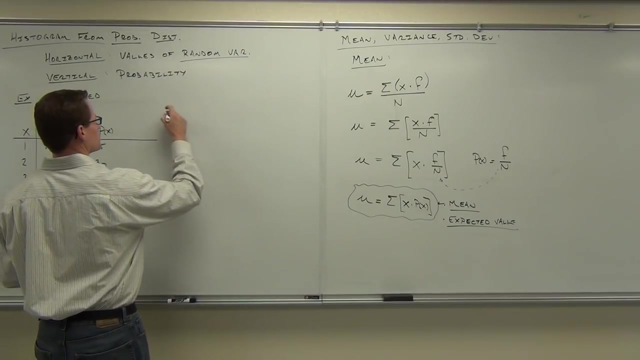 So the next thing you gotta do: add those. Do that for me on your own, add those real quick. Add that column So this would give you the sum of x times p of x, 3.4?, 3.4?. 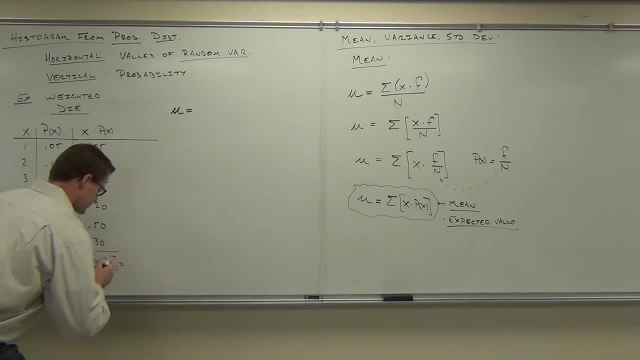 Well, that's actually kinda painless, because as soon as we're done with this shoot, hey, x times p of x, we add them all together. X times p of x, we add them all together. That is your mean. 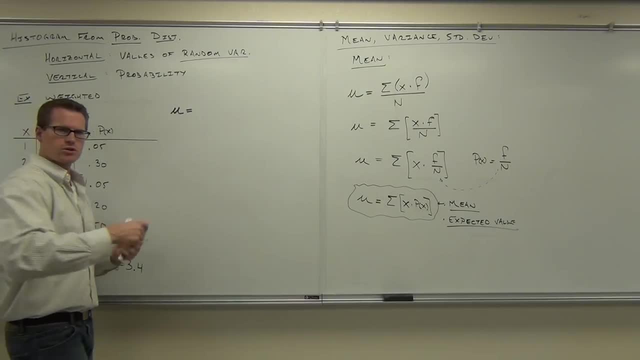 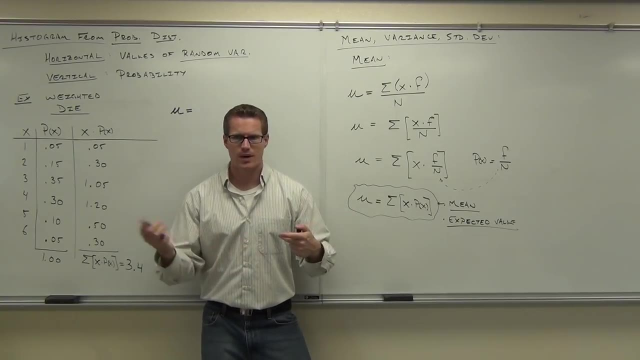 So our mean is, what's our mean here? No extra work, no other dividing. We already took care of the dividing. Look what you're doing. okay, When you're dealing with a mean, you know the average is you add everything up and you divide by the number you just added. 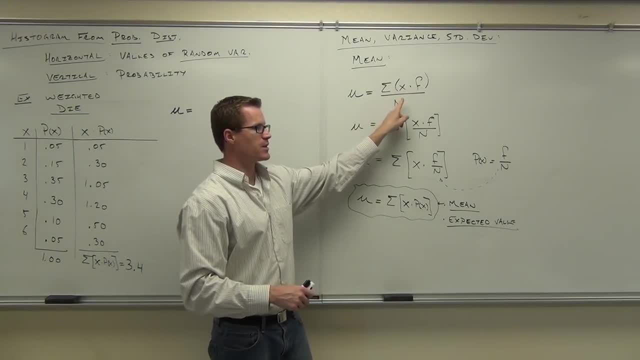 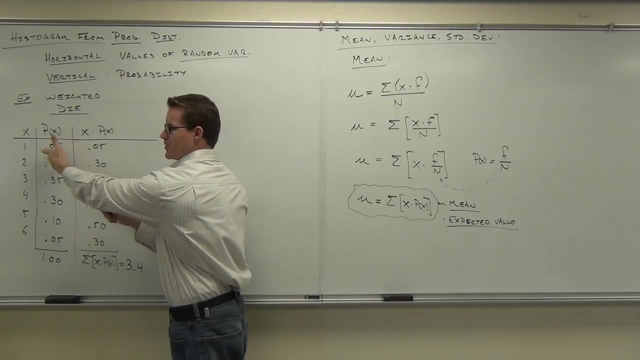 What you're doing here is you're adding everything up and dividing by the number you added. except we're dividing as we're going here. The probability is really, since it's a decimal, it's like you're dividing as you're going. that's fine. 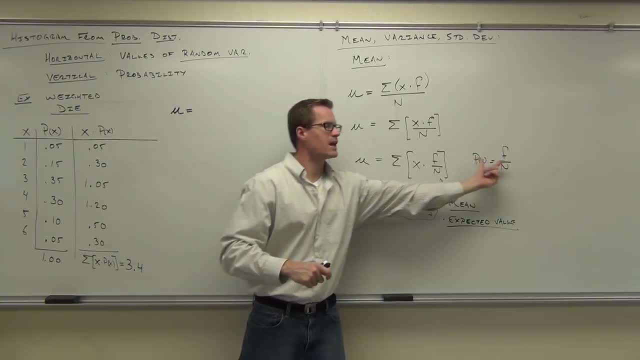 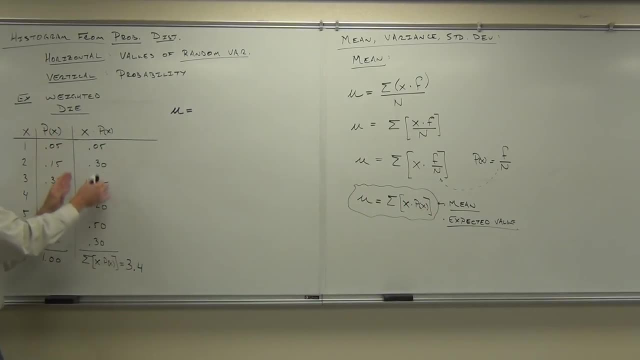 We're just doing that here. We're taking that probability. the probability is already the division. That's what that is. You're just dividing as you go, So we don't have to do any more dividing. You've already done that piece by piece. 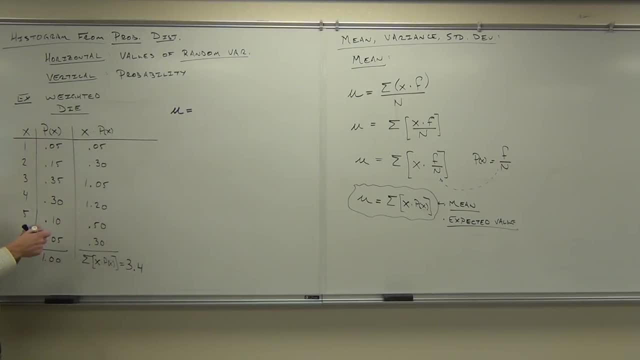 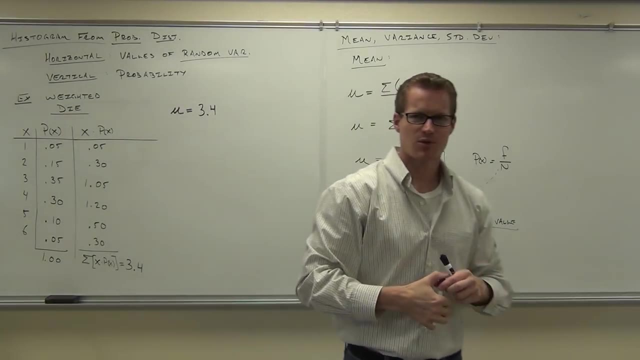 You just add them all up and that is your mean. So your mean in this case is 3.4.. Wait a second, wait a second. That can't be right, can it? Can you get a 3.4 on a die? 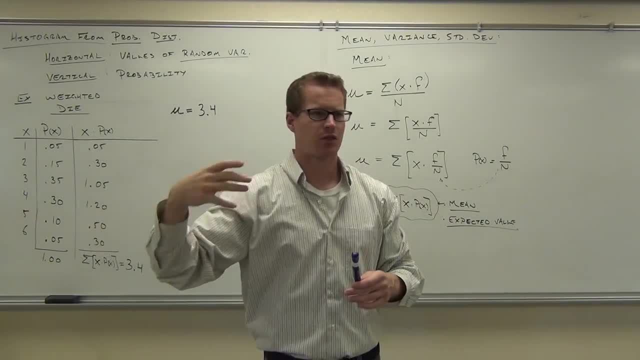 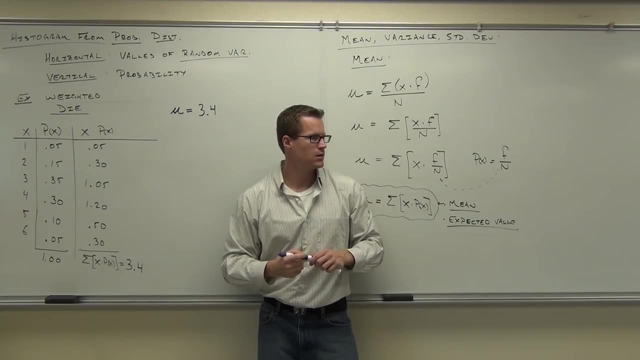 But this is what we're talking about. right is a die. What's it mean? that we get a 3.4 as our mean, as our average, A little bit more of a chance of a 3 than a 4.. 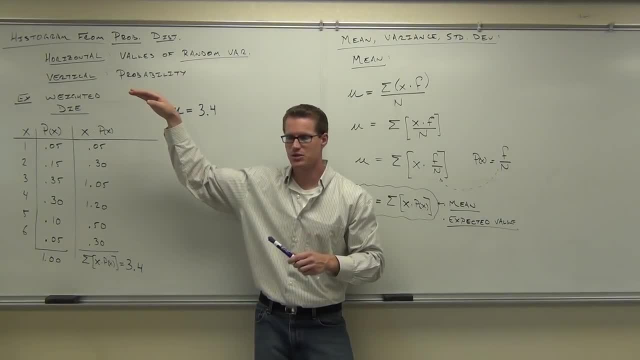 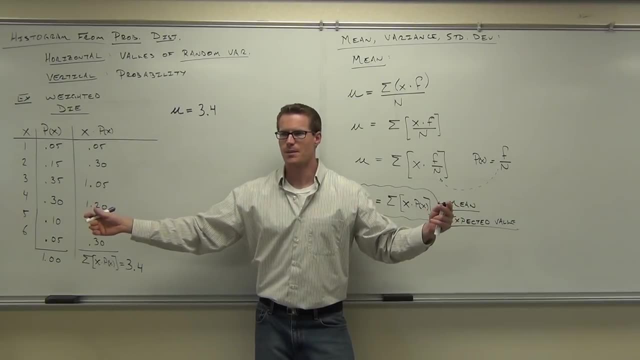 If you remember from your probability distribution I just had up here, 3 was a taller column right, But just by a little bit. What the 3.4 says is that on average over the long run, you roll this a billion times and you average those results. 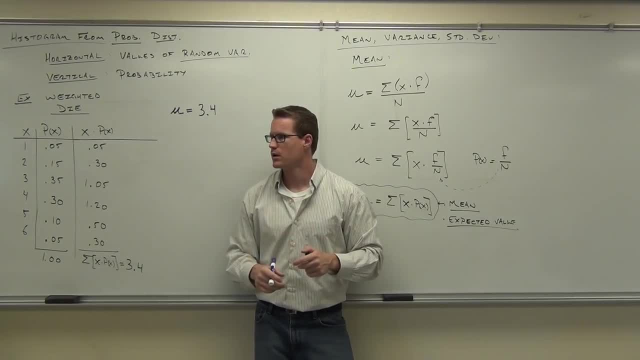 those results will not be a 3 or a 4, it'll be a 3.4.. If you average a couple of numbers, you don't have to necessarily get the number on the die right. You can get a number between there. 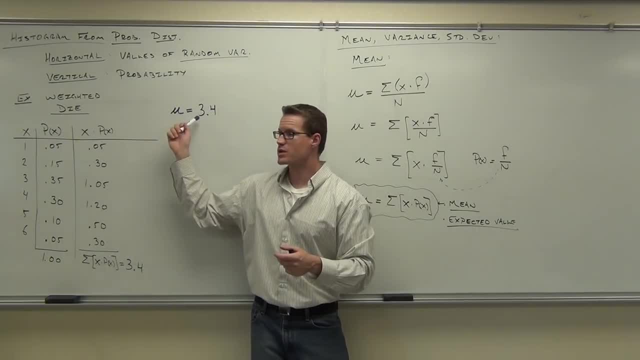 and that's what we're talking about here. What this says to you is that we're most likely going to get 3s and 4s again. That's what it says- More 3s than 4s, just like your probability distribution said. 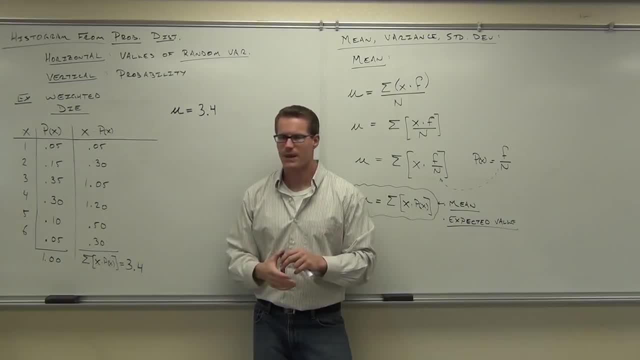 but that is what we're expected: to get somewhere around a 3 or a 4.. How many people understand the idea of a mean Good? Now we do have the variance idea too. We'll talk about variance, Of course. we know variance and standard deviation. 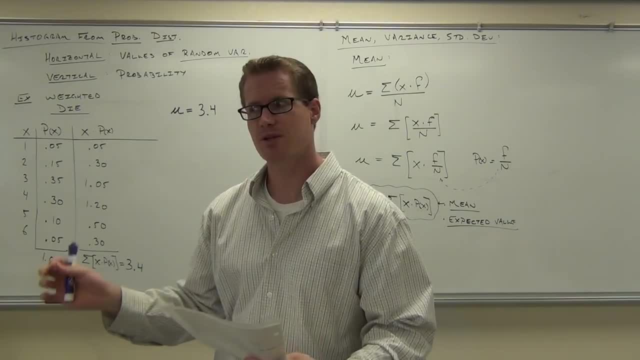 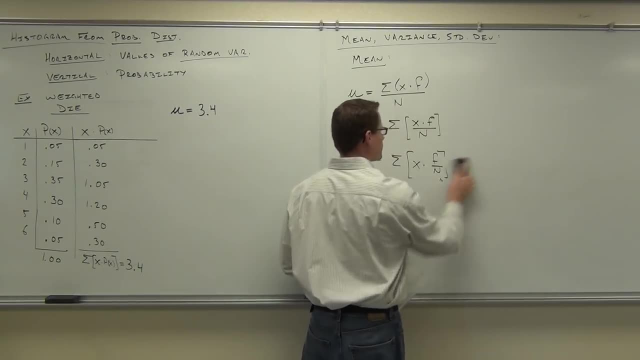 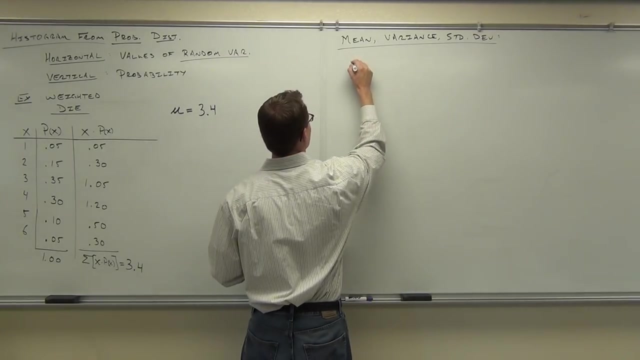 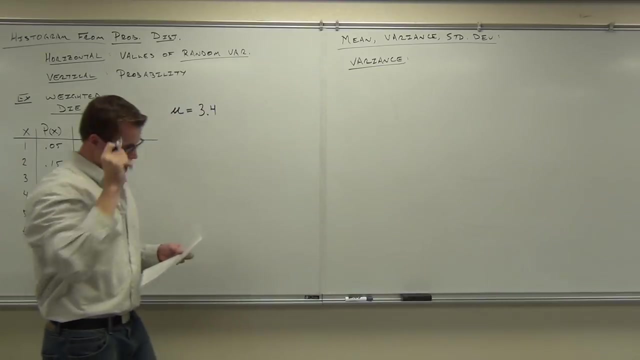 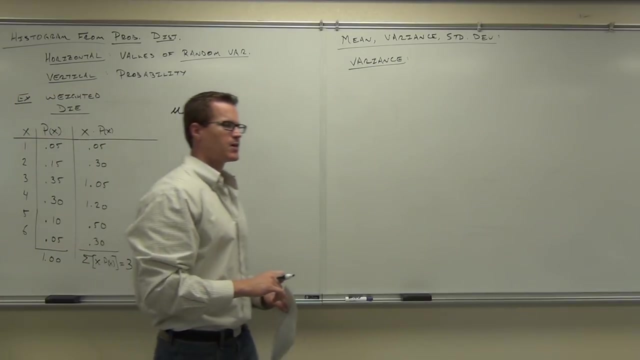 they're very closely linked together, right? So if we find the variance, we pretty much automatically have the standard deviation. Let's look at the variance and then we'll be done after that today. Hey, by the way, we're talking about variance, I know. 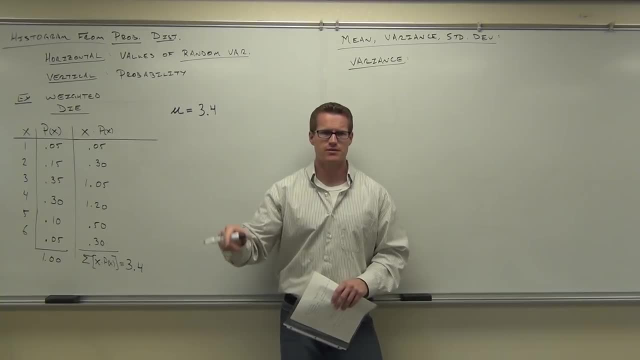 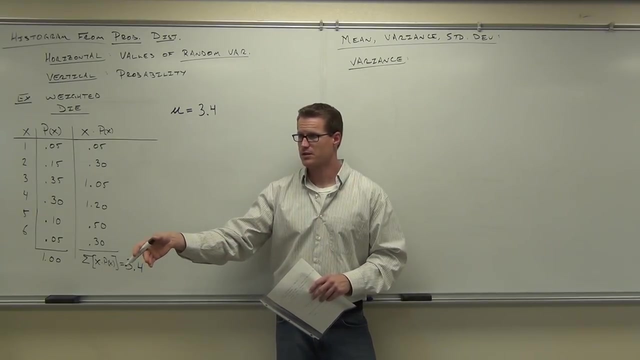 but I want to reinforce the standard deviation idea. What does standard deviation tell you? Oh, kind of A z-score would tell you the number of standard deviations away from the mean. We're not there yet. We're not at a z-score. 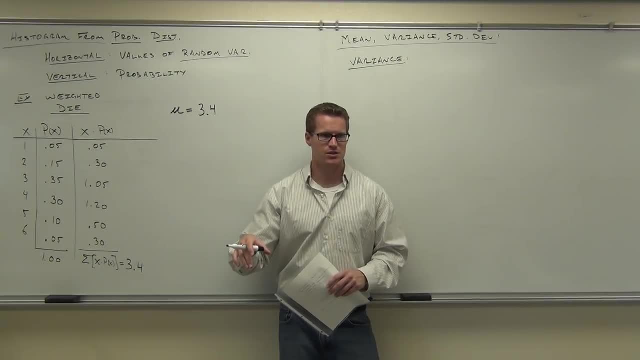 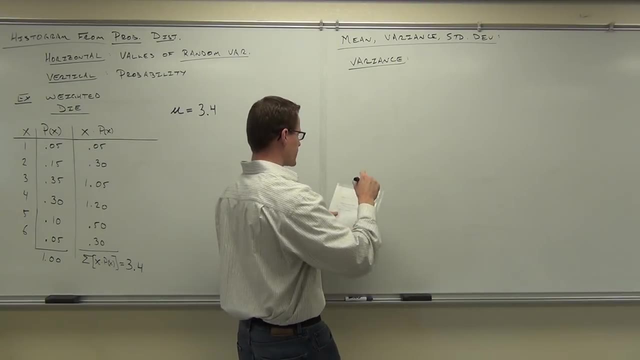 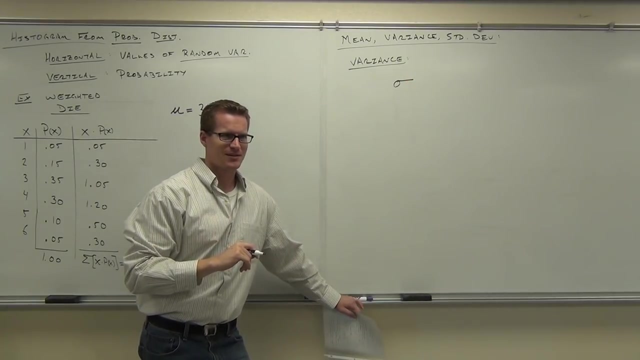 We're talking about standard deviation. Standard deviation gives you the average distance from the mean, the average deviation from the mean. We get that from a variance. Remember that symbol. What's that symbol? Little cannon thing? Pew, pew, pew. 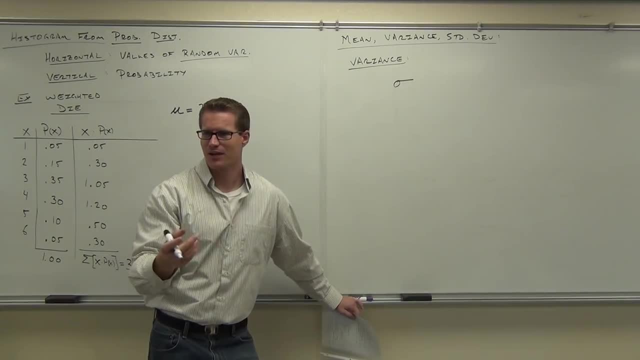 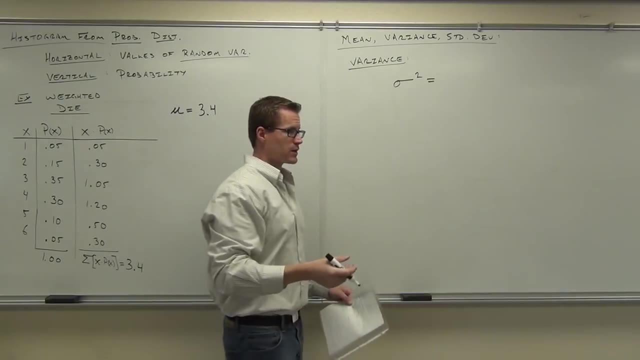 Sigma, Sigma, yeah, very good, Sigma or little cannon thing, we're going to go with sigma. Yeah, this is lowercase sigma For variance. we had squared. That was the symbol for variance. Here's what variance says to do. 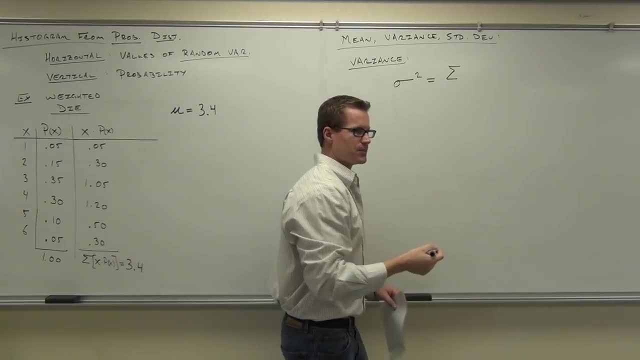 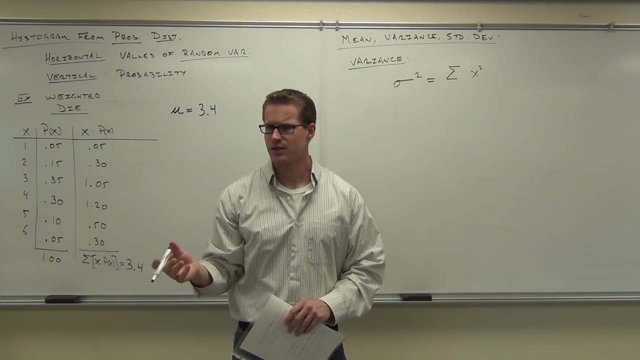 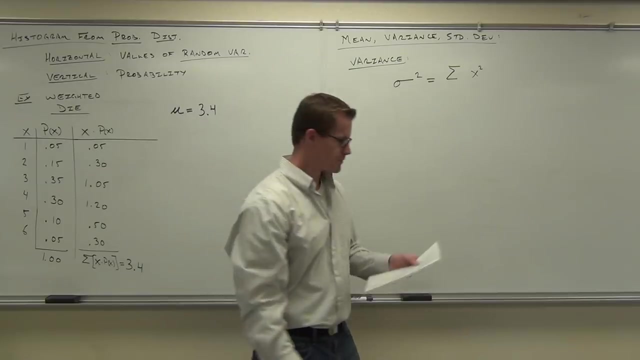 It says you add together the square of your x's. Remember the square for the variance and standard deviation. That should be coming back to you, right? It should look familiar. Go back and look at that in your notes when you get home, or something. 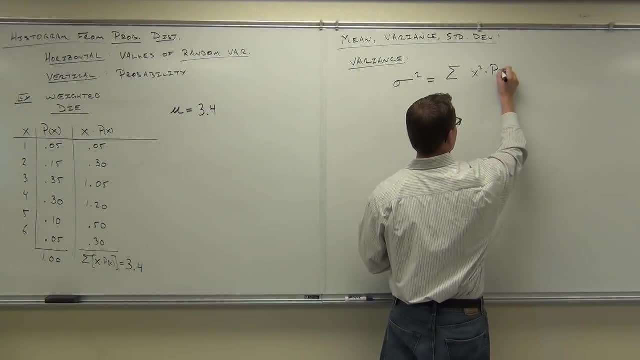 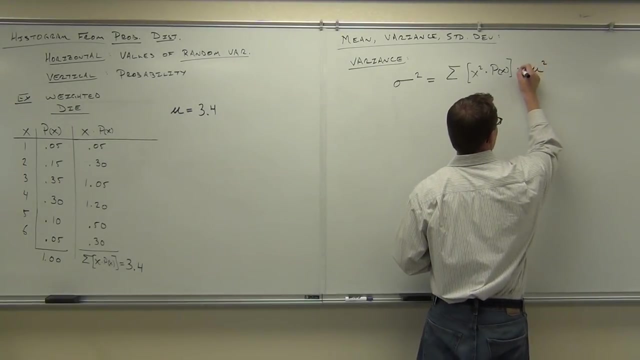 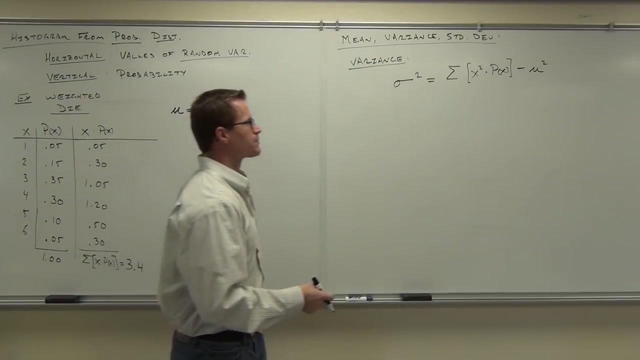 Instead of any frequency, we have probability, And then to find the distance from our mean, we have to subtract the mean. We're just going to do the mean squared, though. subtract the mean squared, That's our formula for the variance. 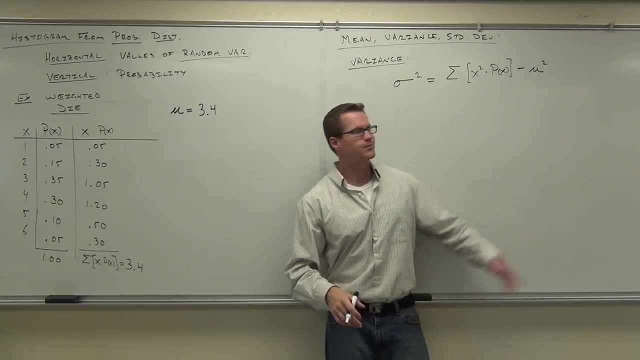 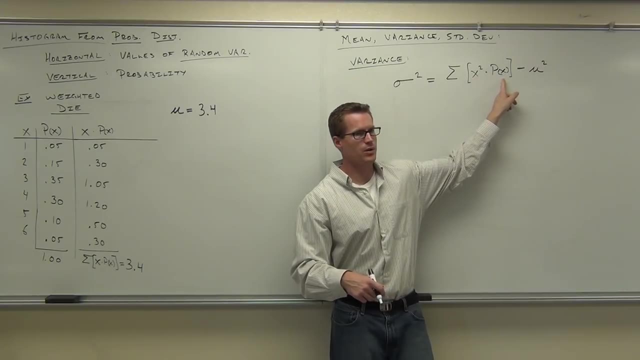 It says: first off, use your order of operations. What do you do? first, You're going to square some x's. You're going to square your x column Next up, you're going to multiply those values that you just got times your probability. 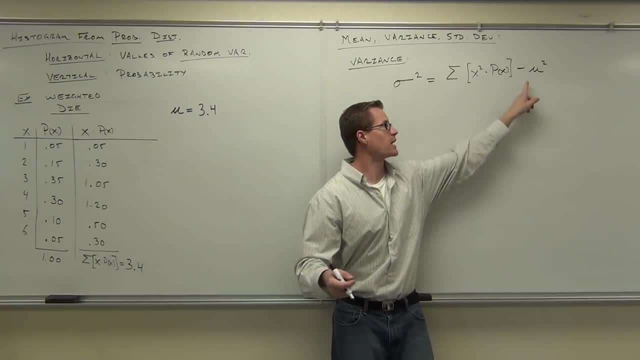 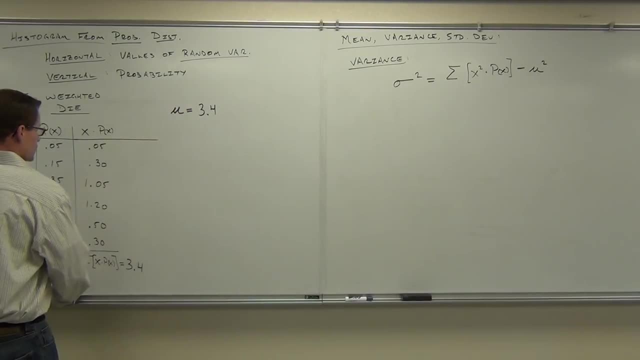 Then you're going to add it up At the very end. you're going to subtract the mean. squared You with me on this? Let's try that. We've got a couple minutes. Let's do this on our way to die. 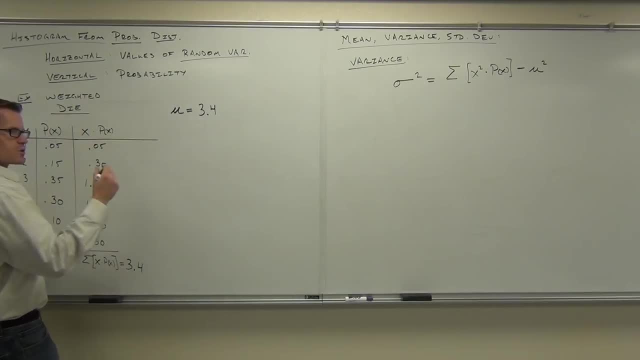 So we already have our mean. We're going to have to draw a couple extra columns here. I'm going to add on to this because you're going to be doing this on your homework and I hope you see that this is a lot easier. 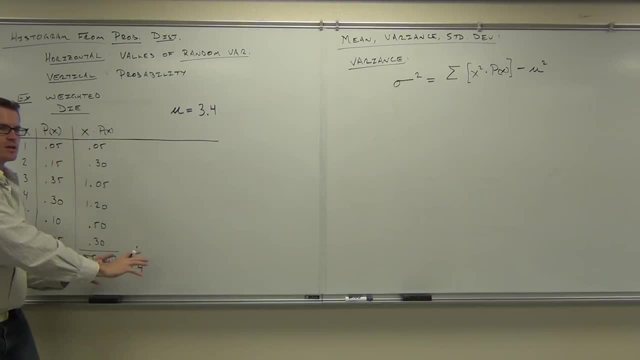 The first thing you do: you're going to find your mean right. Do you see that you need your mean in that problem? You find your mean. The next thing you're going to do: make yourself calm. you're going to have to find your x. 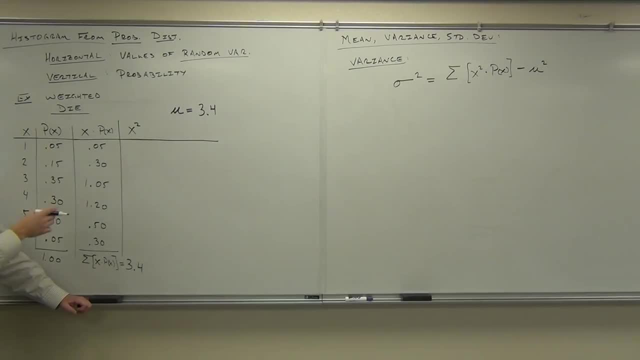 squares which aren't all that bad. Give me the x squares, starting with 1, what do we have? 1. Then 4. Then 9.. Uh-huh, 6., Keep going. 7., 8.. 9., 10., 11., 12., 13., 14., 15., 16., 17., 18., 19., 20., 21., 21., 22., 23., 24.. 25., 26., 27., 28., 29., 30., 31., 32., 33., 34., 35., 36., 37., 38., 39., 40., 41.. 42., 42., 43., 44., 44., 45., 46., 46., 47., 48., 49., 50., 51., 52., 52., 53., 54.. 55., 56., 57., 58., 59., 60., 59., 60., 61., 61., 62., 62., 63., 63., 64., 65., 67.. 68., 69., 69., 70., 71., 72., 72., 73., 74., 74., 75., 76., 77., 78., 78., 79., 80.. 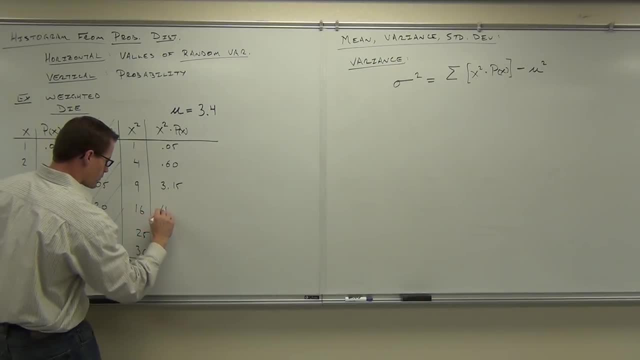 80., 81., 82., 82., 83., 84., 84., 85., 86., 87., 88., 88., 89., 90., 91., 92., 92.. 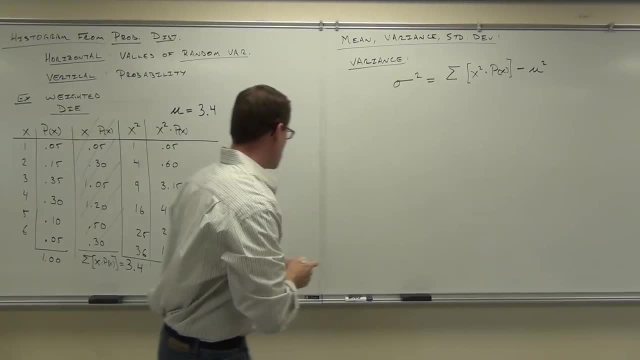 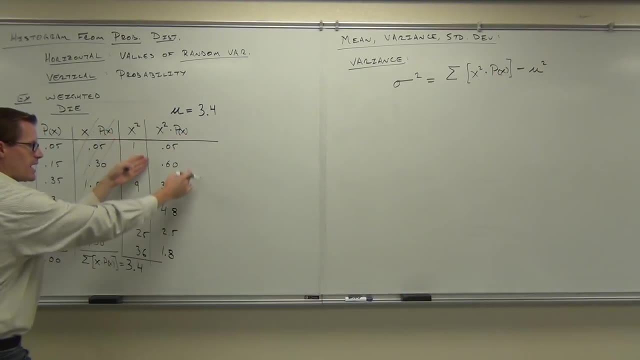 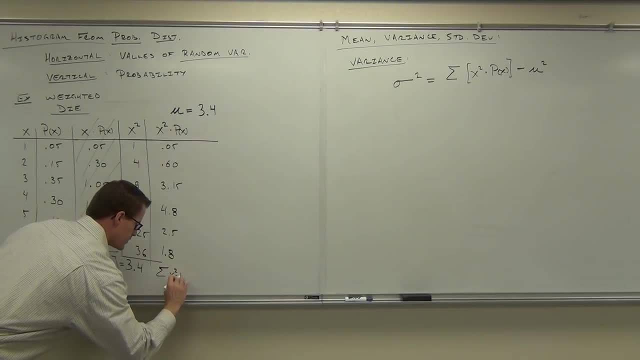 100.. 100.. 100., 100.. 1. 0. 0. 22. 0. 0. 0. 0. 4. 4., 4., 5. 1.. 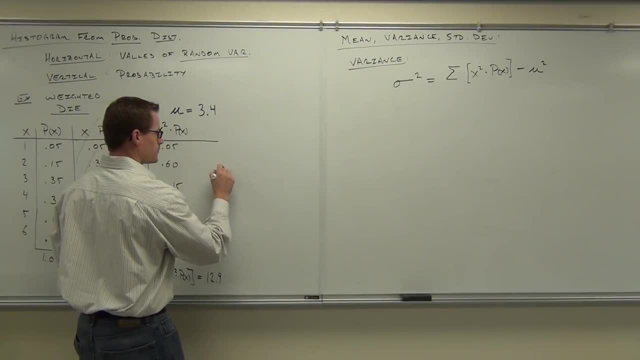 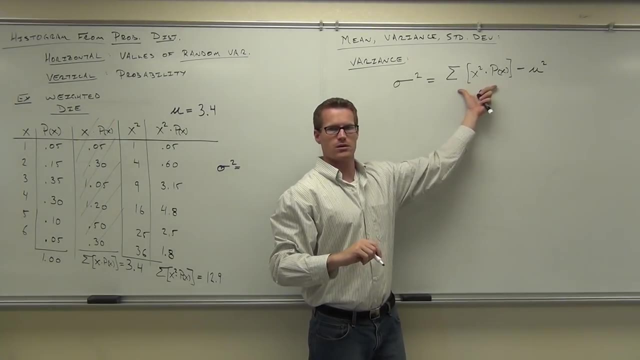 7., 26., 26., 77., 78., 99.. We have this amount. How much is this amount from here to here? Are you guys with me on that? We just found that That's 12.9.. 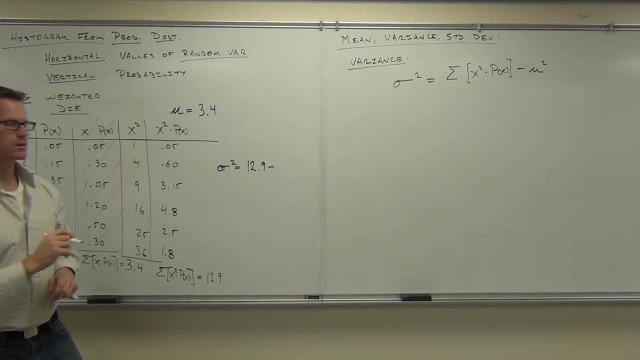 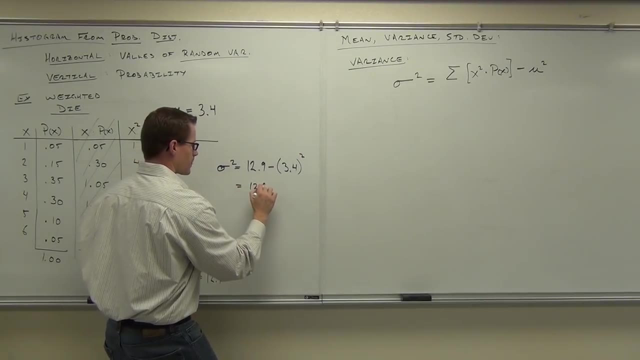 Minus the mean squared. What's the mean? What do you have to do to that Square? Don't forget the square. So we're going to take 12.9 minus what's 3.4 squared, 12.9 minus 11.56, and our variance is: 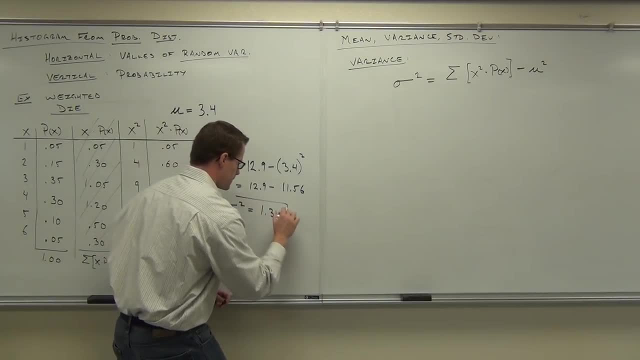 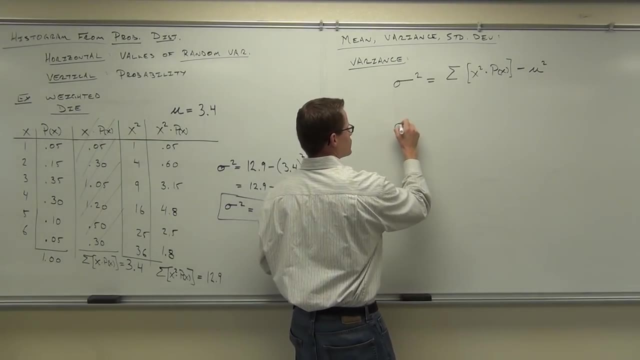 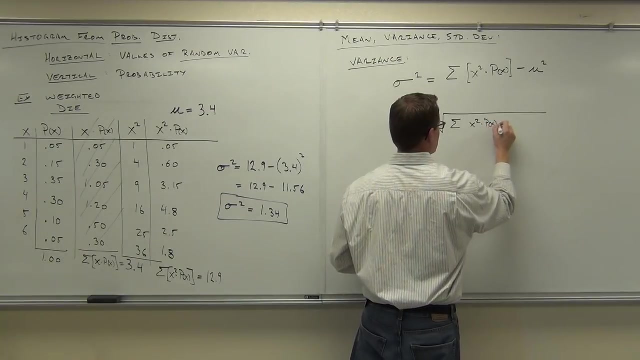 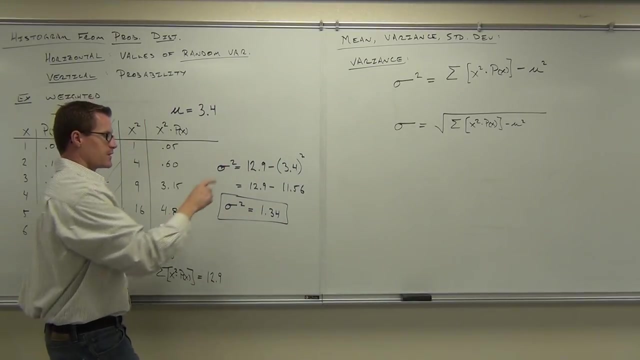 1.34.. 1.34.. We're going to find out next time that, in order to find the standard deviation, we just take a square root of the whole thing. If I square root this one, that's right. So can you take the square root of 1.34 for me? 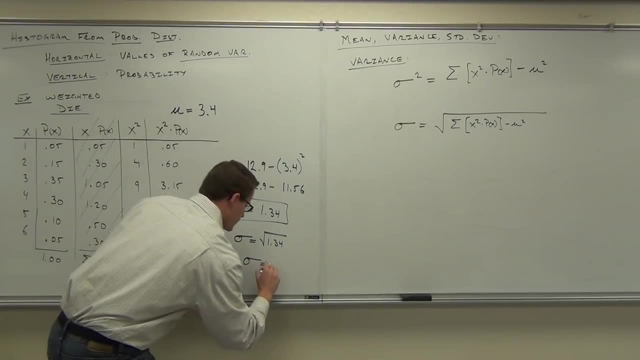 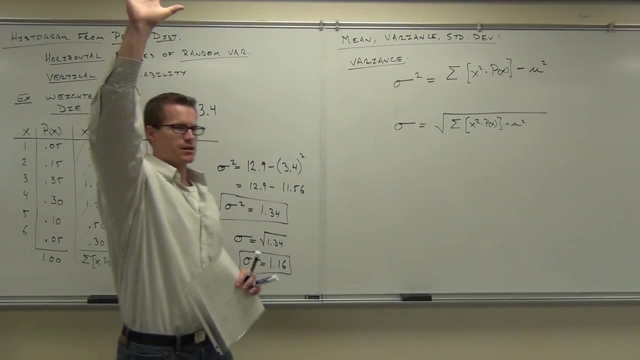 Square root of 1.34? No 1.158.. 1. 1. 1.16.. How many? Okay, what we talked about today, Okay, good, good, We'll talk about what's usual and unusual next time. 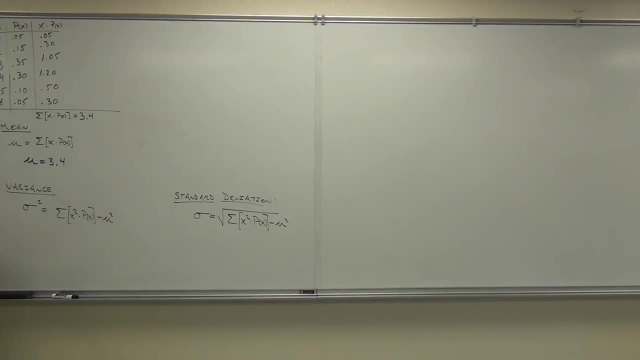 So we've already conquered finding the mean. and you'll notice that in order to find the variance and the standard deviation, which is just one extra step past the variance, we have to have the mean in our equation. So we have to find that thing first before we do anything else. 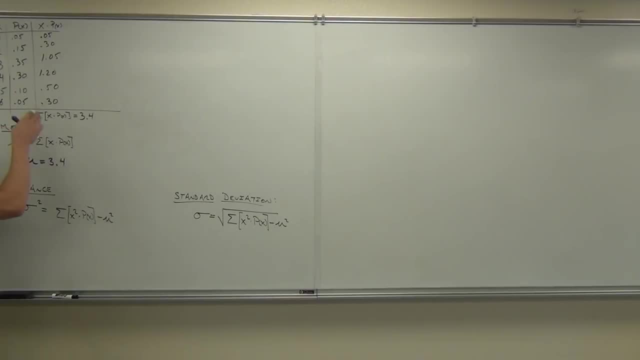 Now, what we learned last time was that after we have the mean, we're going to have these columns here. We're just going to extend this table in order to find the variance and our standard deviation. So let's keep going on this thing. 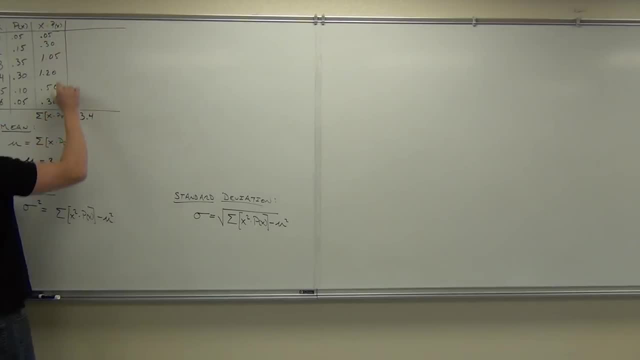 What we talked about was that people often make a mistake and then they reuse this column. After you're done with this particular column, you're not going to use that again, You're never going to go back to those numbers, So we can actually just go ahead and cross that off. 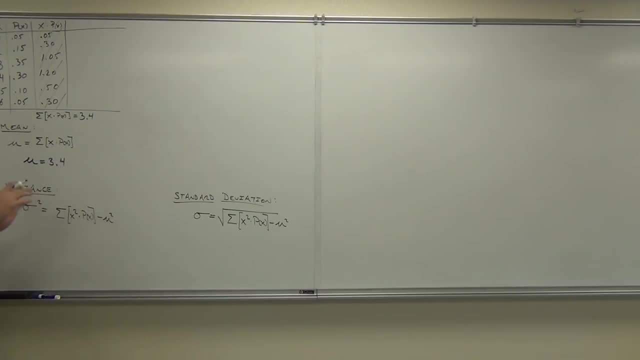 We're not coming back to that. That was simply the calculated mean. We will not be using that again, You with me, In order to calculate the variance and therefore the standard deviation, which is just the square root of it. what we need to do is accomplish this formula. 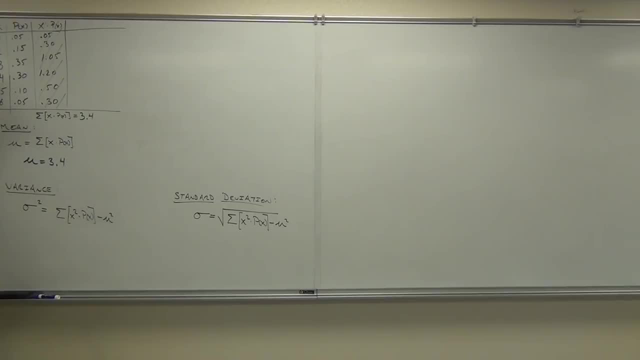 It said we find x squared first. So we're going to take all of our x's and we're going to square them. We'll make up a new column. So with our x squared- we did this last time- we're going to get 1,, 4,, 9,, 16,, 25,, 36.. 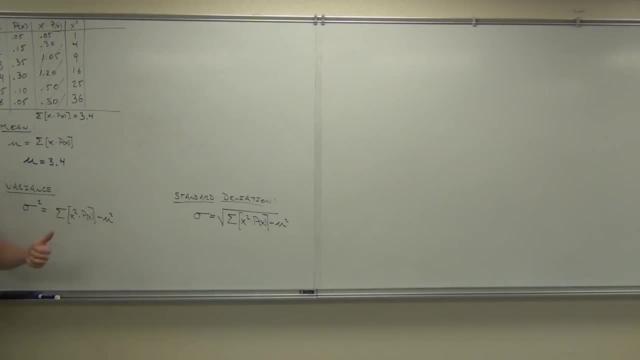 So that gives us one column. Then it says: take those x squared's and just put them together. You're going to multiply them by the probability for each of those x's. So that's why we cross this column out, because I have a lot. 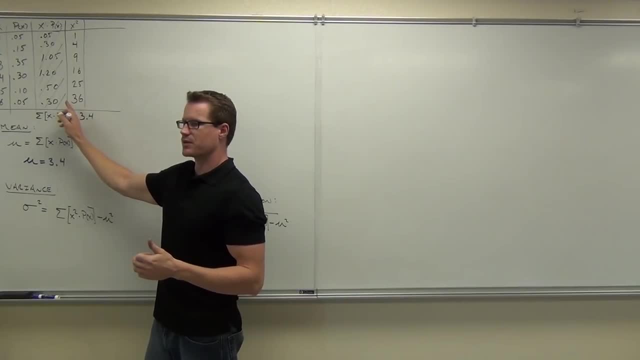 of students who, when they first learn this, they go: oh it's just these two. Now, it's not those two. Cross that out, skip over that one. It's this column: the x squared's times, our p of x. column, the p of x. 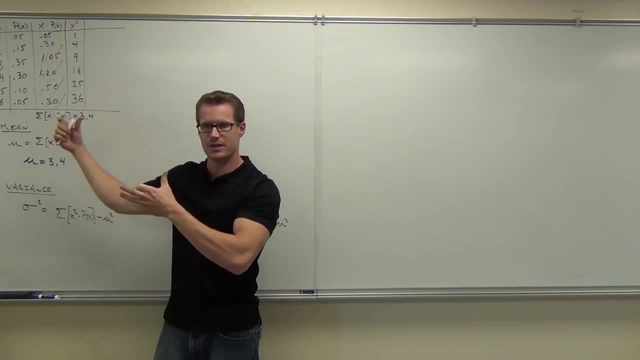 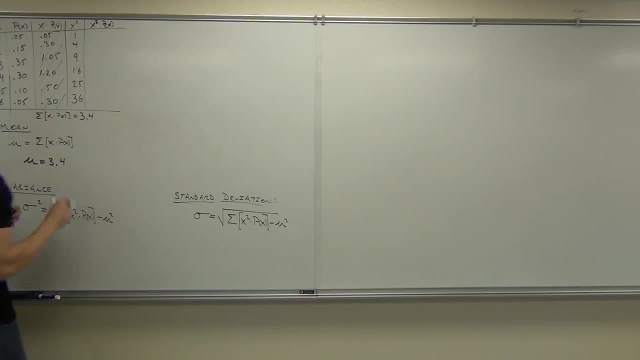 So it's these two columns being put together by multiplication. That's what we're going to have in the next x column, So we'll do x squared times p of x. We did this last time. I just want to refresh your memory on how to do this. 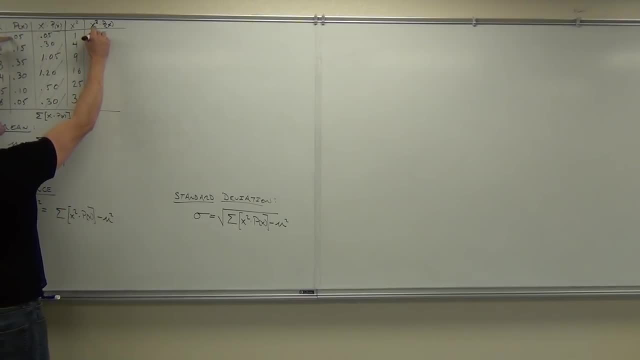 We do the 1 times .05 and get .05.. We do the 4 times .15 and get .60.. We do the 9 times the .35. and what did I get out of there? How much: 3.15.. 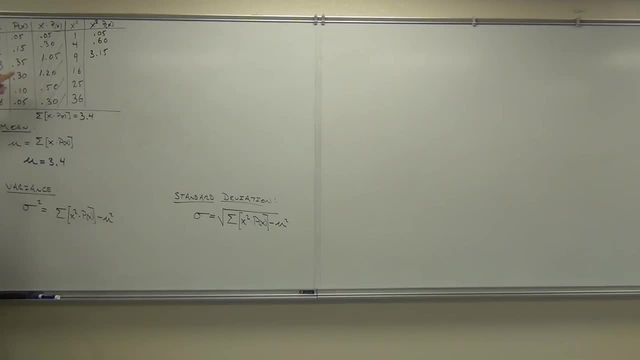 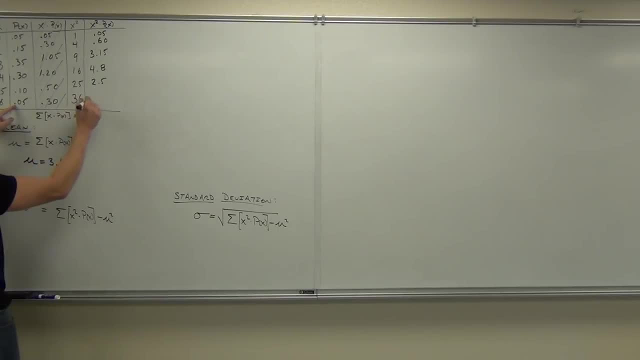 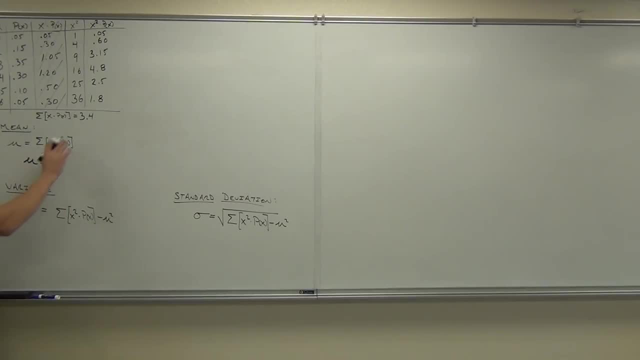 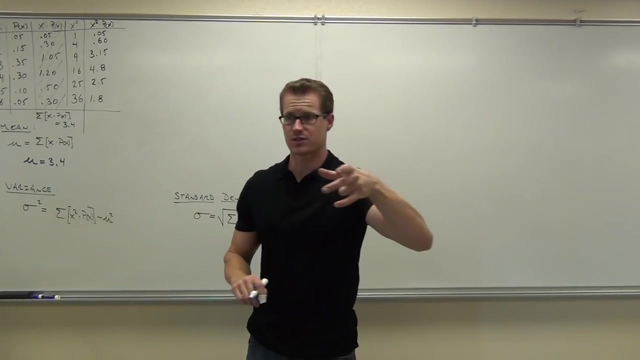 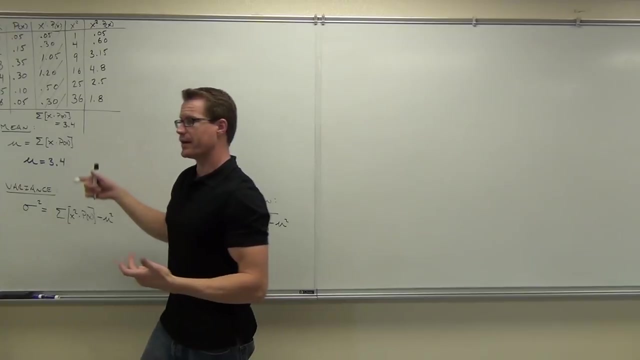 What our formula says to do is take those x squares and multiply them by the probability for each of those x's respectively, And then that summation says: add up that column again. so just like we did on this column, We're going to add that up. 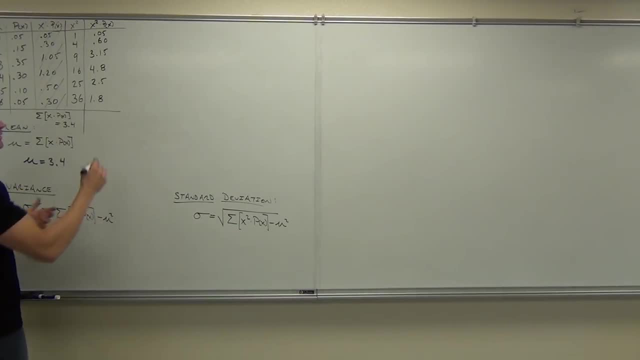 So, after we add those all up, what did we get out of that? I forgot 12.9.. So the sum of x squared times p of x, You said 12.9? Cool 12.9.. So what we found out is that our variance, which is: how do you pronounce it again? 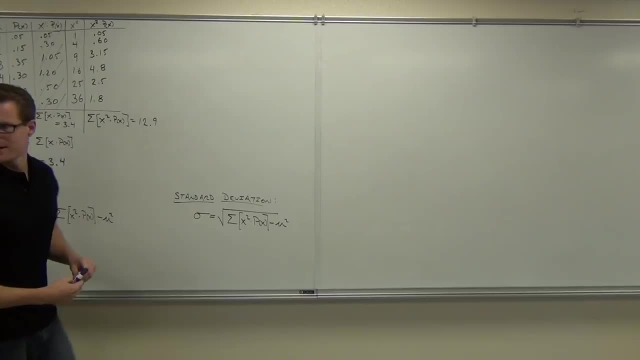 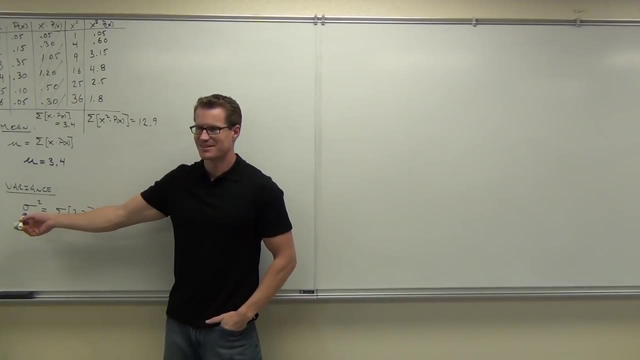 Are you guys awake today? You with me, You better be here. This is good stuff today. Canon squared right, Sigma squared. We say sigma squared. That's our variance. This stands for the variance, So the squared part. this is not variance squared. 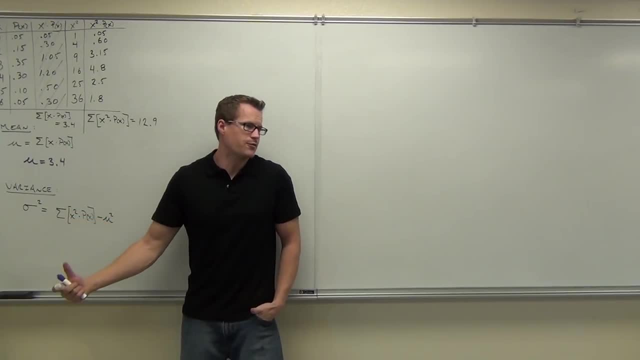 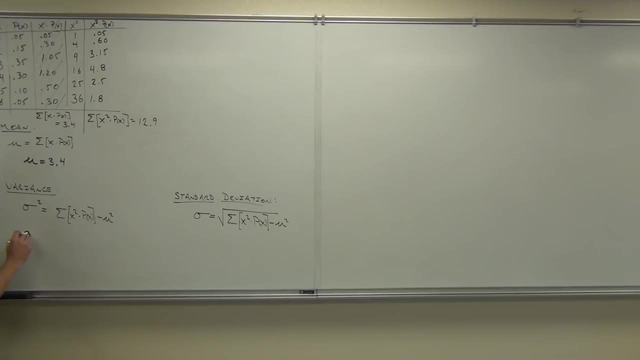 The whole thing is variance. Are you with me on that? So when you write out variance it has a little square there. that's in the name of it. Variance is sigma squared. So it says our variance sigma squared Is equal to that 12.9.. 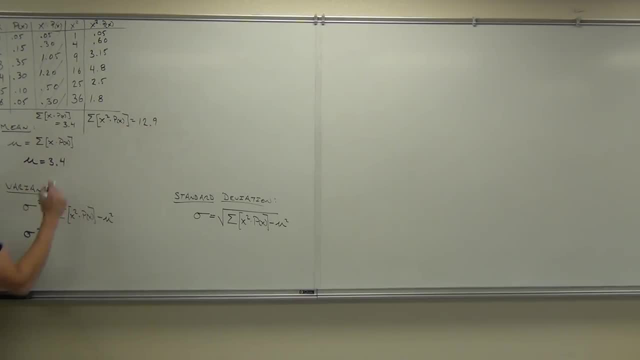 This is our x squared times p of x, and then we add it all together, That's the 12.9.. But then it says there's a crack something. This is why we had to find the mean. first It said: you find that mean and you square it. 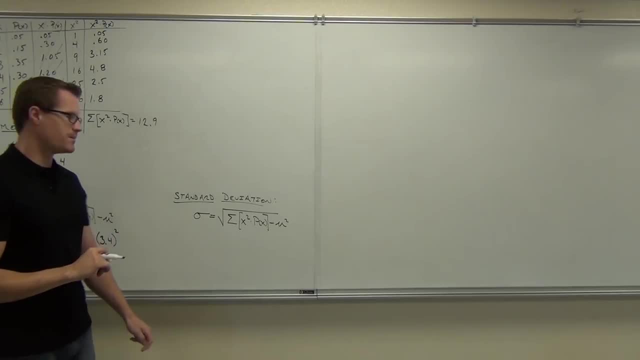 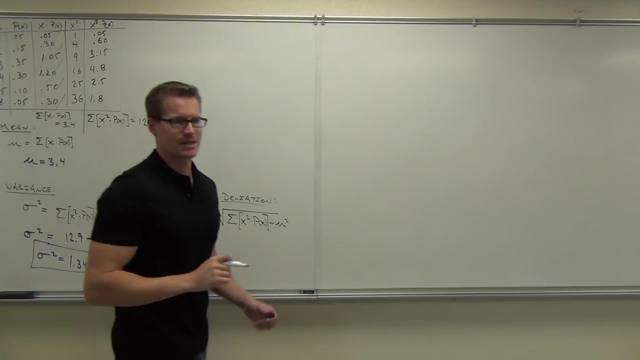 We're going to take that away from 12.9.. Do that for me. Do 12.9 minus 3.4 squared and tell me what our sigma squared or variance is. One point, Three, Four. Now the last couple seconds of class. I said that if we find the variance, 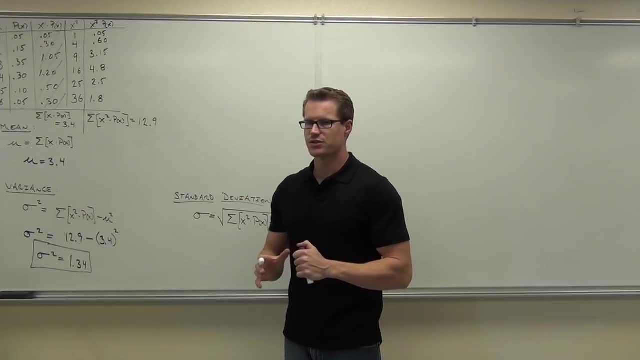 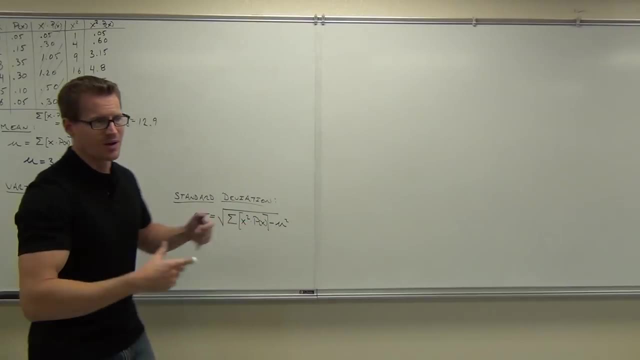 inherently, we already have the standard deviation. There's just one other thing that you have to do with it. Here's the idea. I want you to look at the symbols for this, The symbols for variance. come on, focus in up here. 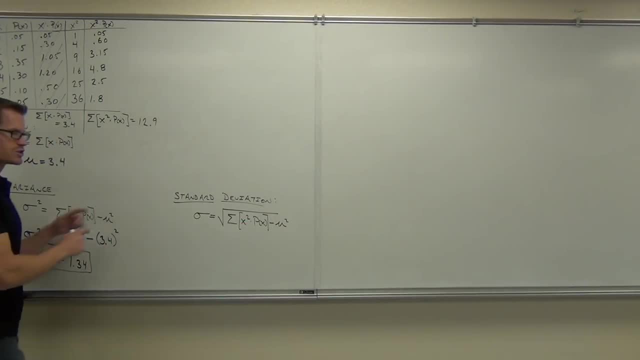 The symbols for variance is sigma squared. What we want to get is just the sigma by itself. So how do you get rid of that square? Treat it like a Square root, Take the square root of both sides. That's what we're doing here. 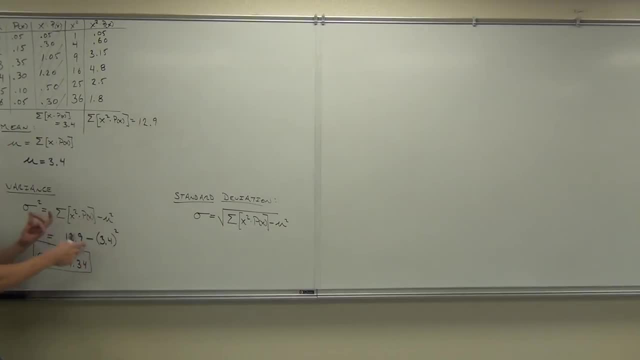 So notice, to get from our variance to our standard deviation, To eliminate the square, we take a square root of both sides. That gives us a standard deviation. So what that means for us is that if we want to find sigma, which is a standard deviation, 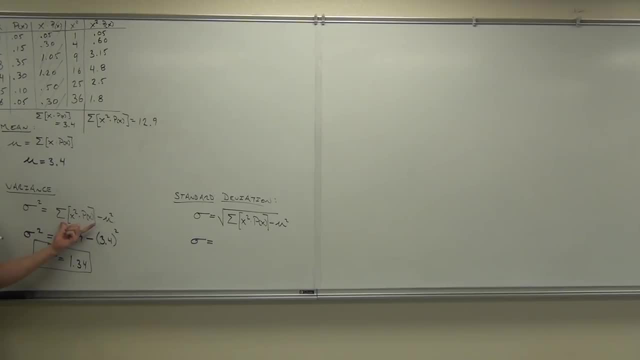 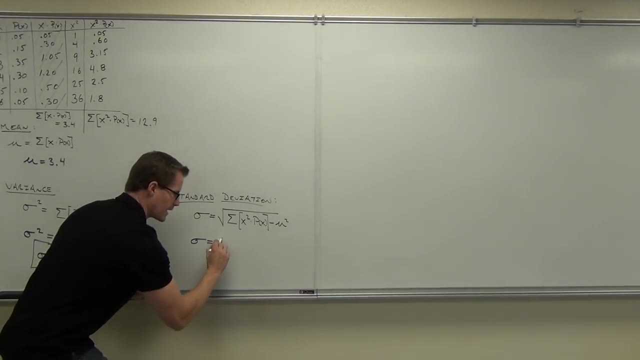 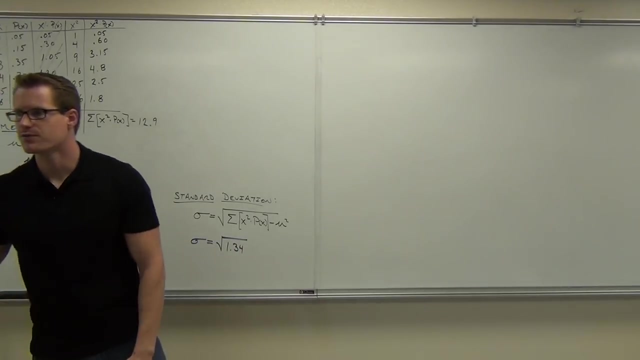 this whole thing was the radicand, which means the inside of the inside of our square root over here, the radicand of that square root. So 1.34 should be the radicand Inside that square root. All you need to do once you find the variance. if you have to find the variance, 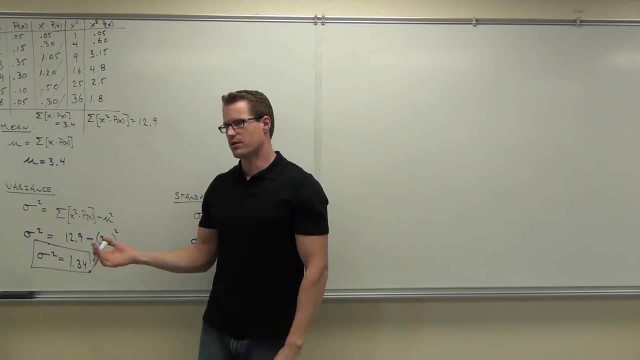 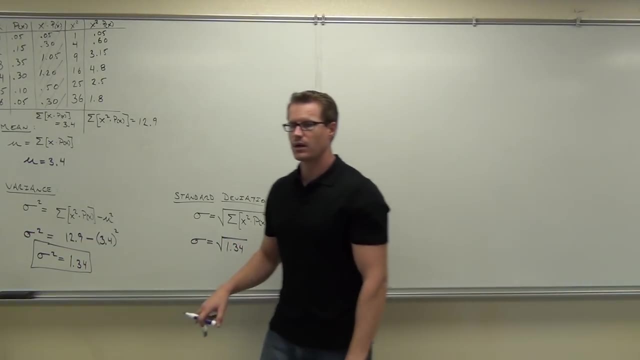 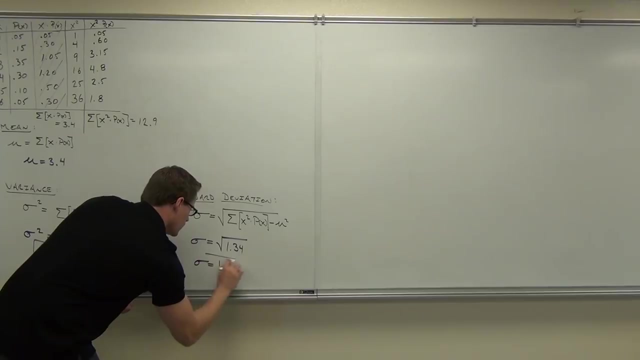 take the square root of that and that will give you your standard deviation. So let's do that. Take your square root of 1.34, and how much did you get? 1.16.. Okay, I wanted to go over this again because it was pretty quick last time. 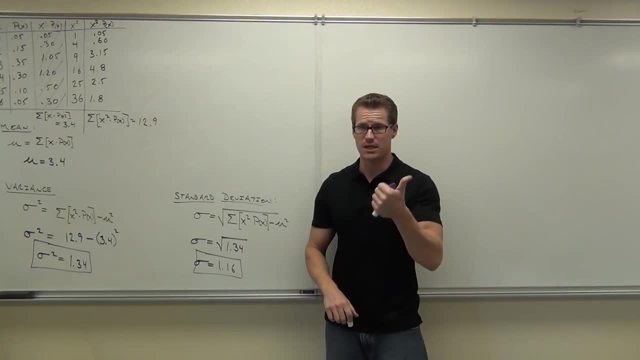 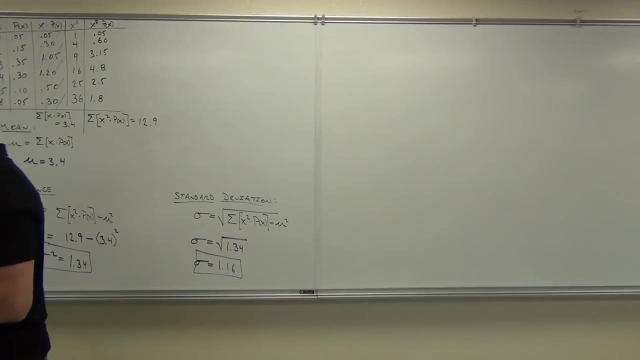 and you need to see it. Make sure you're able to do this. How many of you will feel okay on finding the mean, the variance and then the standard deviation region and feel okay with that? Cool, Now, what we learned a while back was that sometimes we're able. 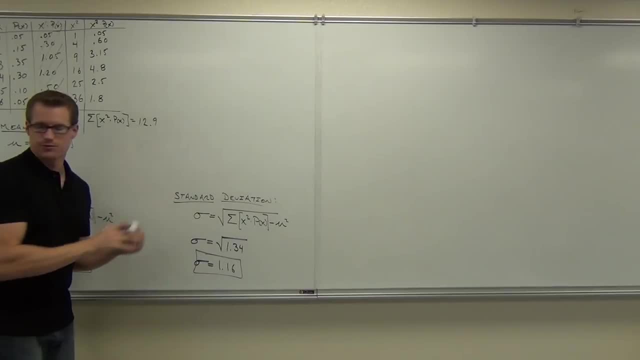 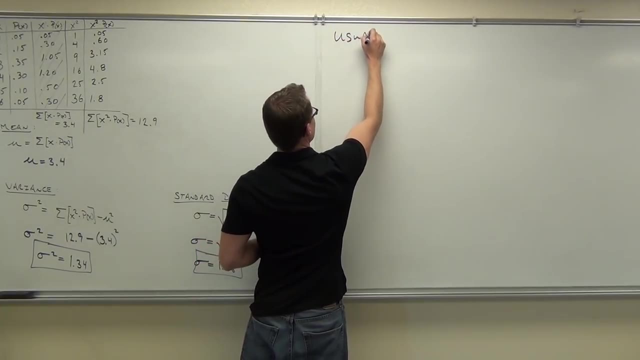 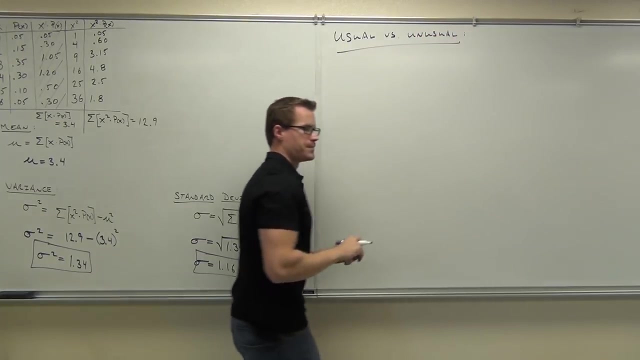 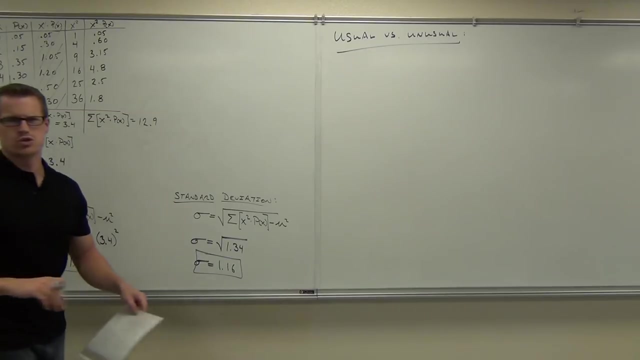 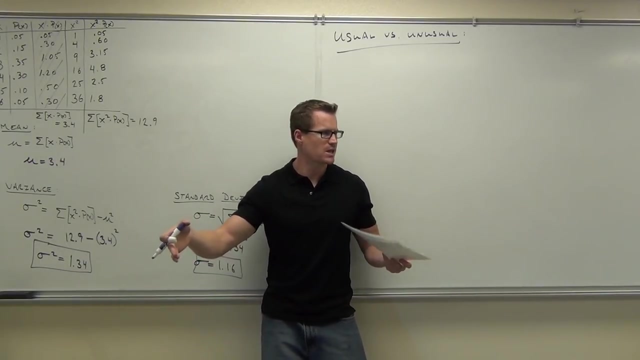 to determine whether things are usual or unusual based on this information. So let's look at usual versus unusual. Hey, what was usual outside of 2 and negative 2?? I heard 2 and negative 2.. 2 and negative 2- what's? 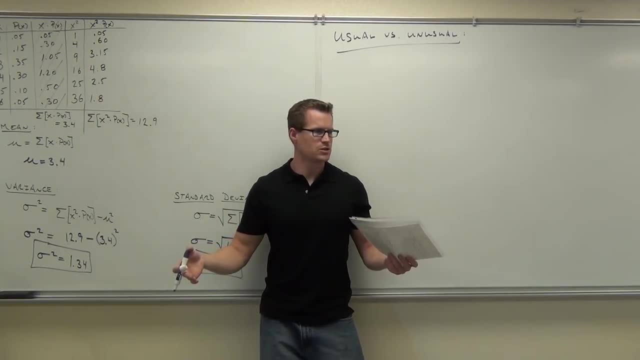 We haven't talked about z-score yet, right? So we're not talking about 2 and negative 2 itself. We haven't talked about z-score, But the standard deviations. that's what we're talking about. So we're outside of 2 standard deviations to the right and 2 standard deviations. 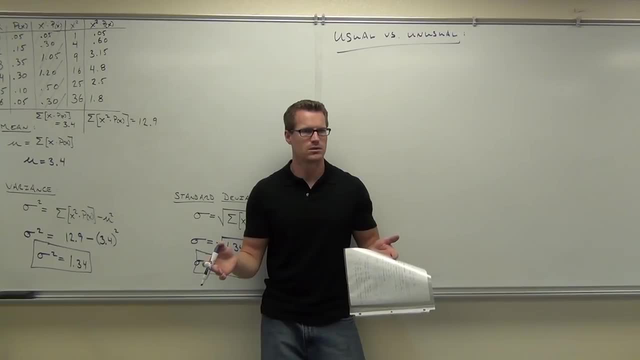 to the left of z-score. Okay, What value? What's the mean? Yeah, you're right. If we're within 2 standard deviations of the mean, we're usual. If we're outside of 2 standard deviations of the mean, we're unusual. 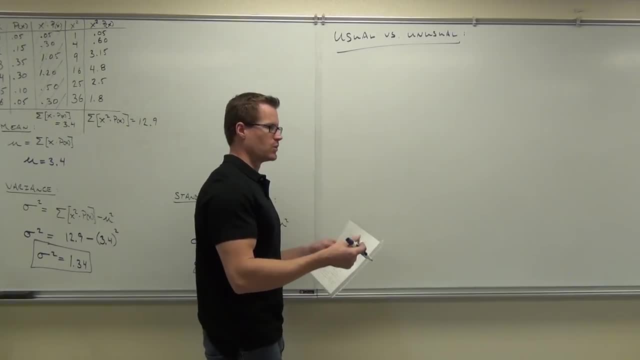 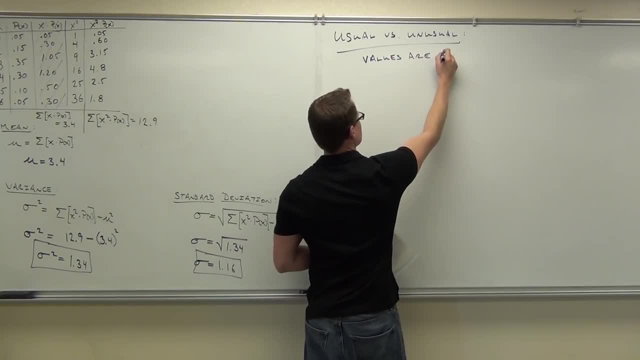 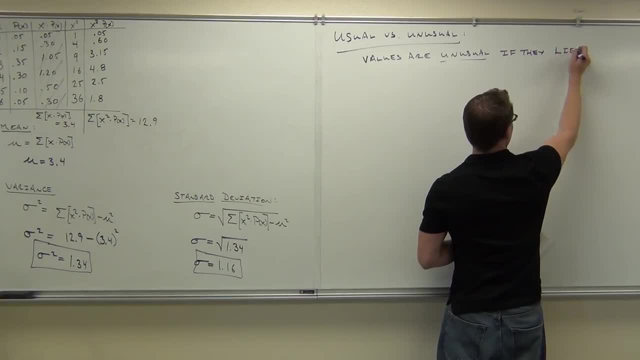 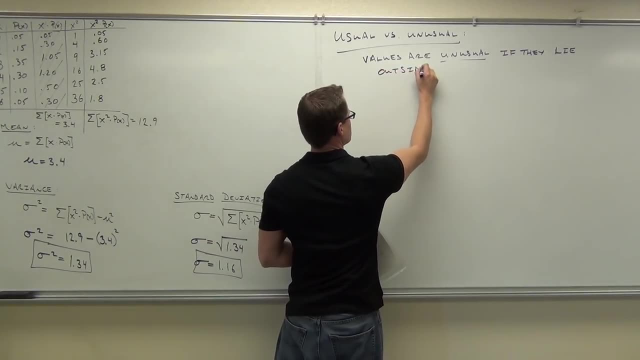 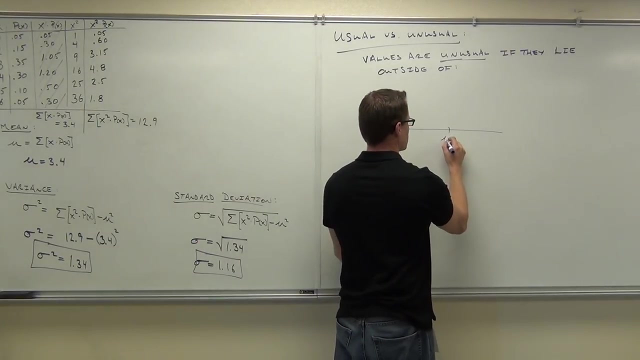 If they lie outside of this range. how do you find 2 standard deviations to the right? Remember talking about that. You'd have your. what goes in the middle? one value, You're mean, You're mean, okay. How do you find 2 standard deviations to the right? 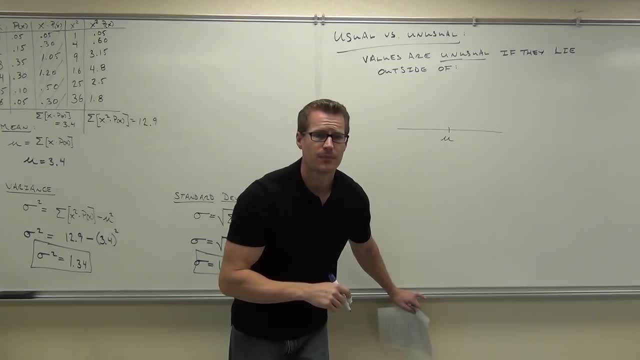 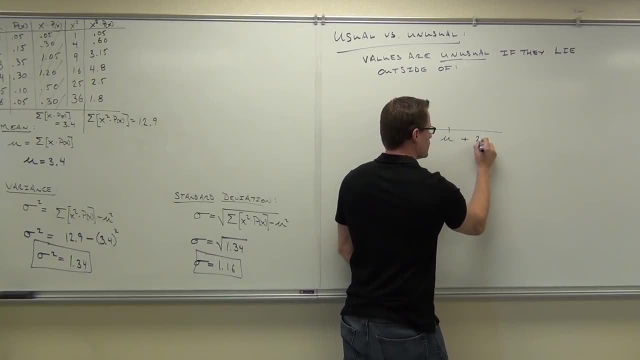 What do you do? 2 times standard deviation, add. Say what, 2 times standard deviation, 2 times standard deviation? and then Add it, add it, Add it. great, Okay. so if we add 2 sigma, that's going to give us the range. 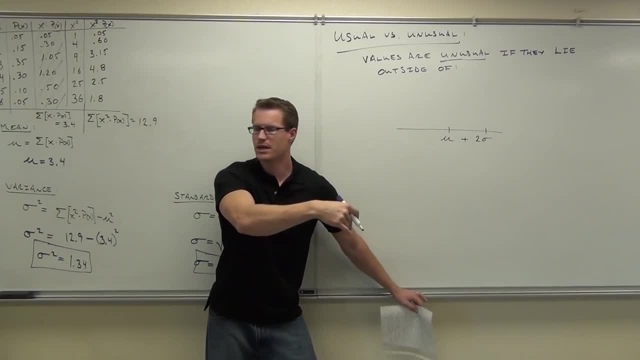 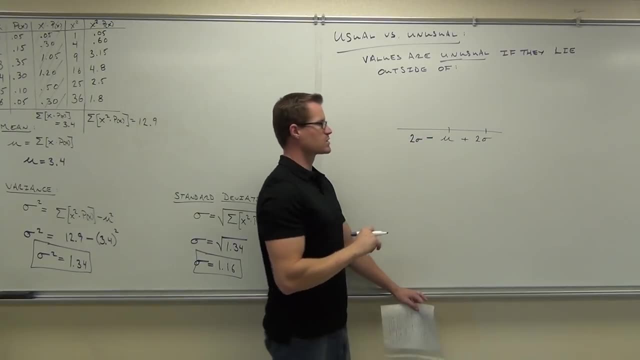 of usual values on the right-hand side- You with me on that- The maximum that we could get If we subtract 2 standard deviations- I know I'm writing this backwards, but hopefully you see it- If we subtract 2 standard deviations, 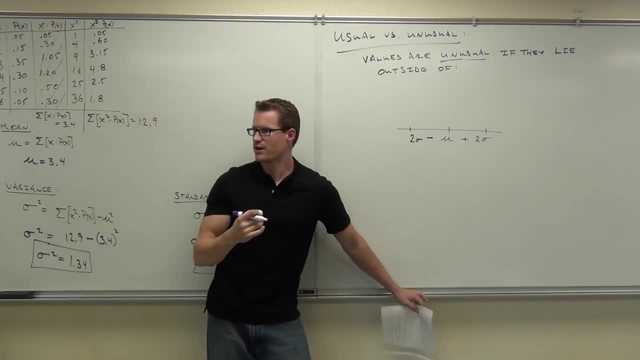 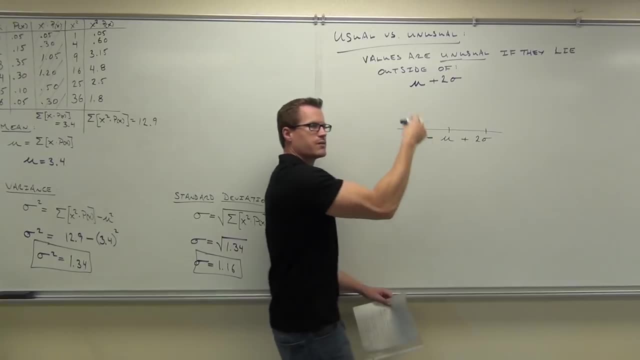 we're going to get the range on the lower limit for the range of our usual values on the left-hand side. So outside of mu plus 2 sigma, that's 2 standard deviations. 2 sigma is 2 standard deviations And mu minus 2 sigma. 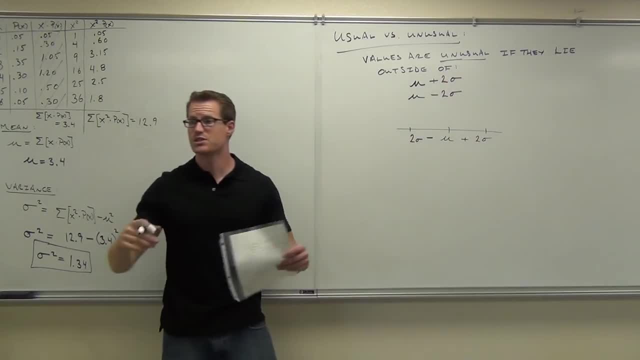 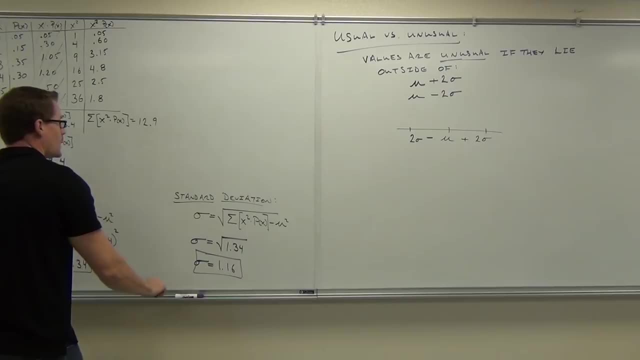 That gives us the maximum and the minimum values that we have for considered usual versus unusual. Let's see if we can do this with our weighted die. okay, For our weighted die. what's our mean Guys? you've got to be better. 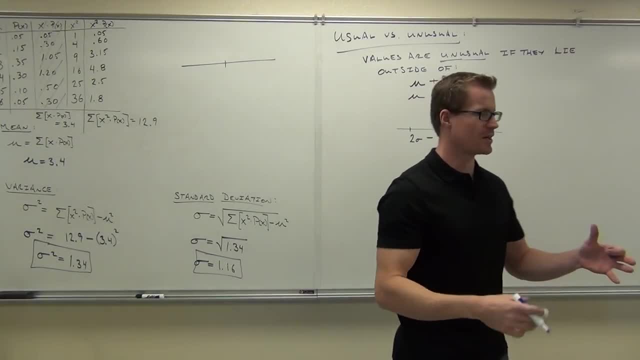 I need more participation in this. I need you to be here and with it and participate, And you can't just sit in the classroom and just sit there. This is going to drop. This is going to drop- Awesome, I know, I know. 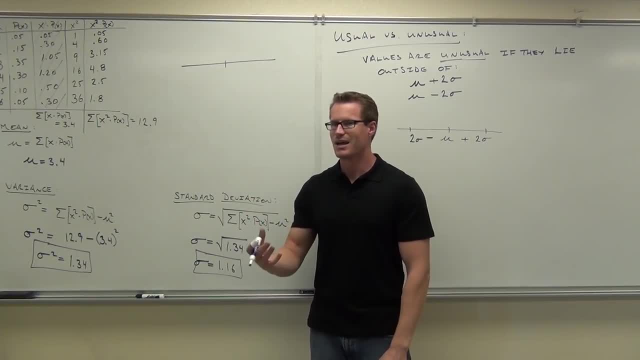 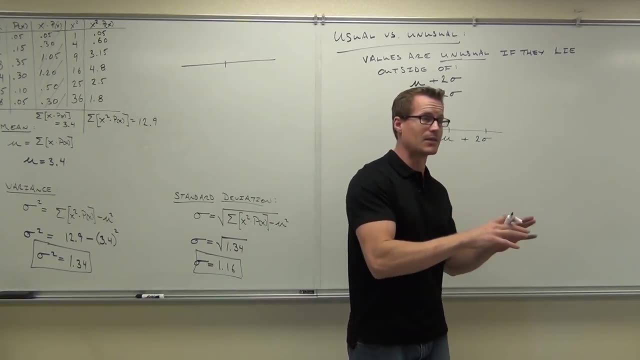 All right, But you've got to be participating because it won't sink in. If you're just listening, that's great, You're here, But if you're not participating, not verbalizing, not thinking about it, it's really not sinking in there. 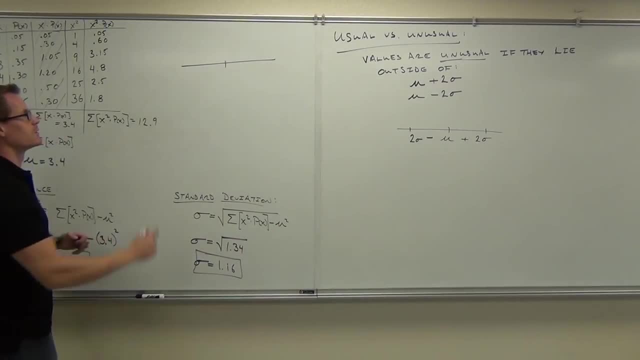 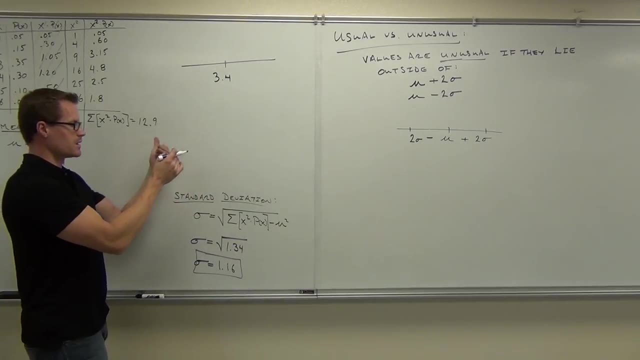 that great, So let's get with it today. What's my mean? 3.11.. I want to add 2 standard deviations to the right and subtract 2 standard deviations from the left To the left. What is my standard deviation? 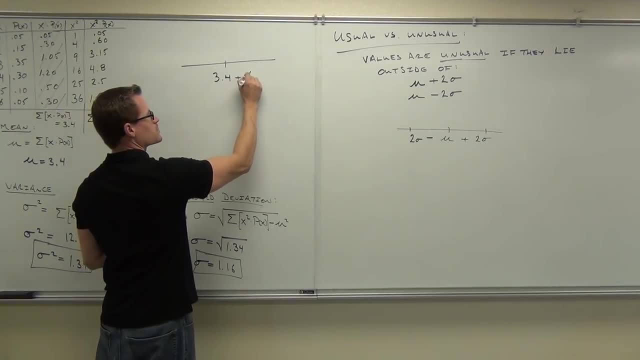 1.1.. So I want to add 2 times: 1.1., 1.1., 1.1., 1.6.. 1.1., 1.1., 1.1., 1.1.. 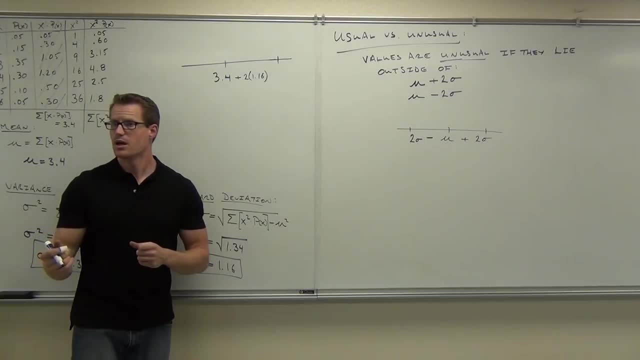 1.1., 1.1., 1.1.. So I'm adding 2.32.. Very good If I add 2.32,. so notice that we're getting 2.32.. That's 2 times 1.16.. 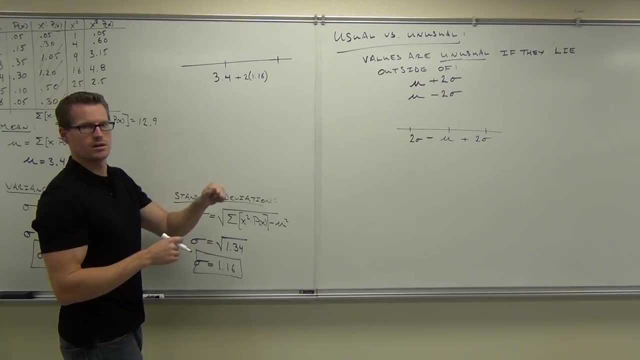 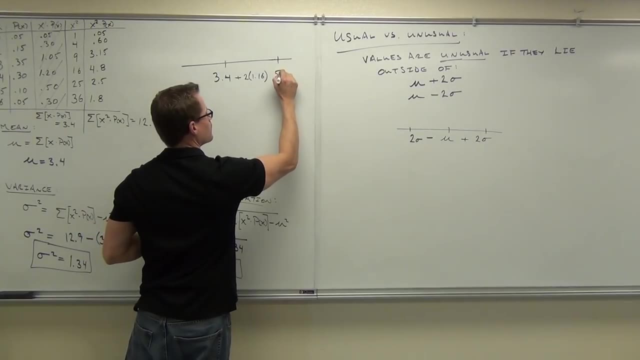 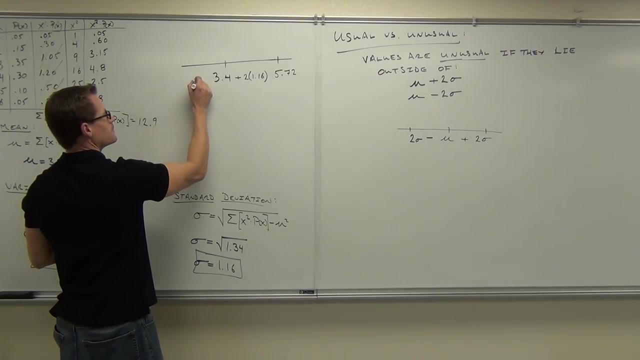 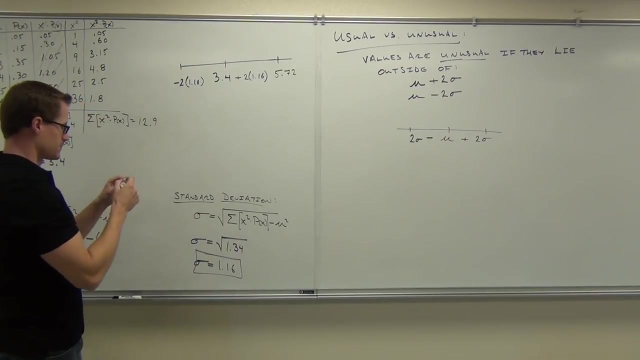 Add that on to the 3.4.. How much do you give Grace say that one more time for me- 5.72.. Now if I subtract it, So if I'm subtracting 2 times 1.16, maybe I'll put these up top so it's not as confusing. 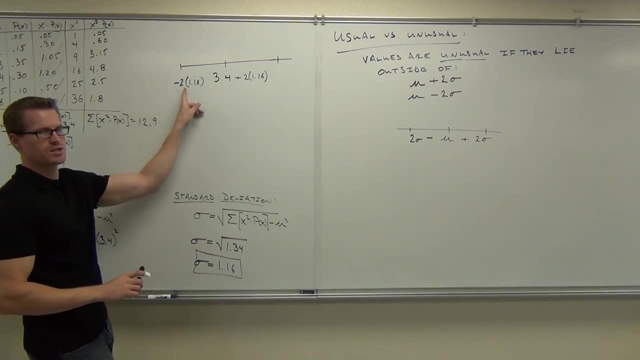 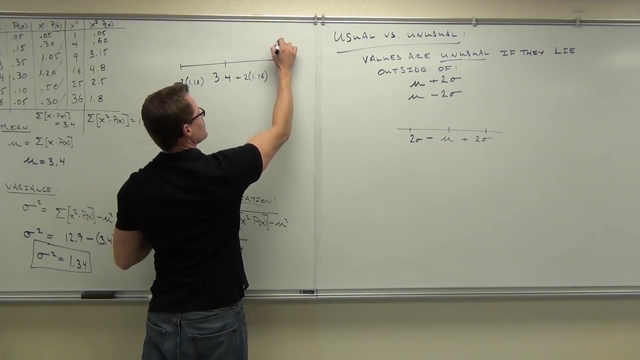 So we're adding 2 times the standard deviation and subtracting 2 times the standard deviation. That's giving us 2 standard deviations to the right, 2 standard deviations to the left. I get 5 point. oh, I erased it. what did you? what did I add there? 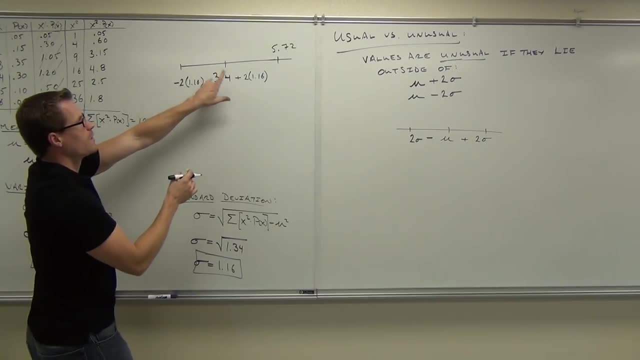 7.2. Good, And to the left-hand side, we're going to take 3.4 minus that: 1. Negative: 1.08.. Negative No, not negative No 1.08.. Oh, because I subtracted it differently, I'm sorry. 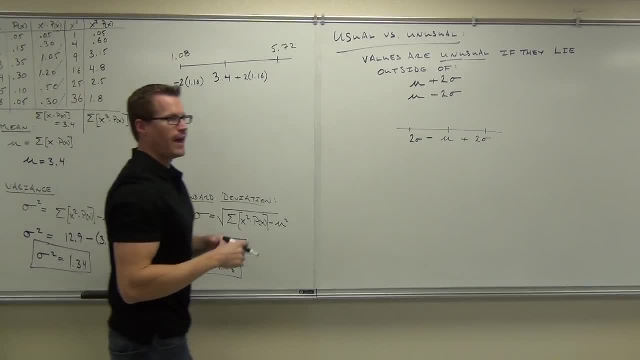 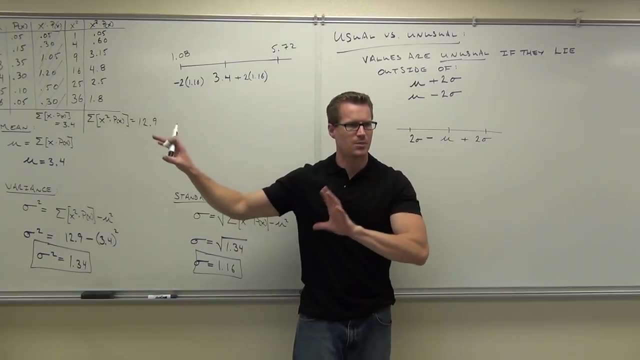 That's okay. That's okay. That gives us the range of usual values. Now, wait a second. What are we doing here? What's our procedure? What's actually accomplished? What's in our our our procedure here? What now? 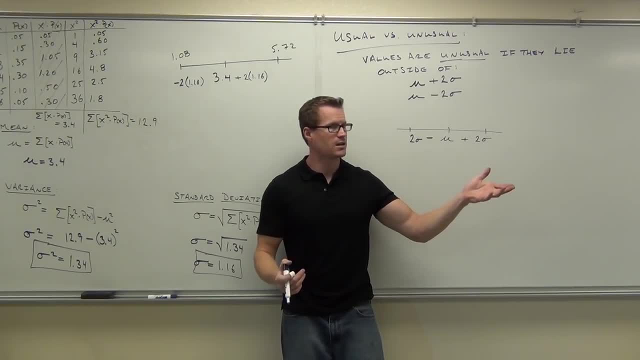 Find if it's usual or unusual. Okay, what are we finding is usual or unusual? What are we actually doing in this experiment? Finding out which numbers would be unusual. What are those numbers coming from? From the die? So we're rolling a die. 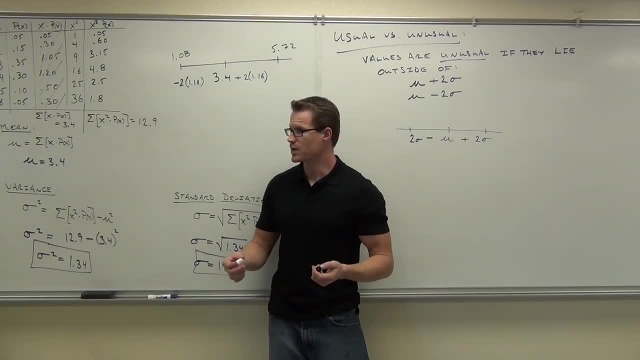 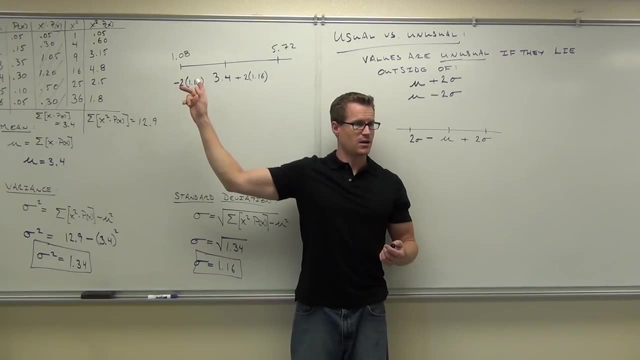 We're trying to figure out what numbers on a die would be usual and what numbers would be unusual. Does this tell it to you? Yeah, How about it? Two, Is two a usual number to get on on this particular die? Remember that this is a weighted die, right? 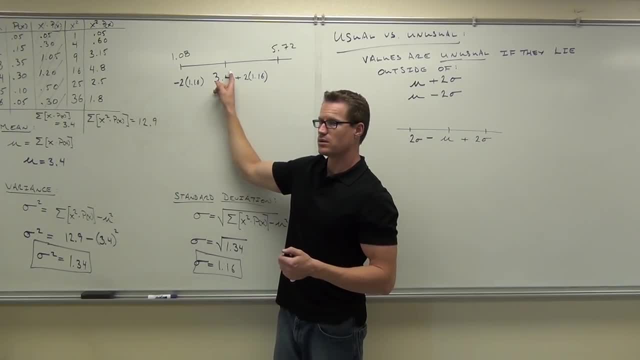 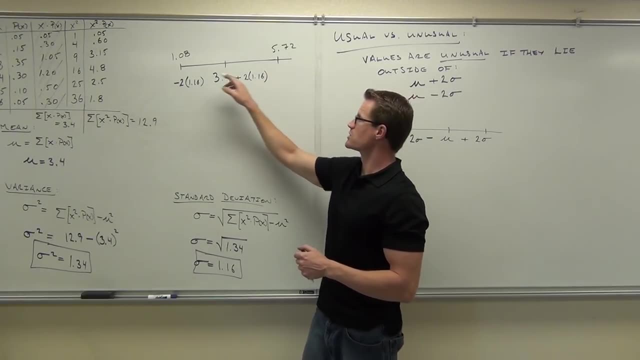 Yeah, This is a weighted die. Is two usual Where's two. Is two over here. Is two over here. Okay, Do you understand that? these are my usual values. My usual values start at 1.08 and end at 5.72.. 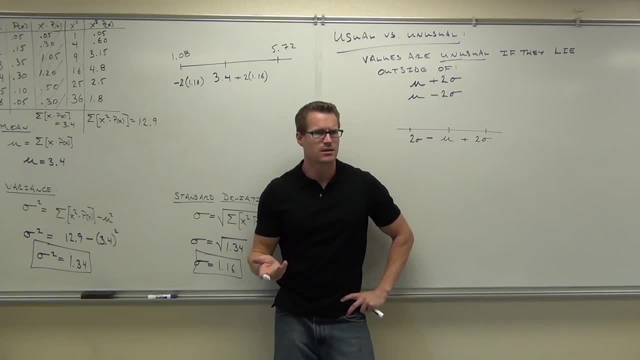 But you're thinking: wait a second, This is a die. right, Can you roll a 1.08 on a die? Probably not. But this gives us the range. This gives us a minimum. Anything below that is not going to be considered usual. 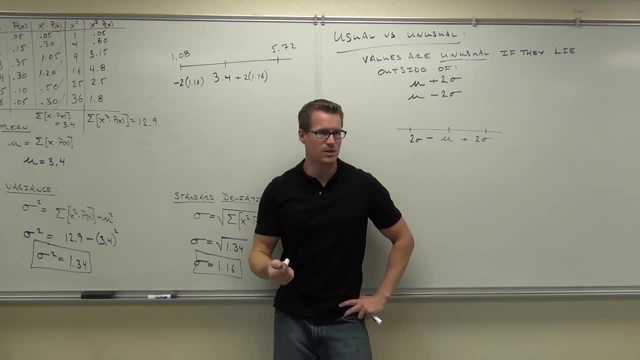 Anything above this is not going to be considered usual. So can you tell me, are there any unusual rolls? One and six? One and six Is one in this range. No, then one's unusual Is two in this range? Yes, two between 1.08 and 5.72.. 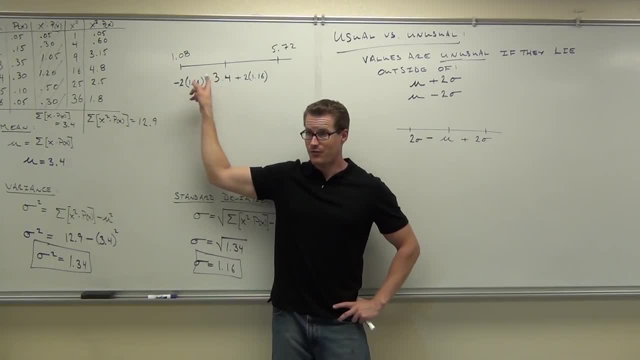 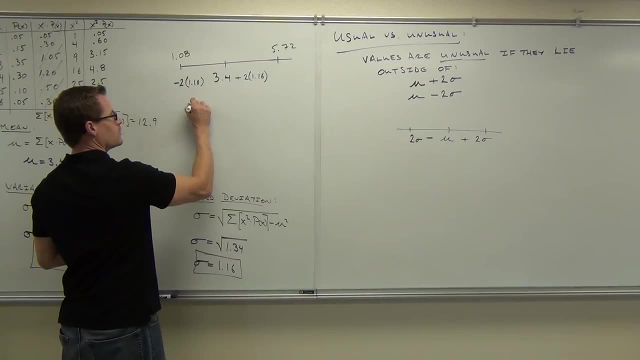 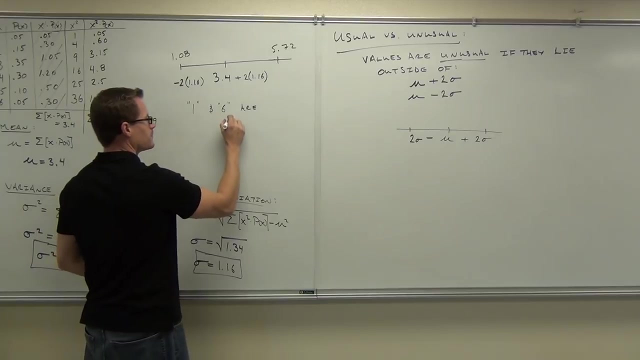 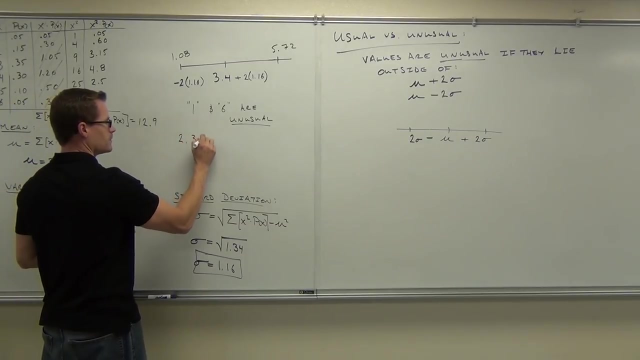 How about three? Is three usual, Definitely. How about four? How about five? Yes. How about six? Yes. So we have two unusual numbers, The numbers one. I'm putting quotations here. one and six are unusual. Two, three, four and five. hey, it falls in that range. 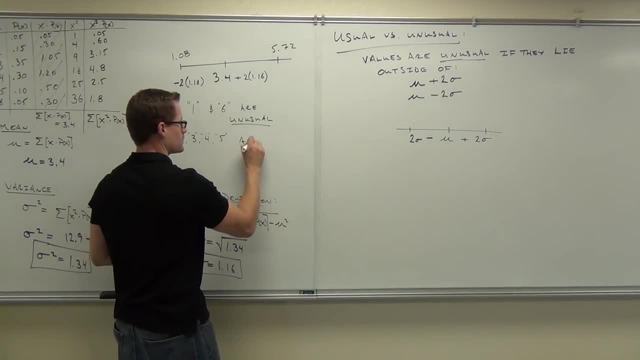 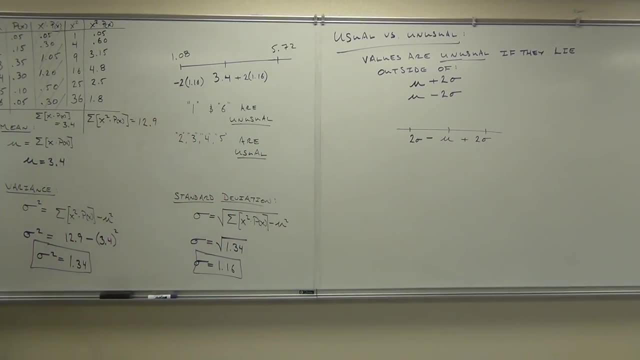 Those are considered usual values, You know. there's also one more thing I need to tell you. I haven't explained this until the end of the class, but I'm going to explain it to you in a minute. I'm going to explain it to you in a minute. 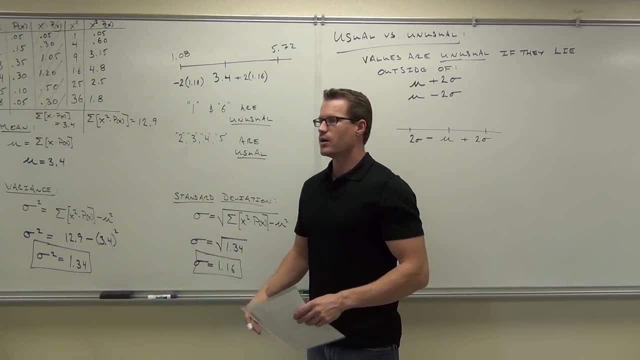 I'm going to explain it to you in a minute. I don't have it up until right now, because right now it's going to really come into play in a little while. We can also do this simply by looking at the probabilities. You may have read this in one of your earlier sections. 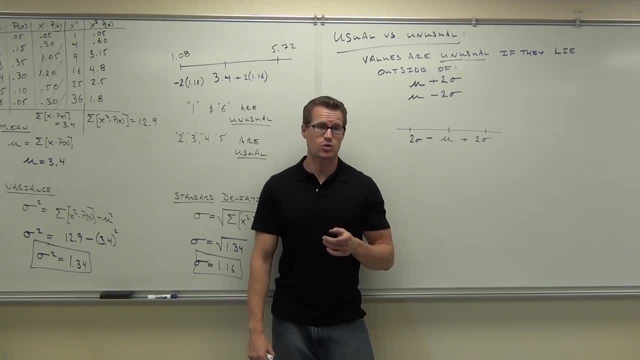 It said: well, the probability is .03.. Is that usual or unusual? Do you remember I had talked about that in your homework? We asked you: according to probability, was it usual or unusual? You probably had to read the book, right. 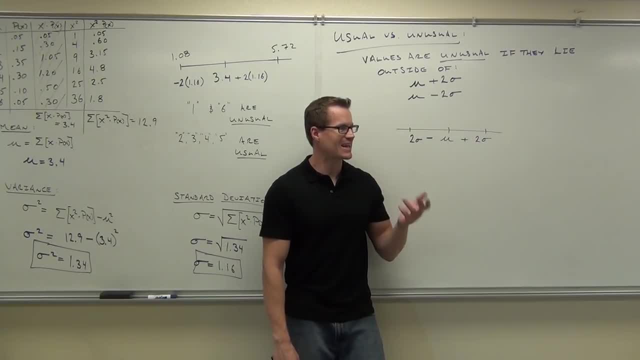 You had to read the book to find that out And it said that any probability that is less than .05 or less than 5 percent would be considered usual or unusual. considered unusual. Dr Heff, you're with me on that. 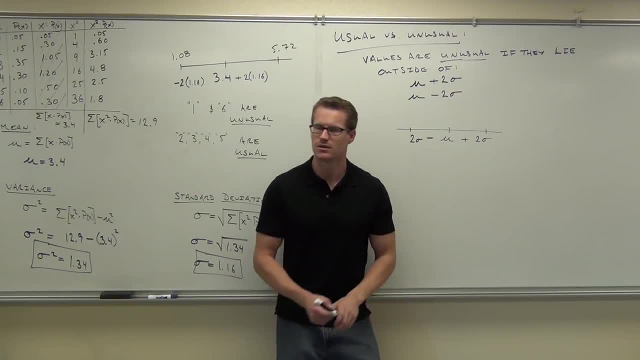 Any probability less than 5%. Why is it 5%? Because how? Why is it 5%? You remember looking at that And we said two standard deviations was the same thing as a z-score of 2 or negative 2.. 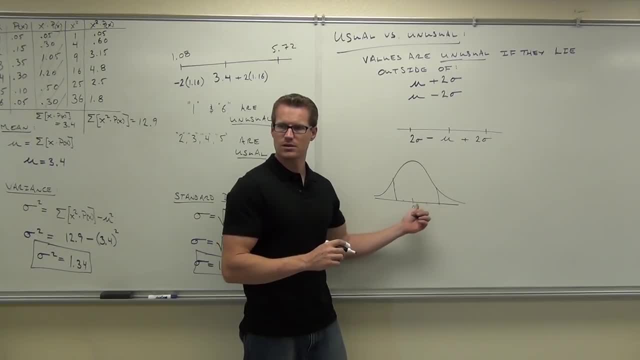 What percentage of the data falls between two standard deviations? What percentage? Remember the empirical rule. You need to know the empirical rule. The empirical rule said: within one standard deviation, within one standard deviation from the mean, you get how much percent of the data. 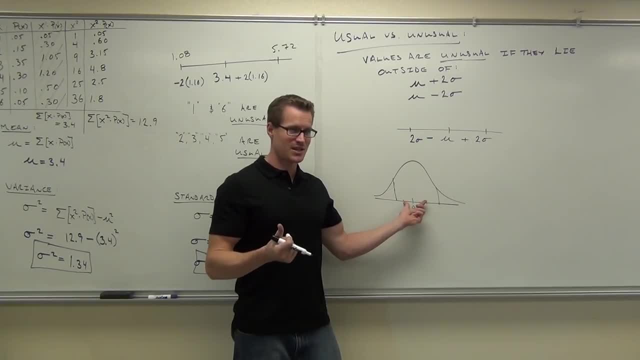 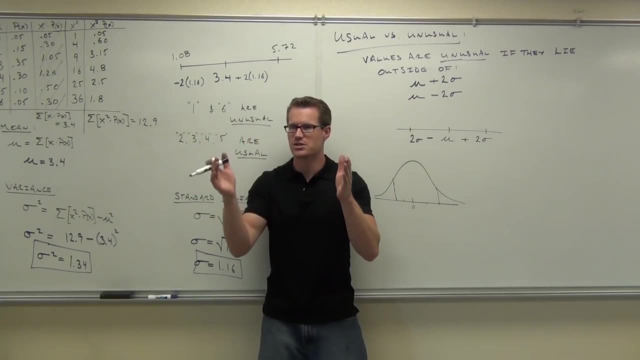 60? 61 higher than 67? 68. 68.. If I extend that to two standard deviations, please be listening here. If I extend that to two standard deviations, what percentage is in that? 95.. 95.. 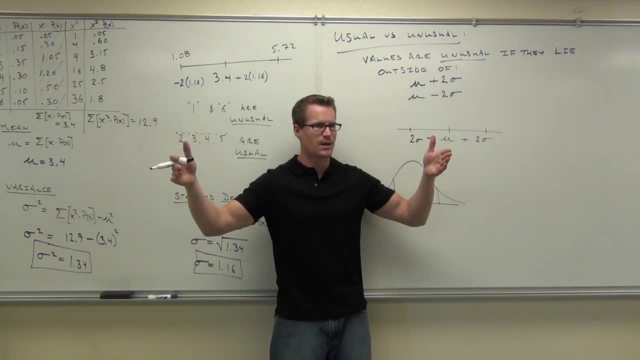 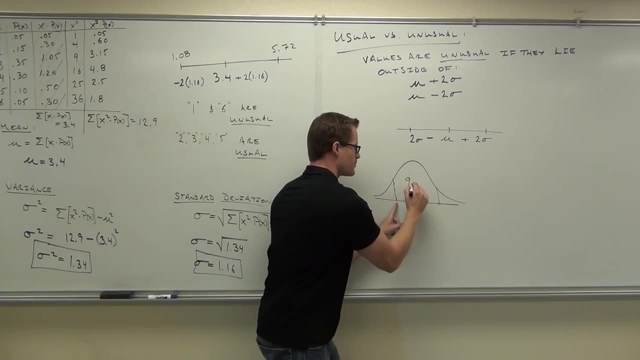 If I extend it to three standard deviations, you get 99.7.. 99.7.. Is those numbers ringing a bell? So here's the idea: If usual and unusual is within two standard deviations and there's 95% of the data within those two, 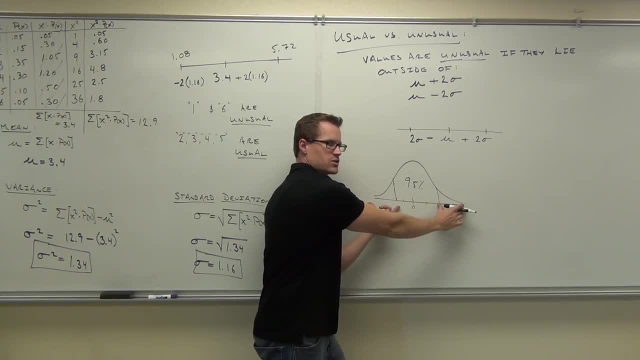 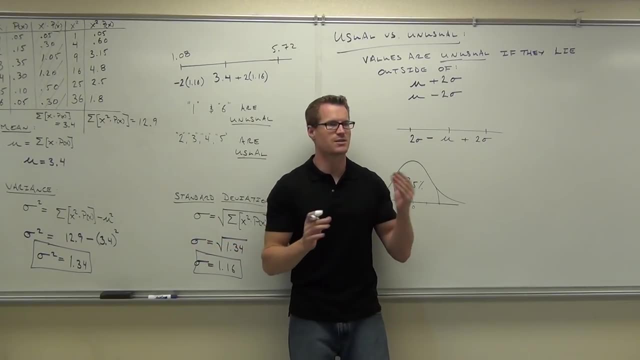 standard deviations. what percent of the data is outside of those two standard deviations? 5%. That's where we're getting that 5% from. It's the same rule. It's just saying if the probability is less than 5%, you are outside of those two standard deviations. 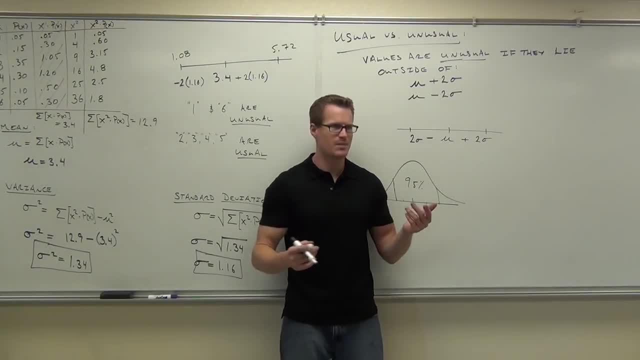 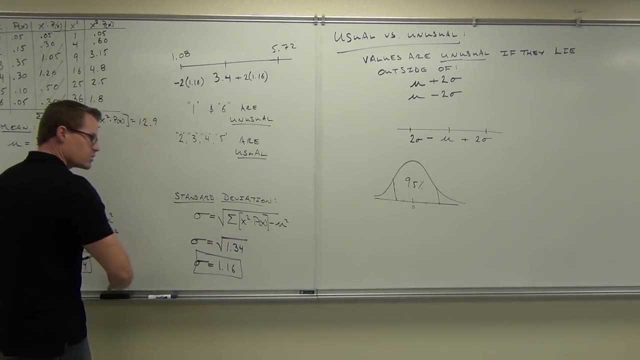 Therefore you are going to have an unusual probability. Does that make sense to you? So same idea. It's just a different way of looking at it, without a graph or without the standard deviation idea. So, according to the probability, if the probability of an event 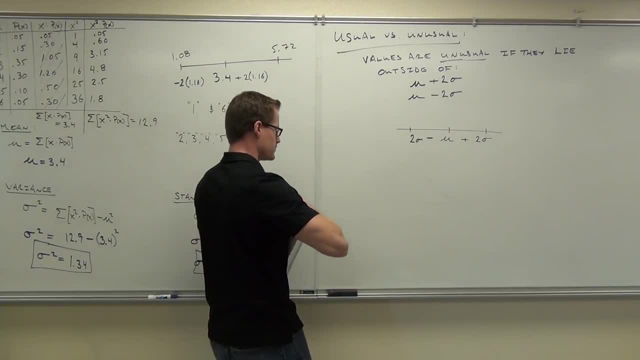 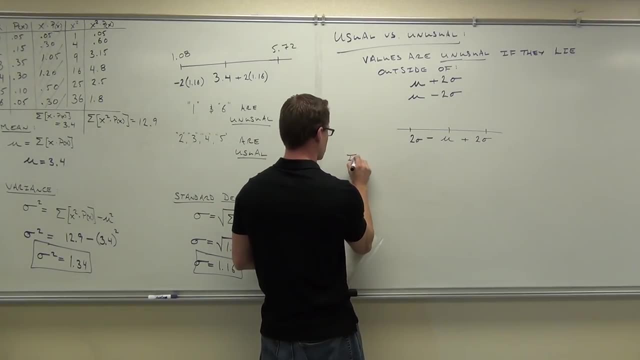 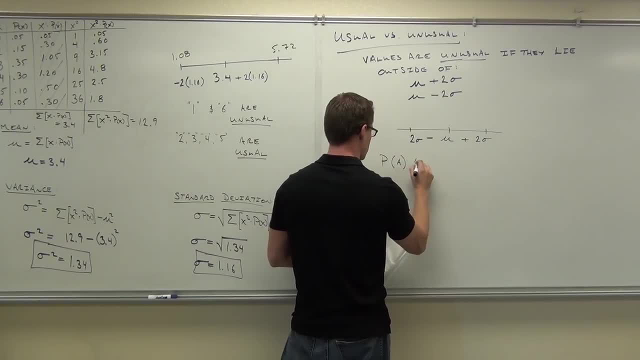 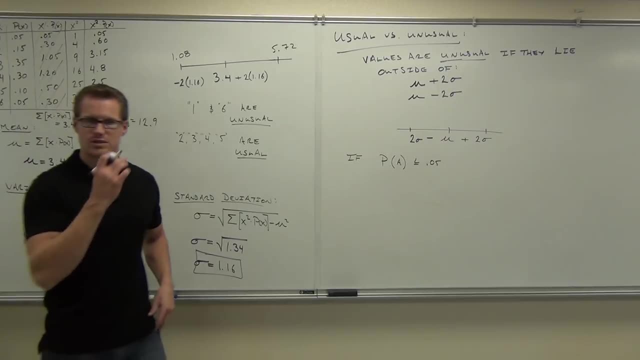 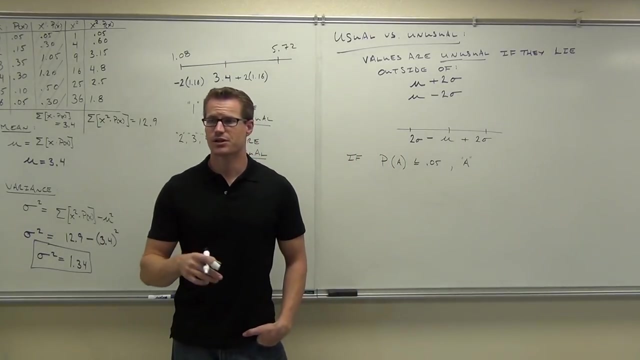 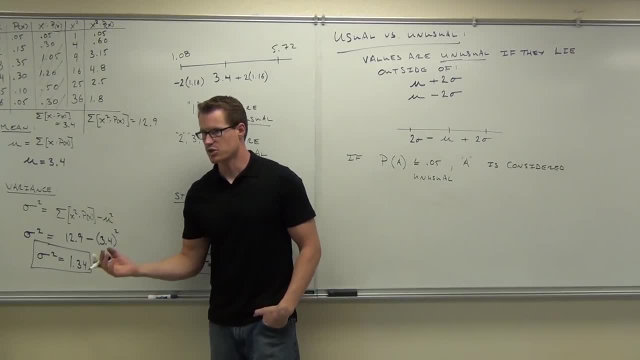 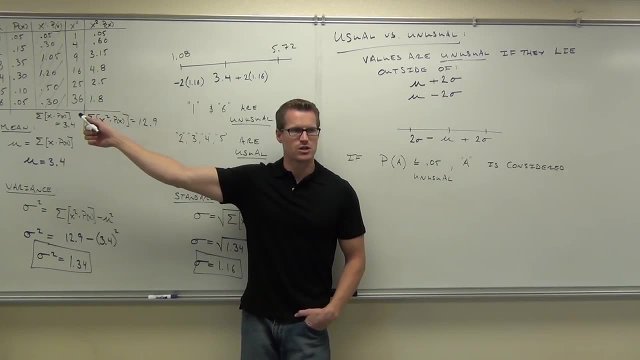 This means if it's greater than .05, we have something that is, of course, usual. Can you tell me just by looking at my probability distribution everyone? look at the board over there on the left-hand side, the probability distribution. 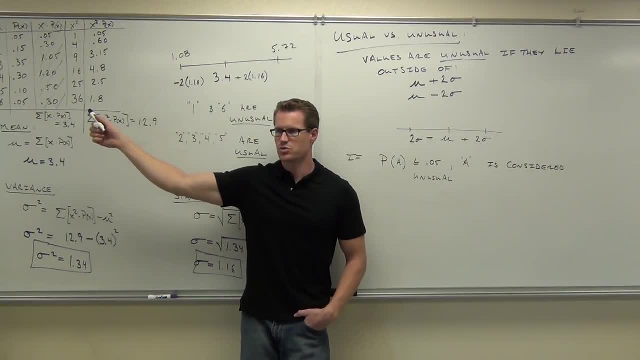 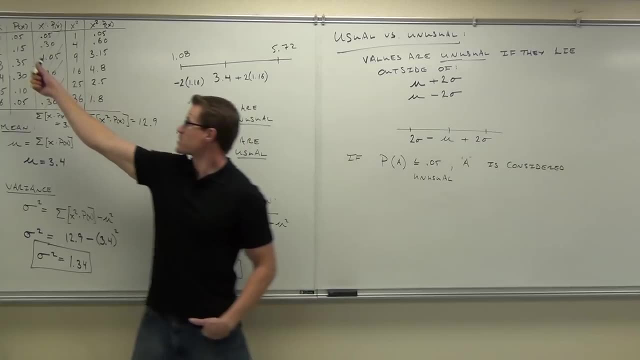 Can you see those probabilities? Do any of those tell you right off the bat which are usual and unusual? I'll check it out. Which one is unusual? One that's five percent Less than or equal to five percent. so .05, that's unusual. 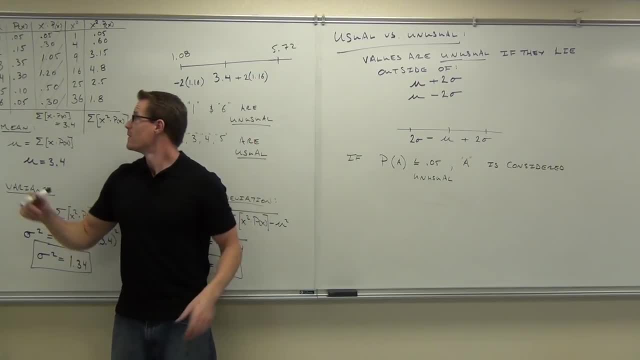 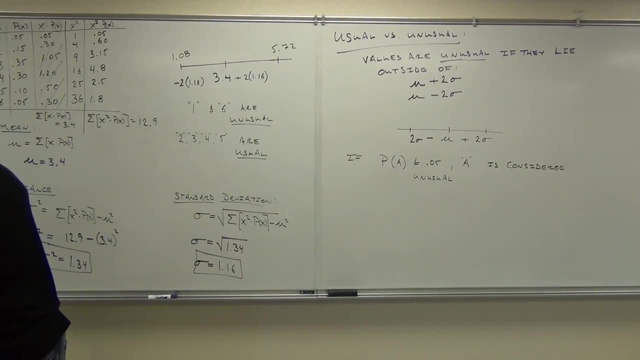 .05,. that's also unusual. It matches up to what we talked about here. These ones are considered usual. How many of you understood that word? Good, I'm gonna kind of feed into the next one. Let's do one more example on that. 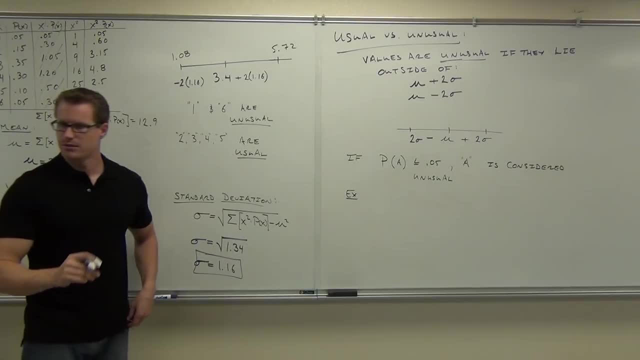 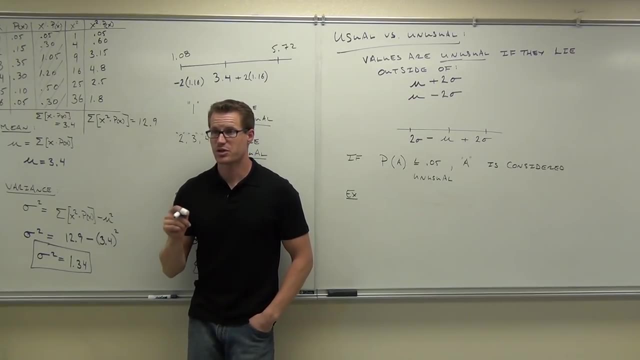 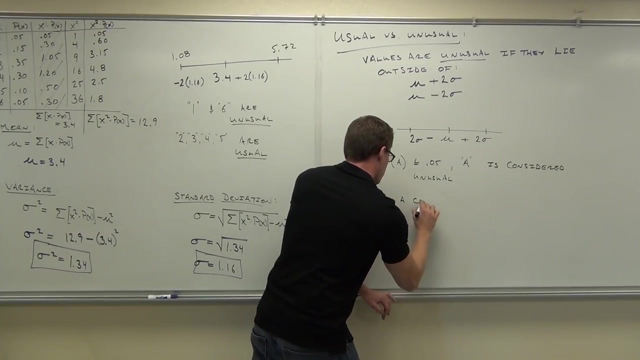 You know, if you flipped a coin a thousand times- coin with heads and tails on it- the probability of getting exactly a certain number of heads is pretty rare. For instance, if I said you're gonna flip a coin a thousand times, what's the probability that you're going to get exactly? 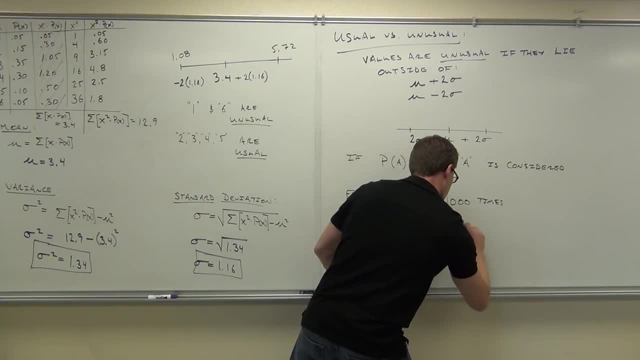 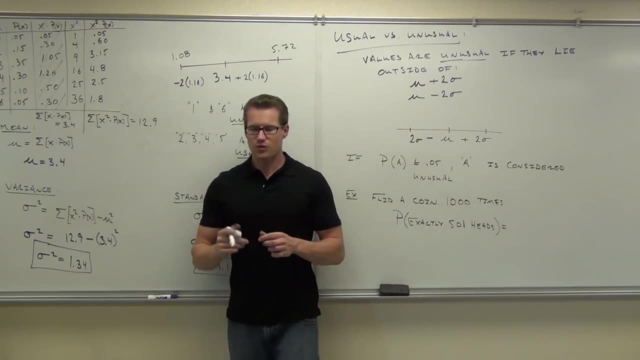 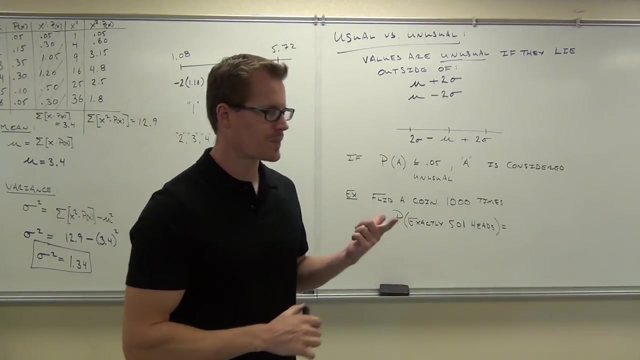 501 heads. Hey, let's think about that for a second. okay, So you're flipping this coin. There's only two outcomes, right? I hope there's only two outcomes. You can either get a head or you can get a tail. 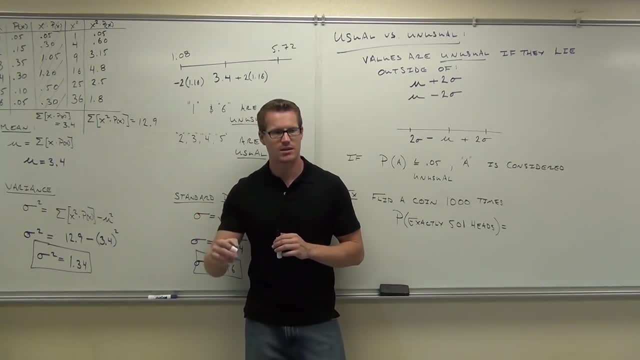 Now you're sitting there flipping this coin, You're counting up. okay, there's a head, there's a tail, There's a head, there's a head, there's a tail. Three tails in a row. whatever, Get some more heads. 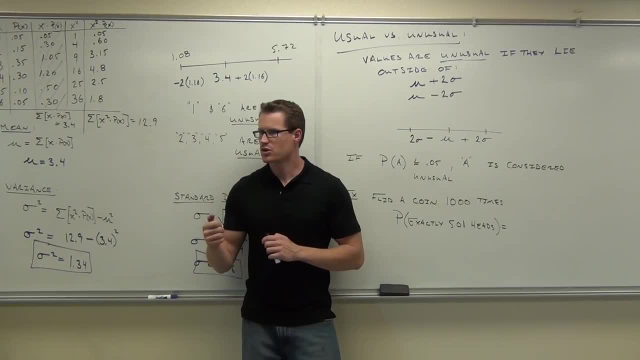 What's the probability that after a thousand flips of that coin, you're gonna get exactly 501 heads. Is that likely to happen? do you think Exactly, 501 heads? Could it happen Absolutely? Could you get 300 heads exactly? 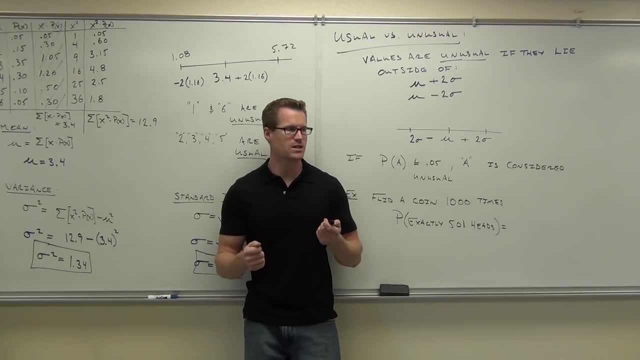 Could you get one head and 999 tails? Could that actually physically happen? Yes, it could. You could get a head and then for the rest of your flips you'd get 990,. would that? is that likely to happen? No. 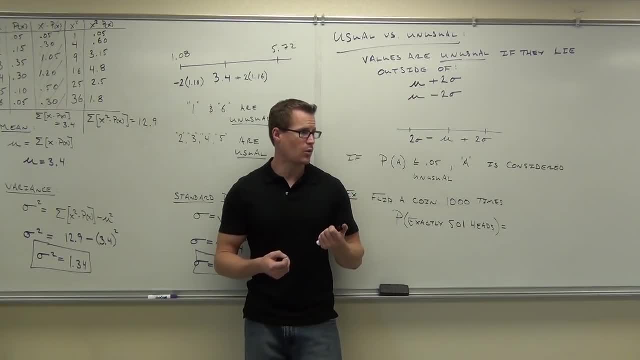 Is it likely to get exactly 501 heads? Probably more likely than getting only one head, but it's still pretty rare, right? Because you could get anywhere from like 450 to 550.. That would probably be reasonable, right? You know it's 50-50 to get a head. 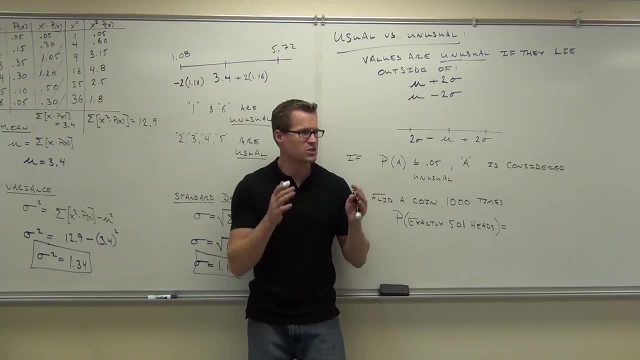 So typically you'd expect somewhere in that range, wouldn't you? Would you expect exactly 500 heads? I mean honestly, if you're flipping a coin and you flip it 10 times, are you expecting exactly five heads every time? 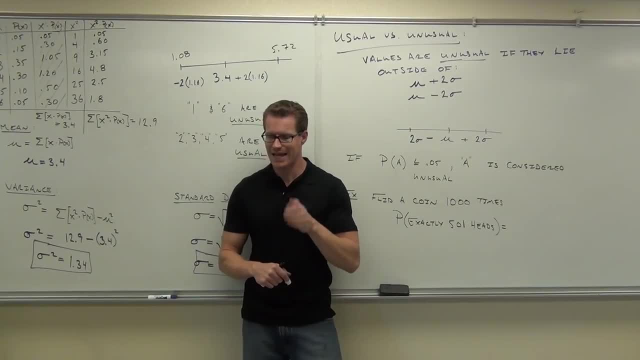 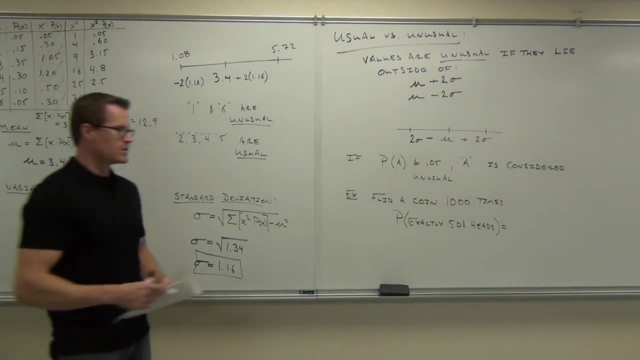 Probably not. If you flip it a thousand times, you're probably not expecting exactly 500 heads or exactly 501 heads. This probability's very rare. It's not gonna. it's not going to happen often, In fact, the probability of this- I did this earlier- 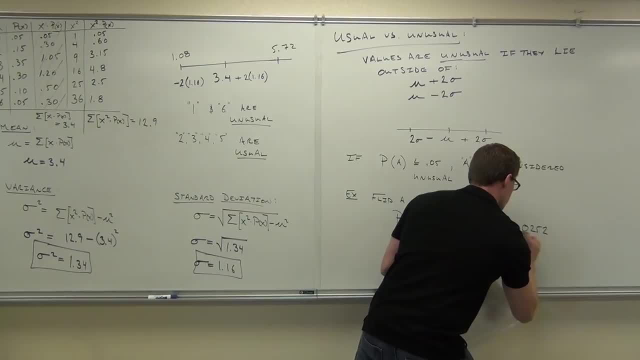 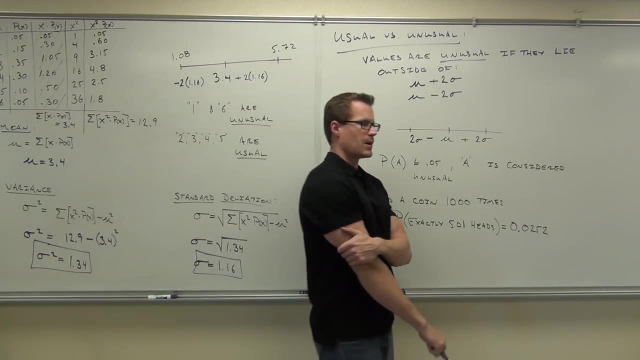 is .00252.. Or a little over 2%. That means that if you flip a coin a thousand times, there's a two and a half percent .00252,, .0252,. there's a 2.5% chance that you're gonna get exactly 501.. 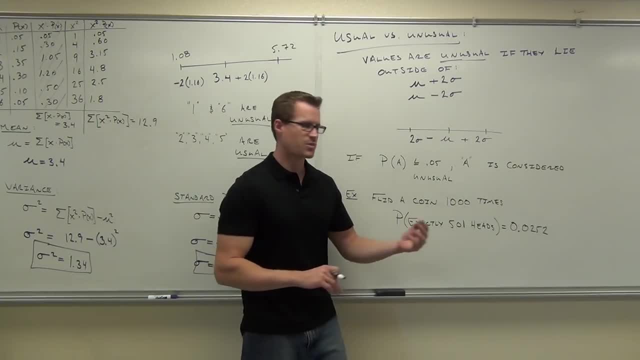 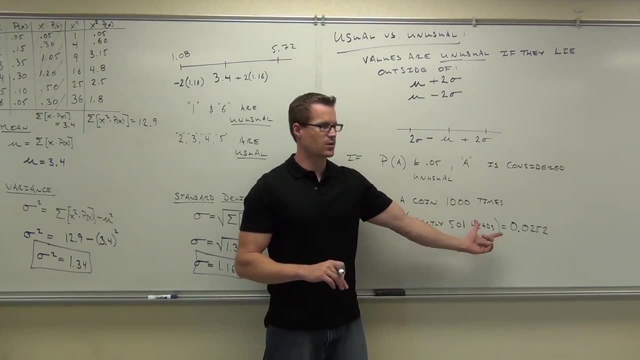 Is that usual or unusual? do you think? Is the probability of this happening usual or unusual? Unusual? Look at the probability. Is it less than or equal to? Is it less than or equal to .05? It's less than that. 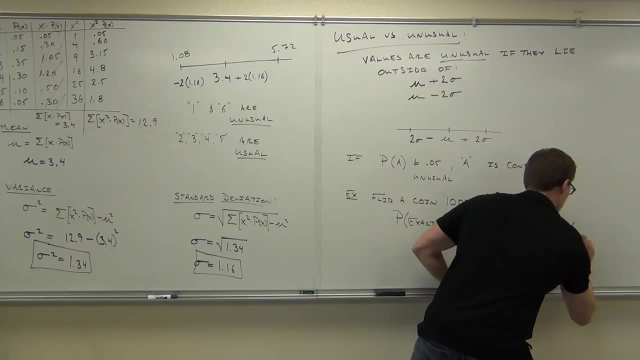 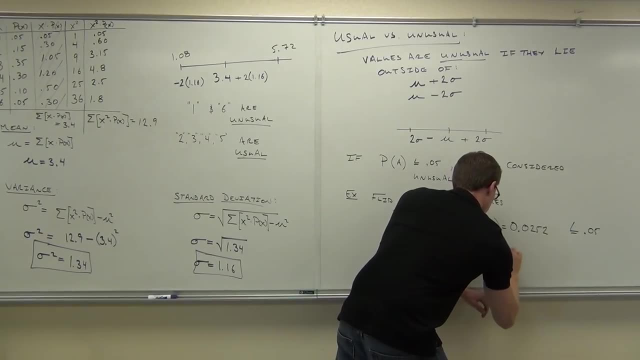 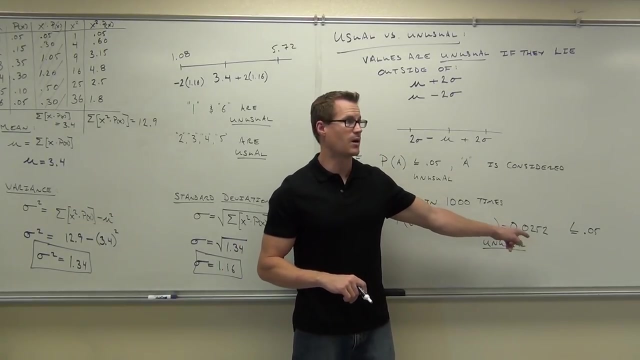 This is less than .05.. That makes this very unusual. So the way you look at this, you say: oh, you know what. I calculated the probability. Now you don't know how to do this yet I'm gonna tell you in about 10 minutes. 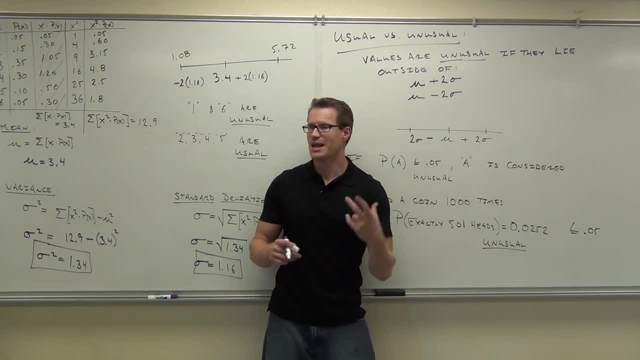 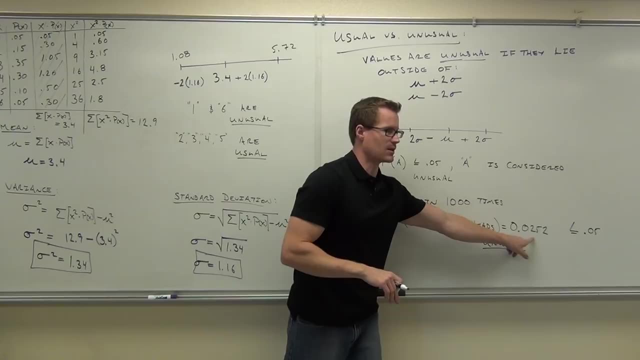 You don't know how to do this, but you look at the probability. If that probability is less than or equal to .05, you know you have something that's unusual. This was unusual. this was unusual. this one is definitely unusual. 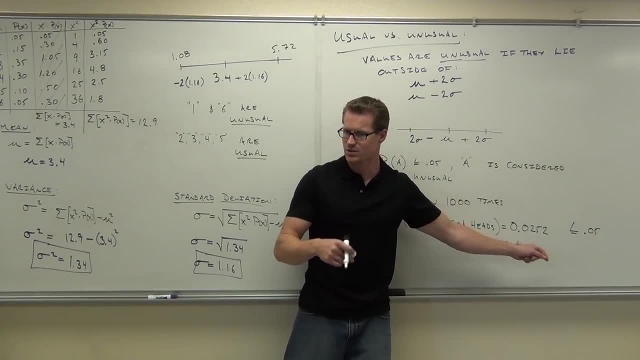 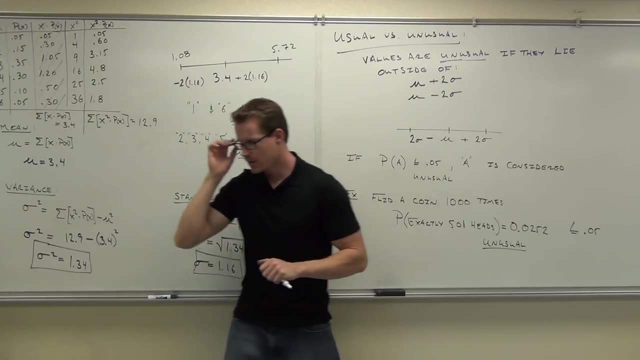 Even though there's lots of digits over here. look at the value of this number. it's .02, right, This is not bigger than .05,, it's less than .05.. How many people understood that? That's unusual, good. 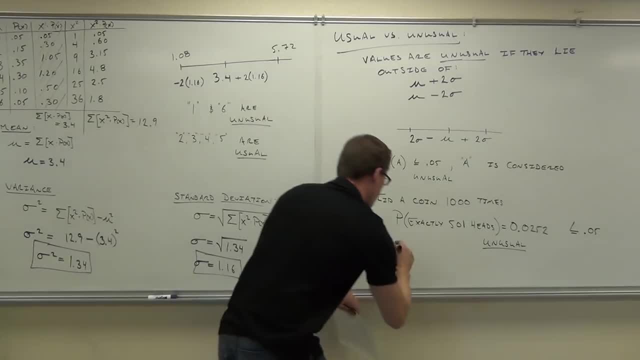 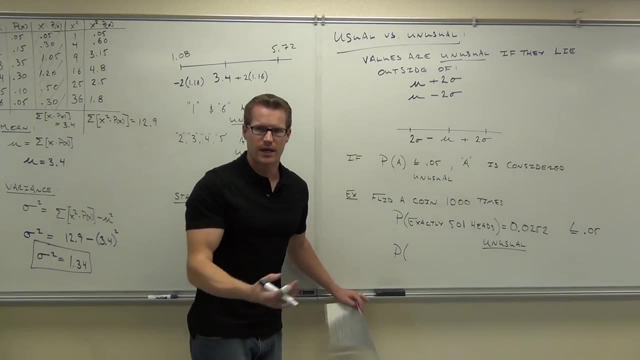 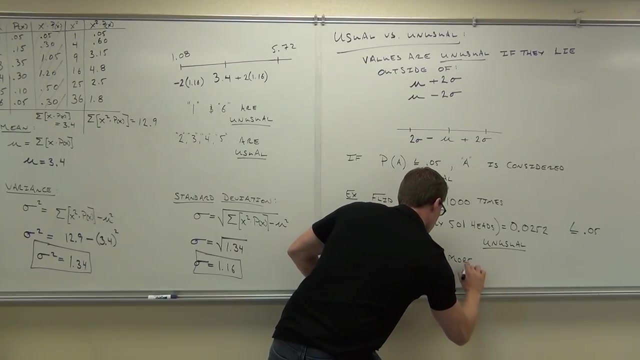 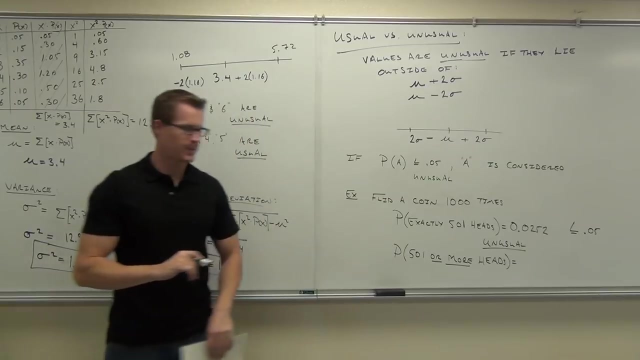 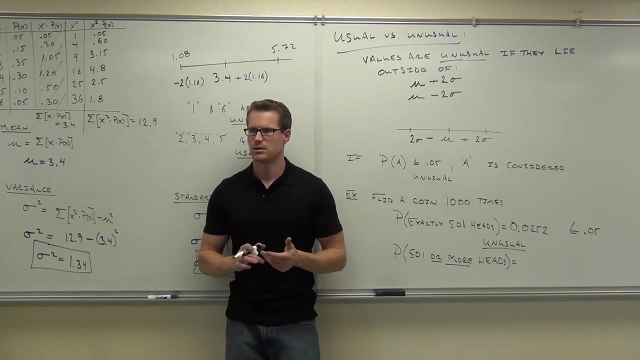 Now, what's the probability? think about this one. What's the probability of getting 501 or more heads, Okay, Hey. what does that? or more? what does that mean? What's or more mean, Okay, so if you have $10 or more, 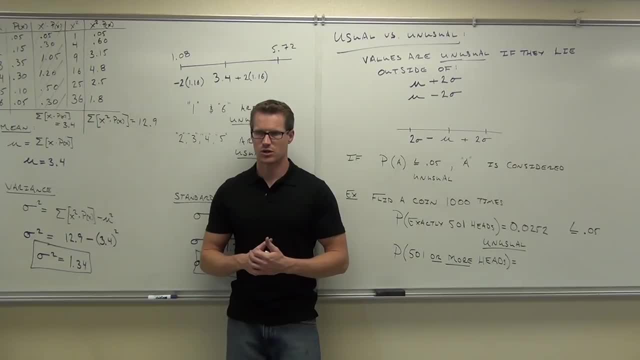 how much could it cost? Could it cost $10?? Could it cost $11?? Could it cost $9?? Not if it's $10 or more. If it's $10 or more, it could cost exactly $10 or anywhere above that. 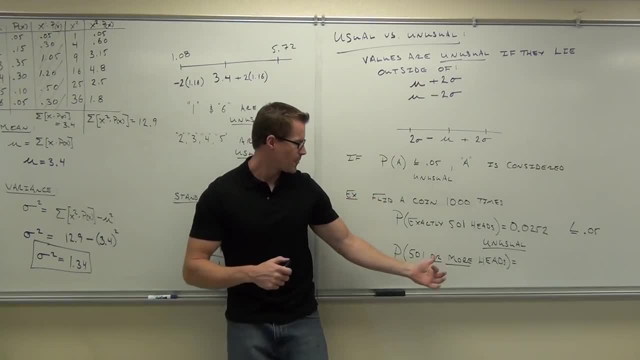 It could cost $1,000.. You with me. So when I say 500 or more heads, that's 500 and or 501, or sorry, did I say 500?? If I say 501 or more, it means it could be 501 or 502 or 503.. 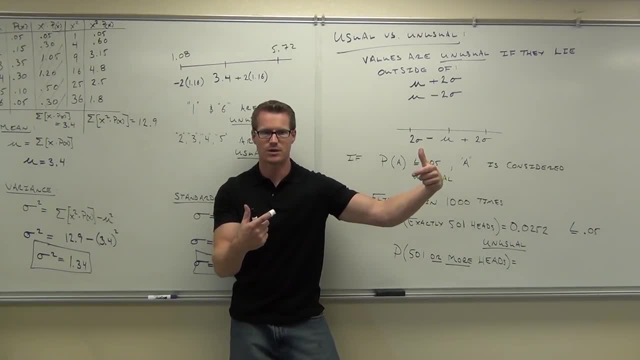 Or 504 or 505.. Do I need to keep going? It could include anything that is 501 or greater than that, up to 1,000.. Does this include the 1,000?? Would 1,000 heads count as 501 or more? 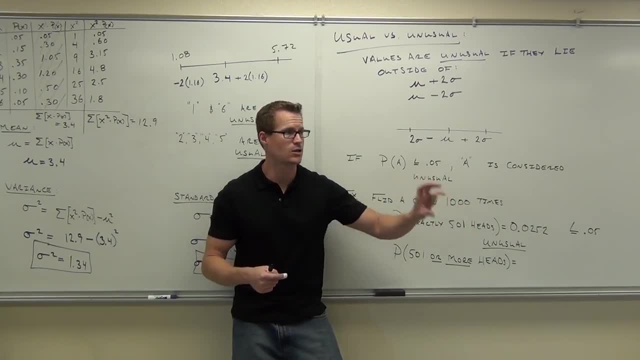 Absolutely Anything bigger than 501, and including 501.. Do you think that probability is bigger than this or less than that? What do you think? Is it likely you're going to get somewhere above 501? 501 heads Probably 50-50.. 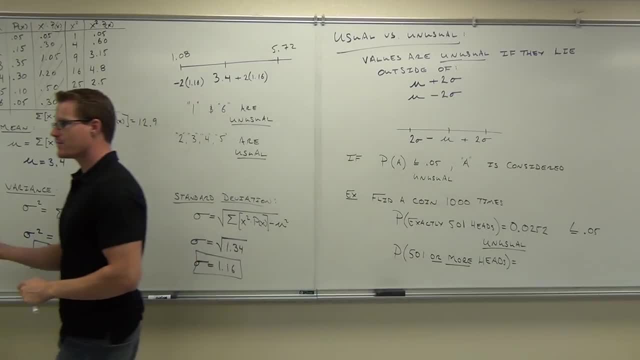 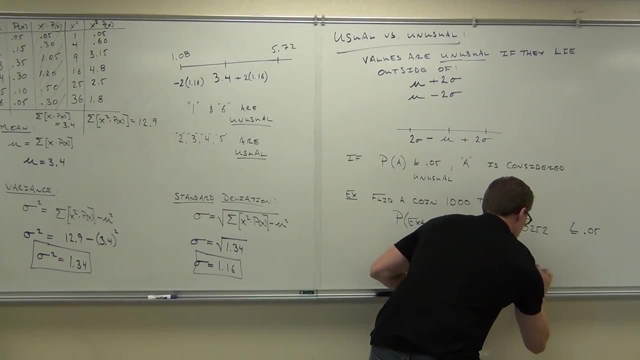 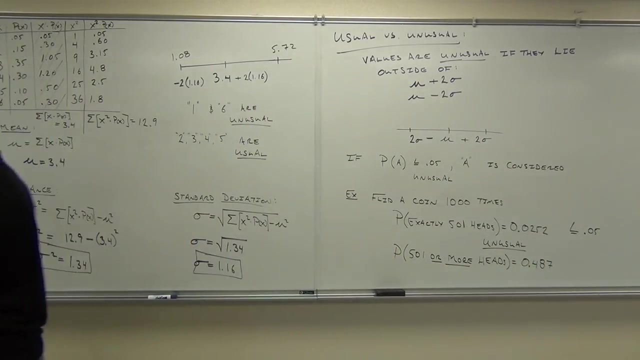 I mean or close to that, The probability of getting 501 or more, 502,, 503, 504 is actually 0.487.. The reason why it's so much bigger. I need you to understand this before I get to the next section. 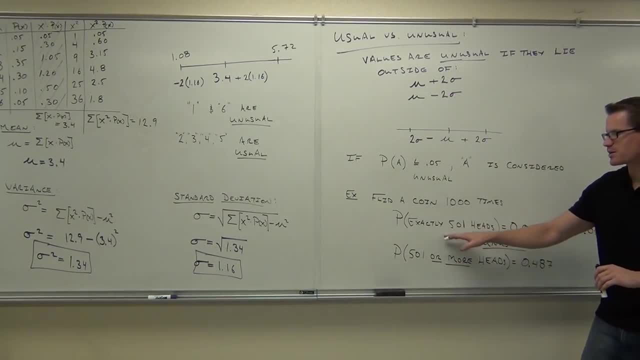 Just listen for a second, The reason why this one is so much bigger than this one. I need you to think about this one. This is the probability of landing exactly on 501 heads. That's pretty rare. This one do. you have a lot more options here. 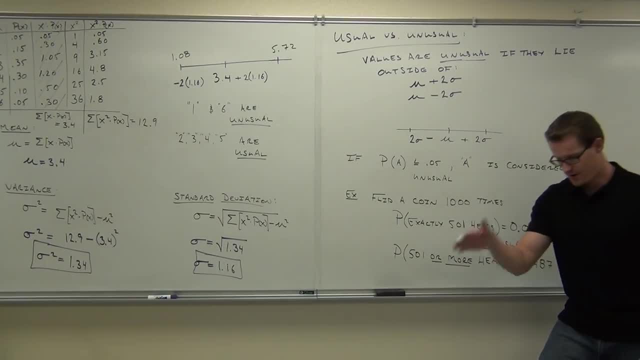 This is one option. This is: 501 will work, 502 would work, 503 would work, 504 would work And every option up to 1,000 would actually work. This is hopefully you remember this. this is an or probability. 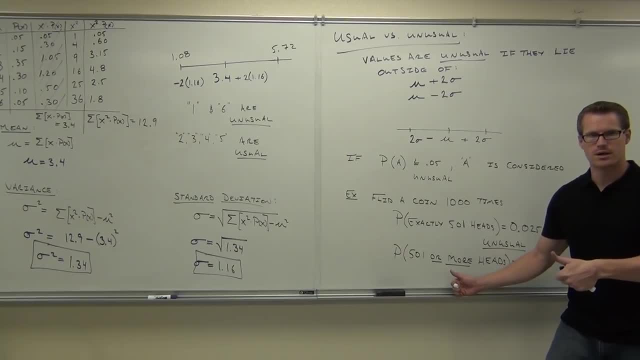 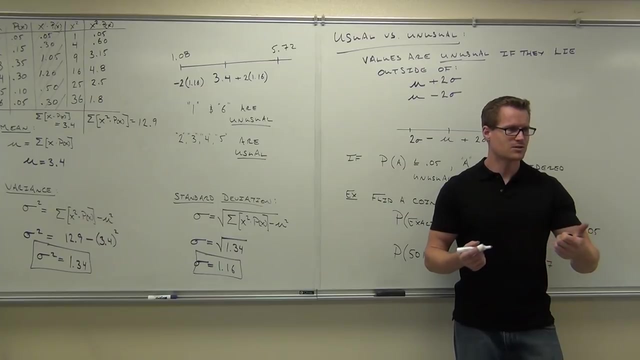 This is 501 or 502 or 503.. What do you do with those probabilities? Remember, when you have an or probability, You better remember this for your test. You have an or probability. Do you add that or multiply that? Give me notes or something. 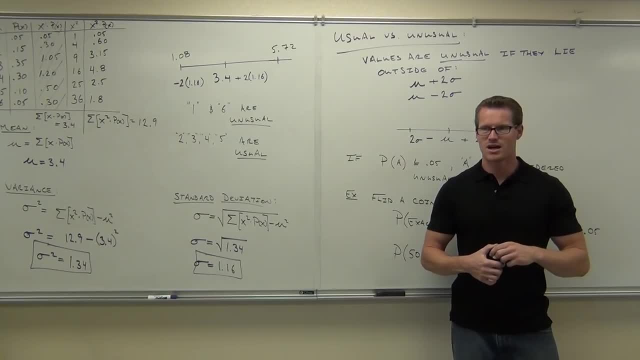 Figure it out. Your time is running out. You have an or probability An or probability Something or something. Do you add it or do you multiply it? That's why it's called the what rule, That is, the addition rule. 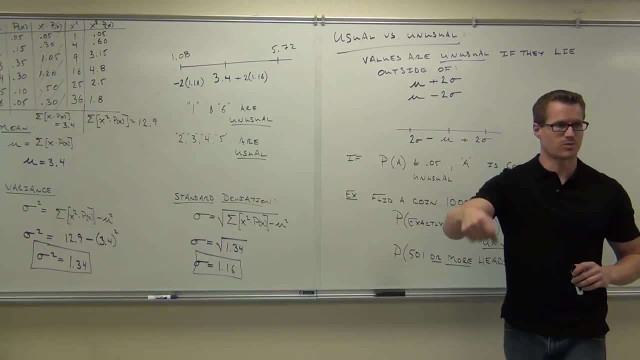 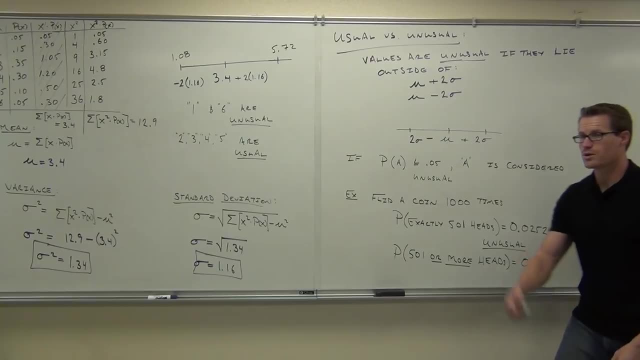 The addition rule is used for, or. So here's what this means. ladies and gentlemen, You better refresh your memory on that. if you don't know that, okay, Go back and watch those videos. If you have a 500 or more, you have 501 or 502 or 503,. 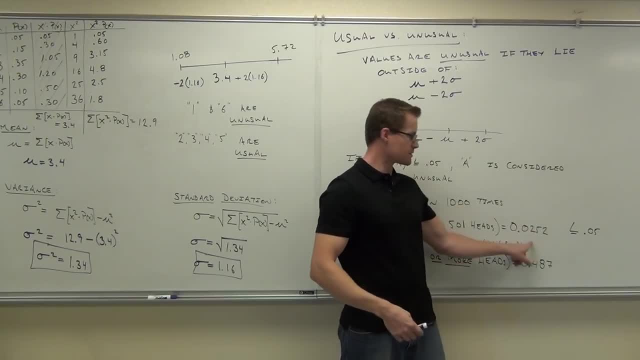 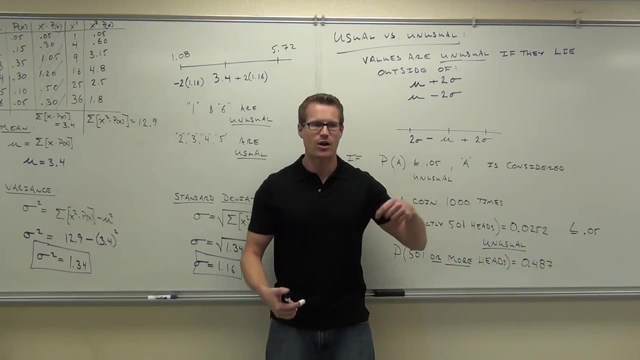 you're adding every one of those probabilities. It's like this: They're all small, but you're adding them up, and you're adding 498 of them, 499 of them together. Okay, so if you add all those probabilities up,